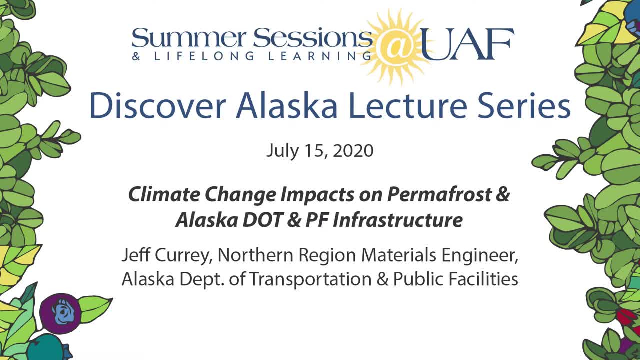 of Transportation and Public Facilities, Jeff Curry, has been working in, on and underneath permafrost for nearly 30 years. He has been the Northern Region's Material Engineer for Alaska Department of Transportation and Public Facilities since 2011,, supervising the region's drilling. 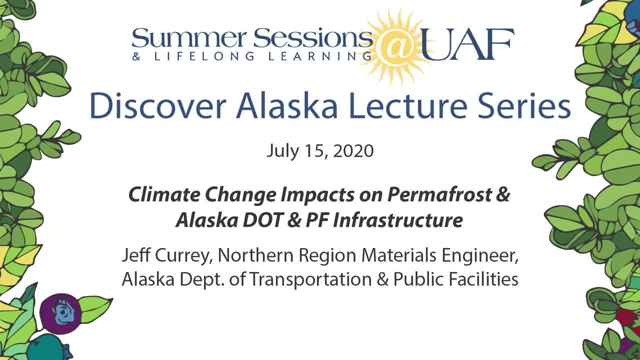 engineering, geology and geotechnical engineering programs. He started his DOT career in 2000,. including Highway Designer and Materials Engineer. He was Northern Region Geotechnical Engineer for six years prior to that. Jeff has also worked in the mining and mineral exploration industry in interior Alaska throughout. 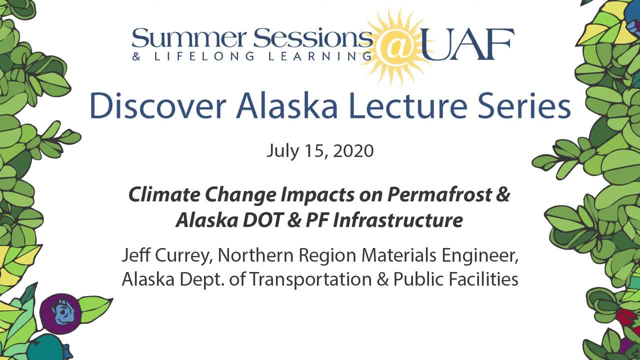 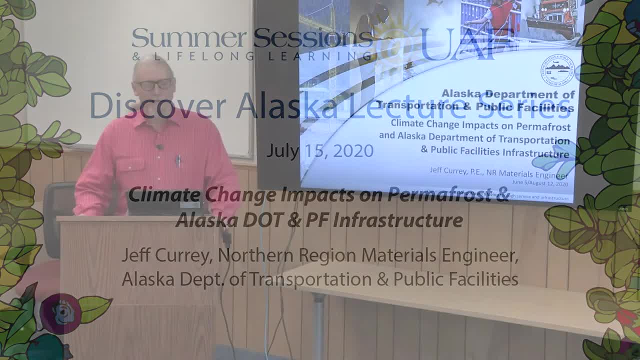 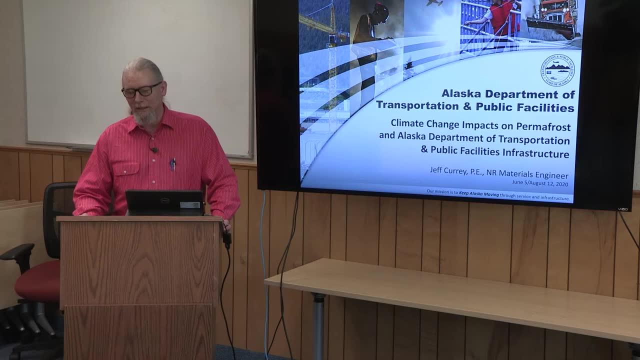 the 1990s. We thank you, Jeff. We appreciate you sharing your expertise on climate change on the transportation infrastructure for Discover Alaska. Good afternoon everyone, Good evening. actually, I understand you'll be watching this on August 12th in the evening. 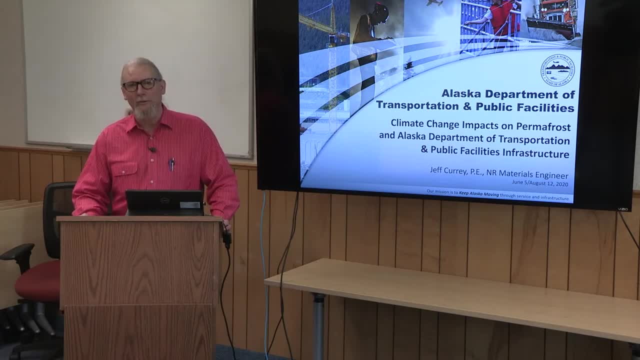 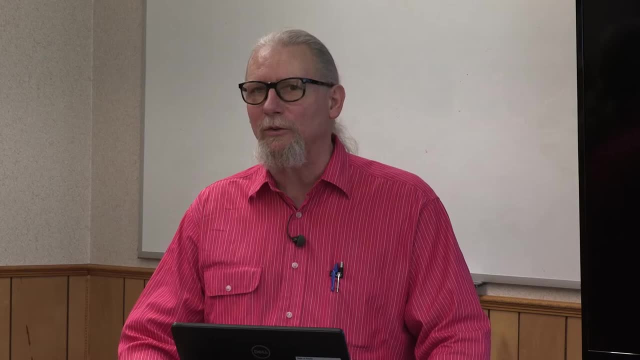 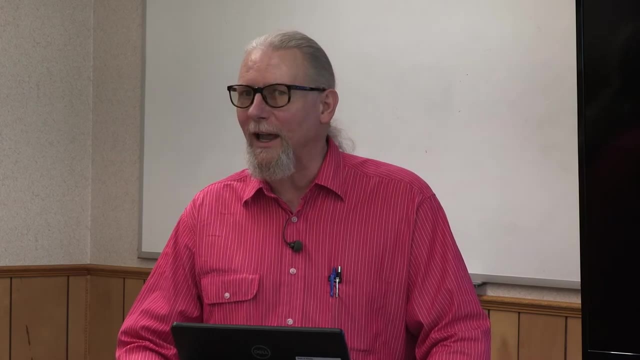 but we're recording this on June 5th in the afternoon, So a couple caveats that come with that. First of all, anything weird that happens between June 5th and August 12th that makes anything I say sound silly or stupid is not my fault and I got no control over that. 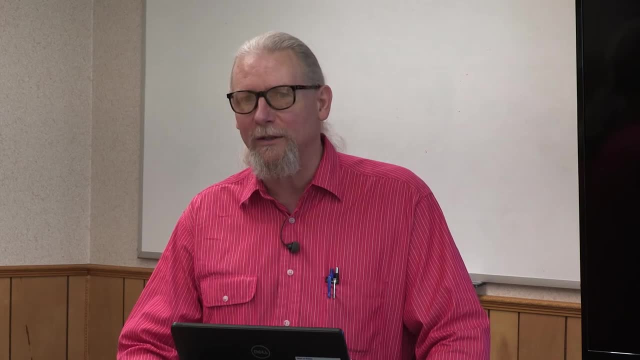 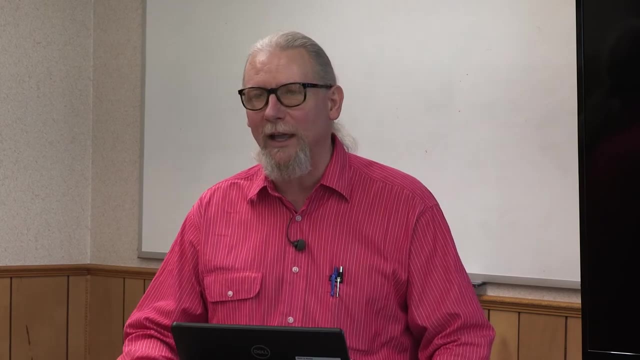 My crystal ball is pretty dusty. The other thing is that I normally give a presentation just to folks live and I enjoy having some interaction and asking some questions. So this is a little bit weird for me, but that's okay, We'll get through it here. 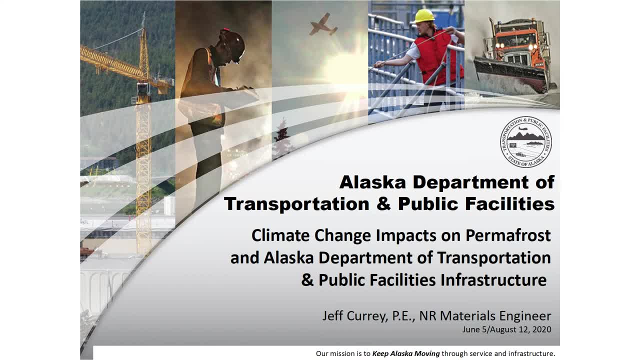 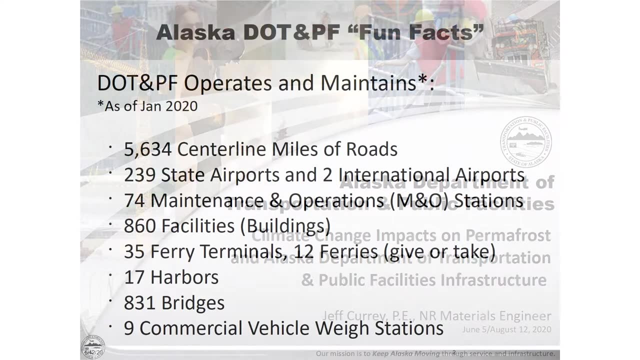 I work for the Department of Transportation and Public Facilities, DOT and PF, and so I get to talk. get my little obligatory spiel about DOT first. Our mission is to keep Alaska moving through service and infrastructure. A few fun facts about Alaska- DOT. We operate and maintain roads. We've got about 5,600 miles of roads, which may sound like a lot, but for a state the size of Alaska it's really not, and most of our roads don't have very much redundancy. A lot of them are the only road to get where you want to get, Unlike most DOTs. 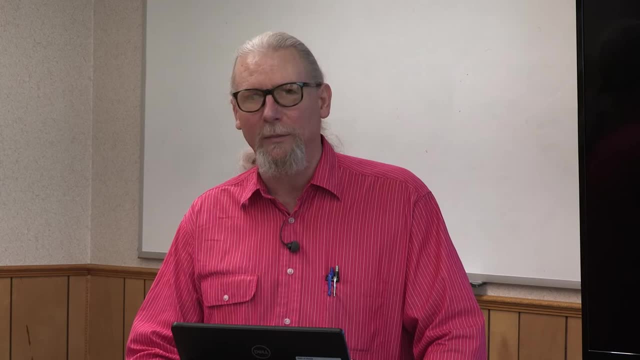 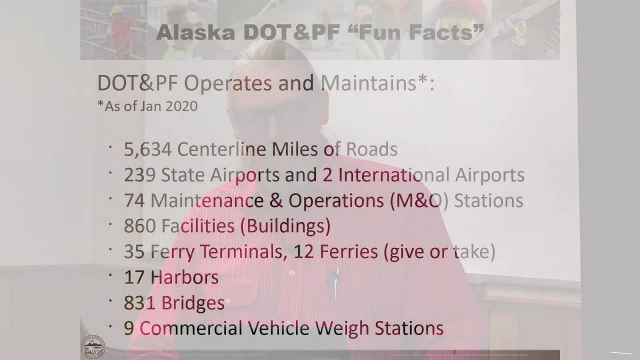 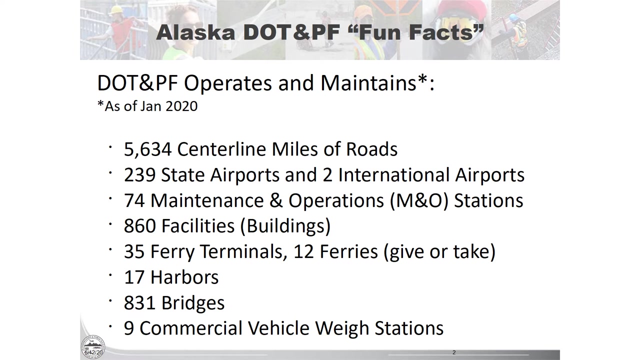 we have a lot of airports, We do airports and we have something like 142 communities in the state that rely on airports exclusively for their access. You'll hear me use the term M&O a lot, and we're also used to using the term M&O a lot- And we've got maintenance and operations folks. 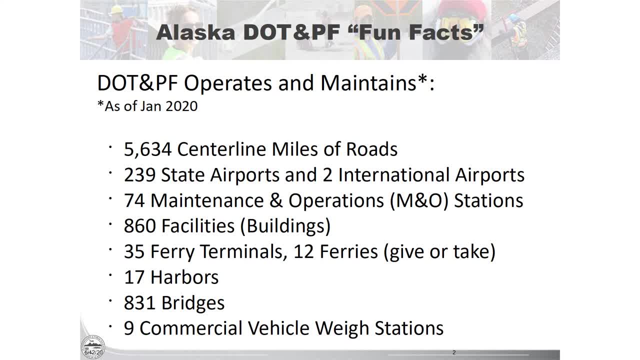 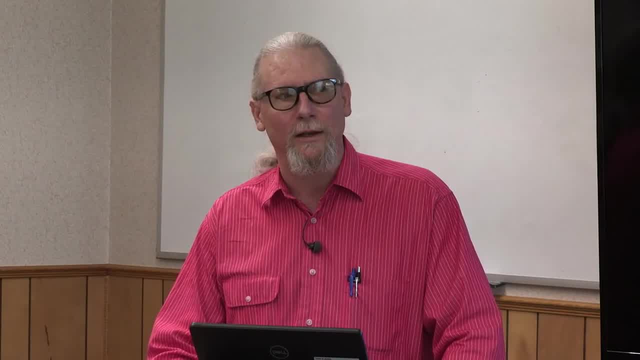 These are the guys and gals who are out plowing snow, fixing potholes, clearing brush and whatnot and, among other things, fixing damage due to thawing permafrost. We've got maintenance stations on our road system and, because these roads are so far-flung, a lot of these. these: 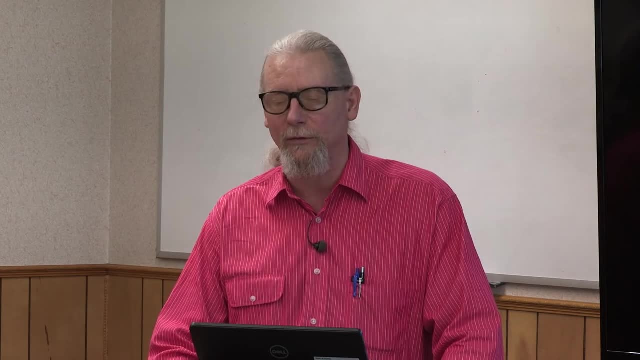 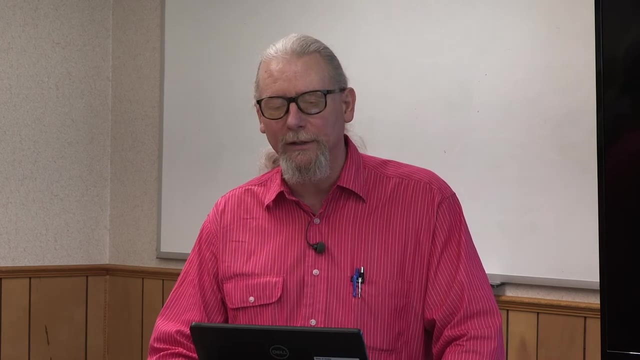 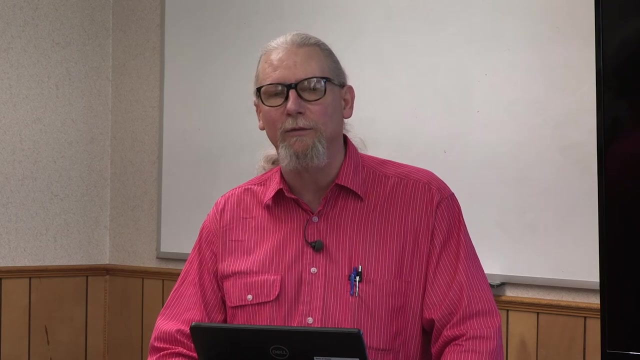 stations are actually camps where the operators live and stay for shifts, doing shift work. and PF does not stand for permafrost, It's public facilities, which is to say buildings. We have something like 780 buildings that are actually DOT facilities. These are these. 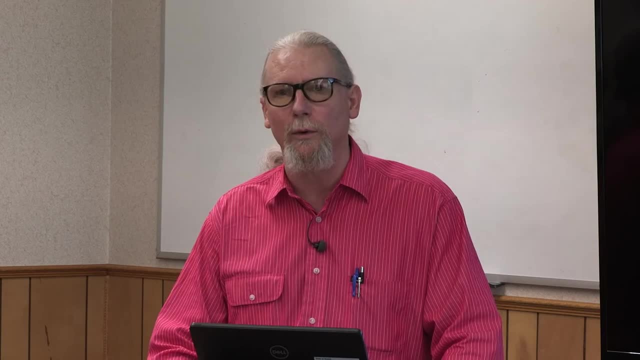 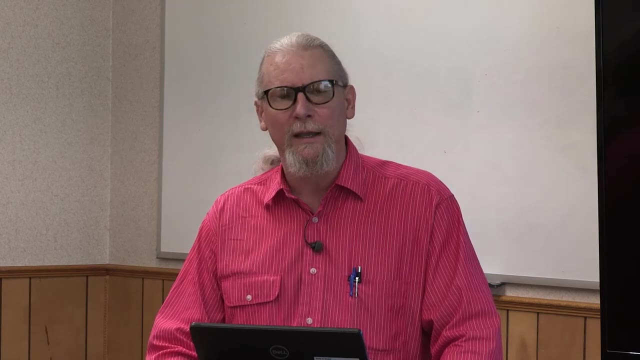 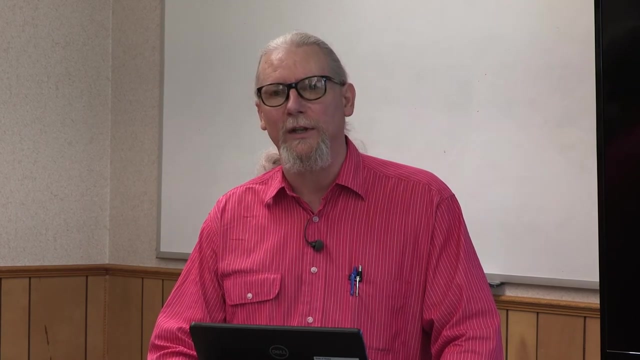 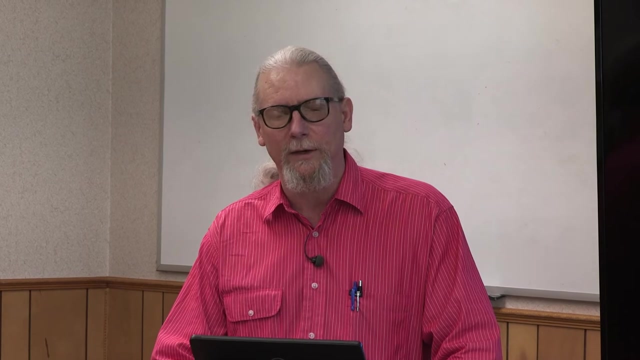 maintenance and operation stations, the offices that we're recording this in right now, snow removal equipment, buildings at these airports. But a few years back the state decided to make DOT and PF responsible for maintaining other state buildings as well for our sister agencies. So something like 80 of those buildings that we're maintaining now are other agencies. and the plan is to have about 1,800 under our operation and management by the end of 2021.. Also, unlike most DOTs, we operate a ferry system. We have 35 terminals and 12 ferries give or take. 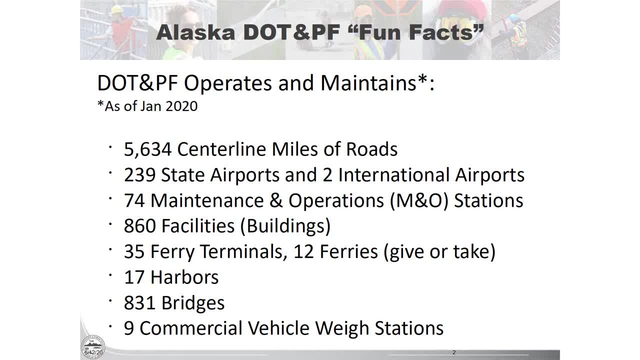 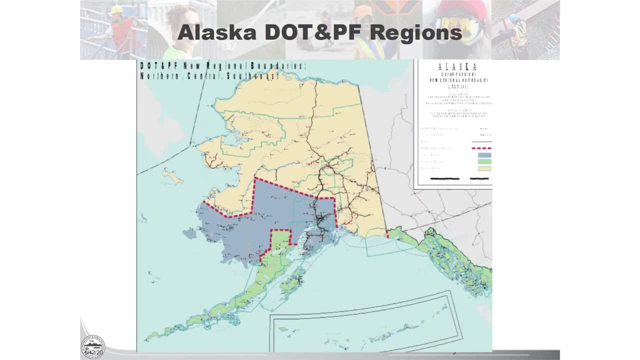 Not necessarily, Not necessarily all operating at any given time. We have harbors and, of course, with the roads, we've got bridges and we've got commercial way stations. DOT is organizationally broken into three regions. The green area is our south coast region. It used to just. 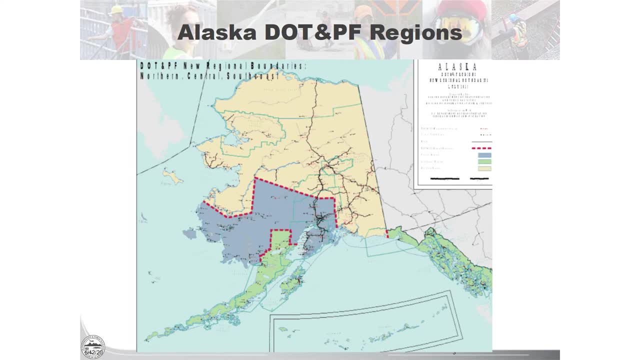 be southeast. but now a few years back they moved the Kodiak, the Aleutians and a little bit of the YK Delta And to combine it with southeast to make our south coast region kind of makes sense. It all has sort of the same character Climatologically. they're all similar. 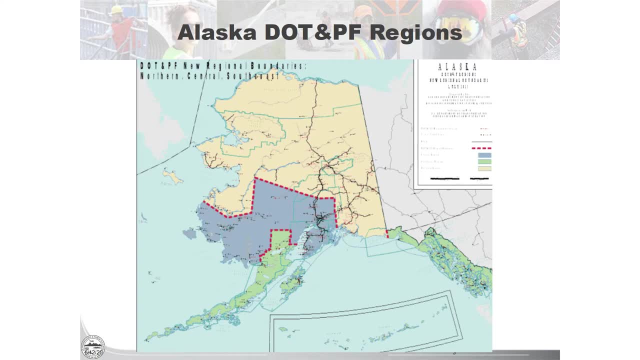 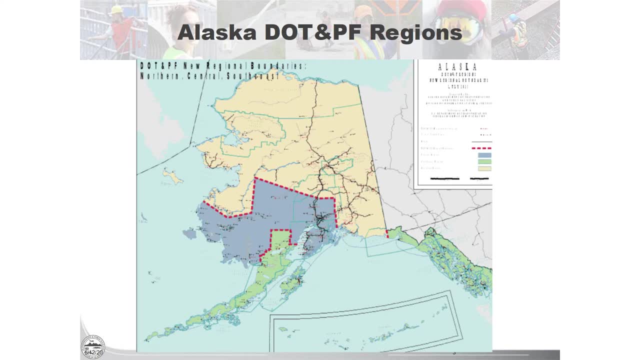 of the roads, most of the national highway system, most of the interstate highway system. Yeah, we do have interstate highway system, believe it or not, It's a classification- even though we don't connect to any other state And we have more than half of the airports. 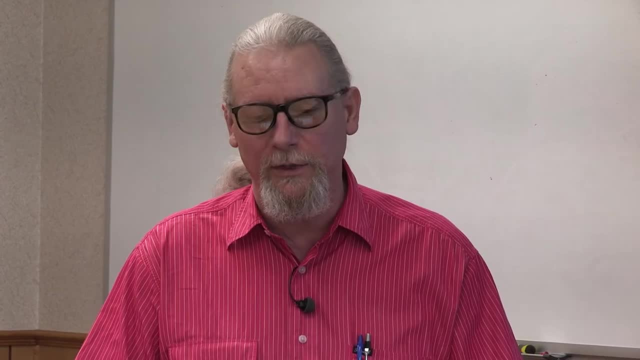 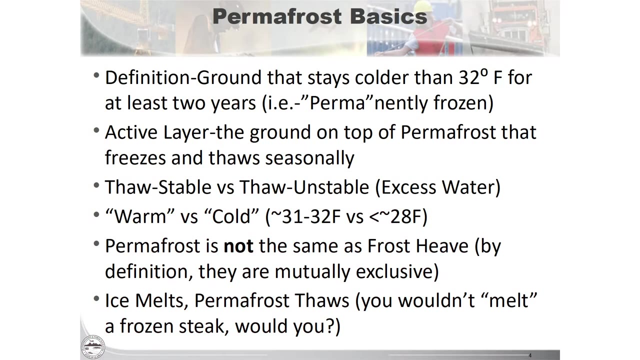 Just so we're all on the same page when we start this, let's do some definitions for permafrost. Permafrost is defined by a thermal condition. We define permafrost as ground that stays colder than 32 degrees continuously for at least two years. Now, two years is sort of arbitrary. 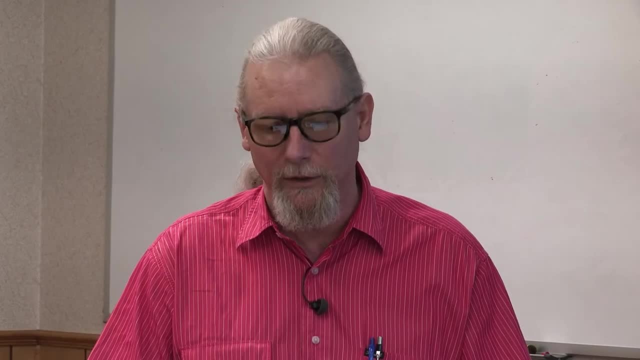 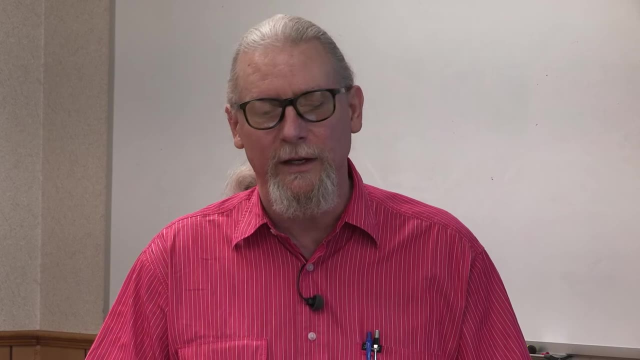 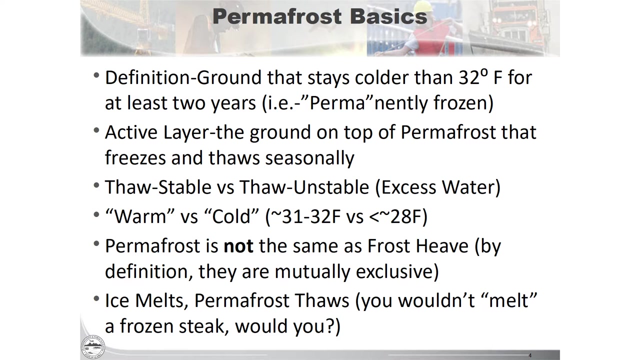 Most permafrost has been frozen for thousands of years, But the point is is that it doesn't ever get above 32 degrees. If it does, then it's not permafrost. Now, the active layer is the ground that's above permafrost, And that's the area that thaws in the summertime, when the air is warmer than. 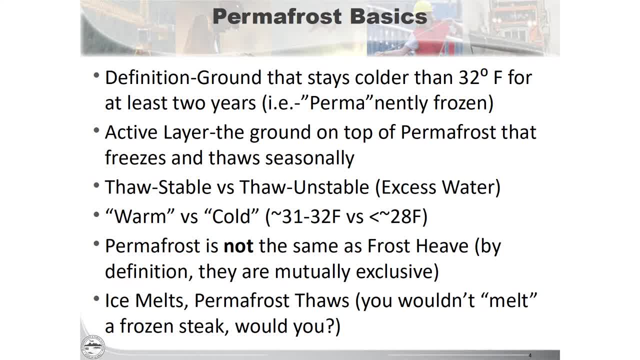 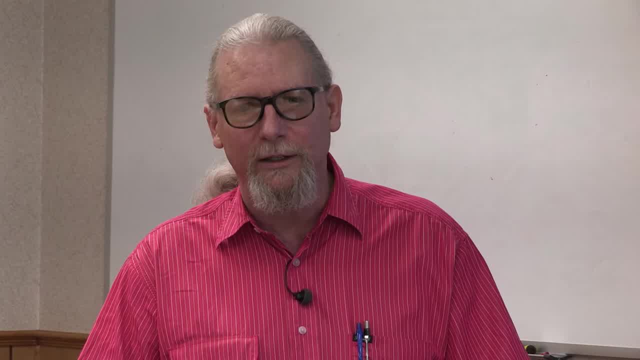 freezing and thaws or freezes back in the wintertime. We frequently classify permafrost as whether it's thaw stable or thaw unstable. We frequently classify permafrost as whether it's thaw stable or thaw unstable. The fact that it's 31 degrees makes a big difference for some things, not for others. 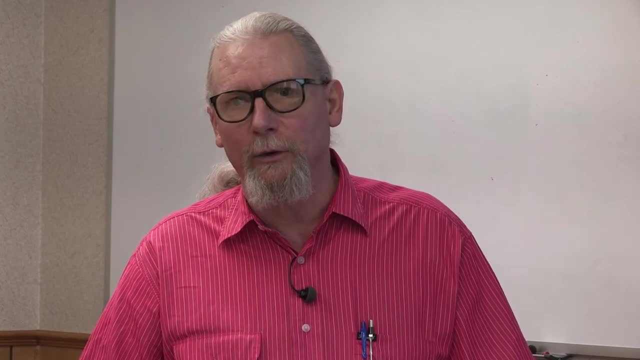 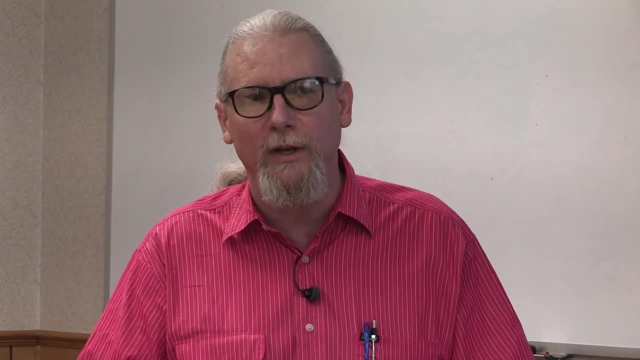 Take, you know, solid bedrock, for example. You build a road on solid bedrock. it's 31 degrees, It warms up to 33 degrees, Nobody cares. River gravel tends to be pretty stable whether it's frozen or thawed. It's really stable when it's frozen. When it thaws, not much happens and it's. 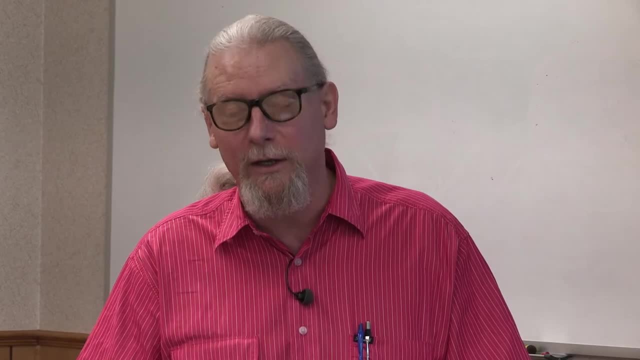 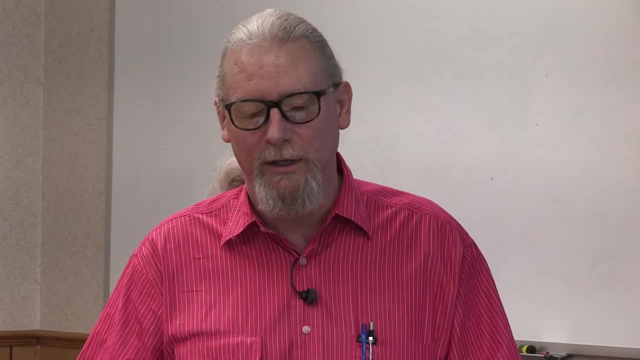 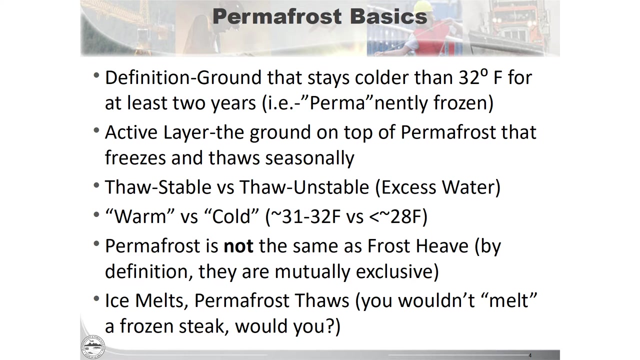 still a pretty good foundation for roads. Silt, on the other hand, in particular ice-rich silt with excess water, is what we call thaw unstable, And that's the problem actor. We'll be talking about that a lot more. We frequently distinguish between warm permafrost and cold permafrost, Warm being really close to. 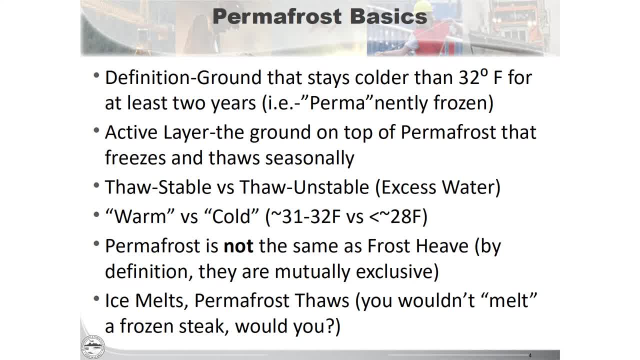 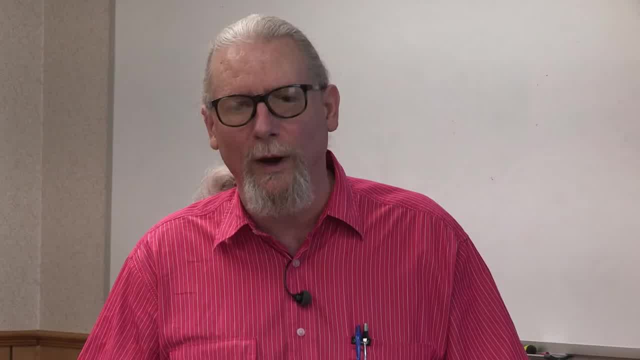 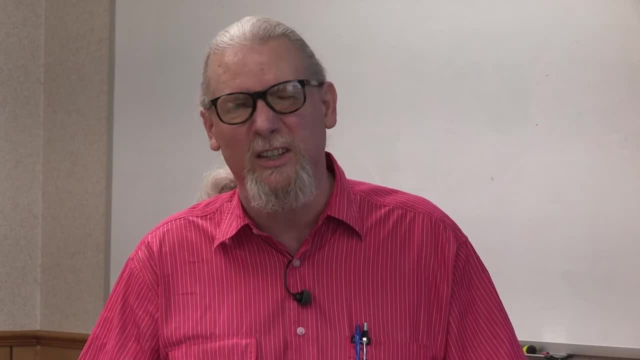 freezing and that's the kind of permafrost we have around Fairbanks. It's, you know, within a degree or so of freezing, and the takeaway there is: if the ground warms up a degree or two, boom, you've got thawing permafrost, Whereas on the north slope, for example, permafrost might be, say, 25 degrees. 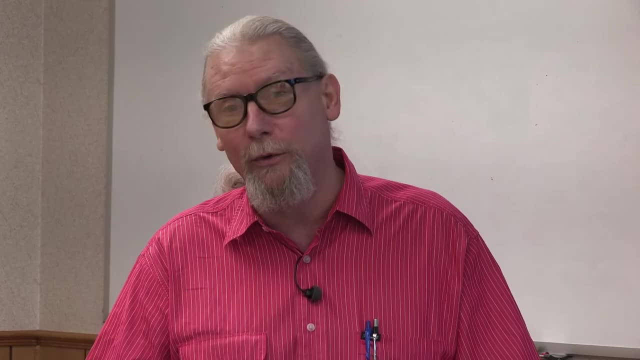 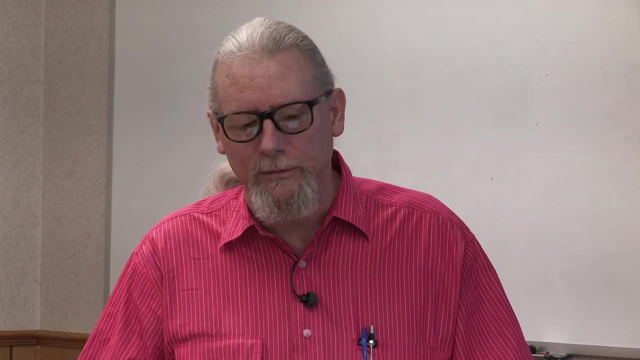 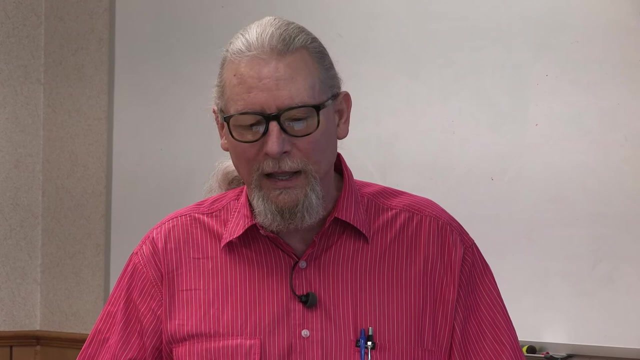 and if it warms up a couple degrees, okay, it's still pretty cold and it's still pretty frozen. A couple things that irk some folks, including me. permafrost is not the same thing as frost heave. There's a lot of people who should know better but confuse these terms. Permafrost is 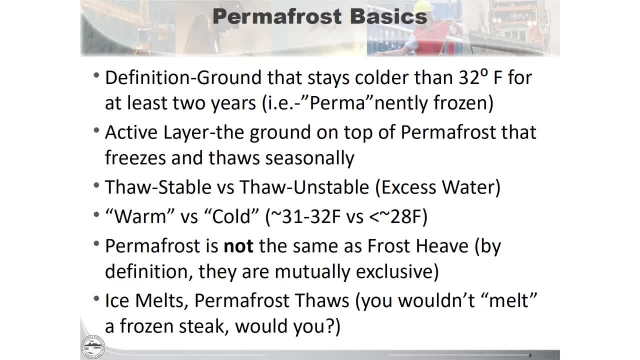 continuously frozen right Frost heave is, by definition, ground that freezes and, for a number of reasons, heaves in the wintertime and then settles back to freezing. That's the kind of permafrost that freezes and then settles back down in the springtime when it thaws. Well, if it. 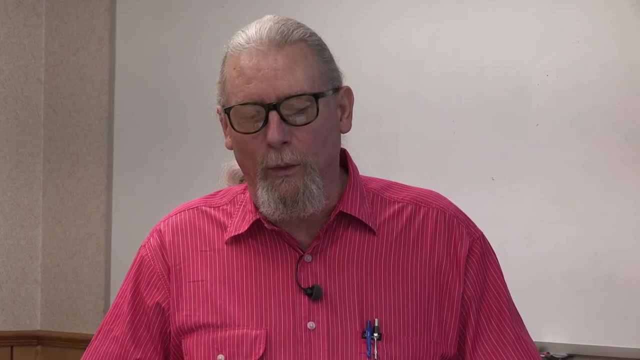 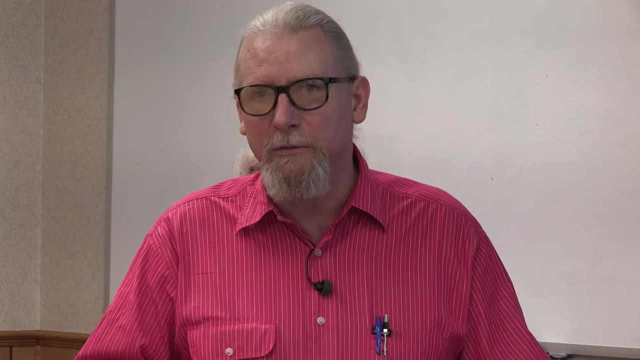 thaws, it's not permafrost, right. And then, finally, we melt ice, we thaw permafrost. If you pull a chicken out of the freezer and put it on the counter, you're not melting out your chicken. 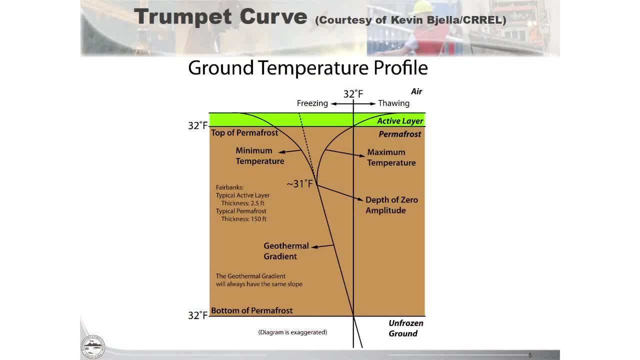 right, You're thawing it out. This diagram, this trumpet curve, shows the temperature of the ground, the maximum and minimum temperatures in the ground and at the highest and lowest part of the year At the surface, at the ground surface. 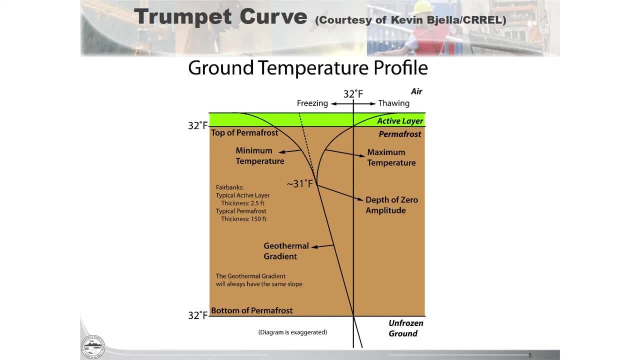 the air temperature goes from what in Fairbanks, maybe 40 below these days, maybe, maybe not, up to 80 degrees or 90 degrees in the summertime. Well, the surface of the ground pretty closely tracks the air temperature, And so on the warmest or around the warmest day of the year, the surface of the ground is going to be pretty close to the air temperature, But as you go deeper it doesn't get as warm. There's the specific heat of the ground, there's the insulating factor, and this may not happen at the same, in fact. 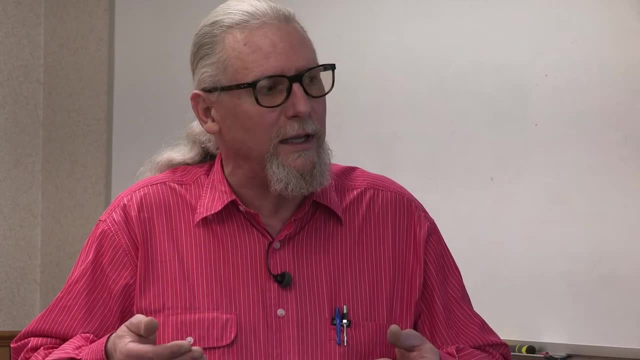 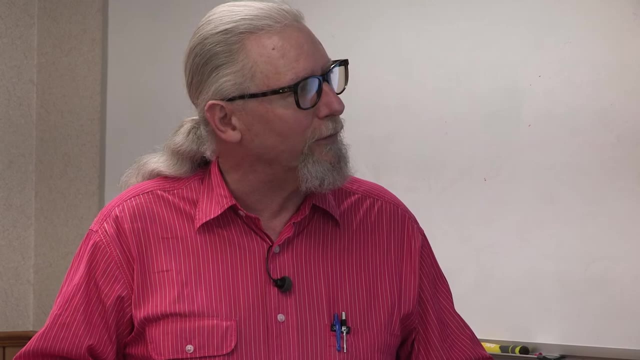 it doesn't happen at the same time, because it takes time for that heat from the summer to work its way down into the ground. That point where the curve reaches the 32 degree Fahrenheit is probably in October, Prr. 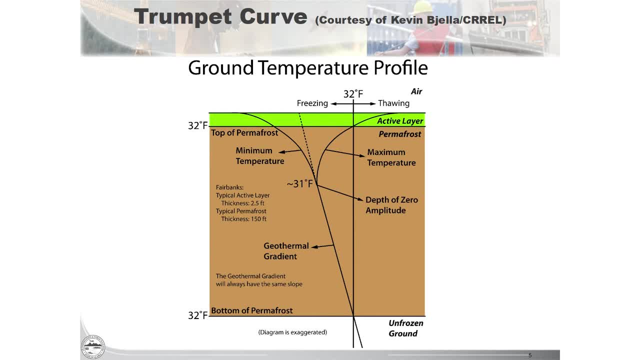 likely after things are starting to freeze a little bit just because of that delay. But the takeaway here is: as you go deeper in the ground, the hottest temperature, warmest temperature the ground ever gets is less and less as you go deeper until 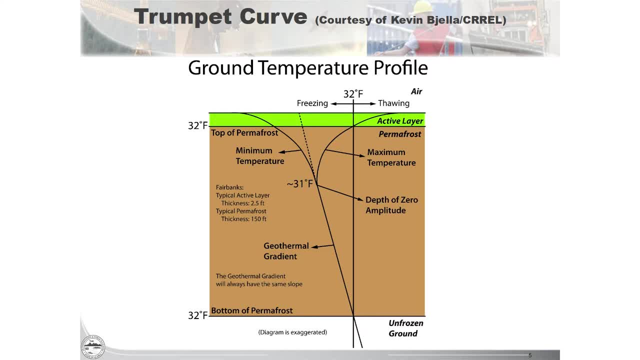 hey, once you get below that 32 degrees temperature, if it's 32 on the warmest day of the year, on the warmest day it ever gets, then it's more than 32 below the rest of the year, And so 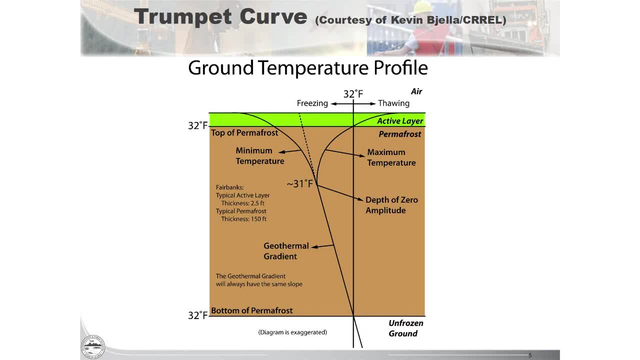 boom, now it's permafrost. Similarly, on the cold end the ground surface gets much colder than the typical surface at depth because it's exposed to the air temperature in the middle of the wintertime, And the deeper you go, the less cold the coldest day of the year is. 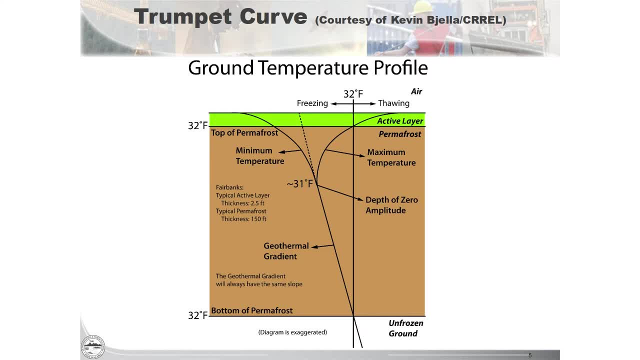 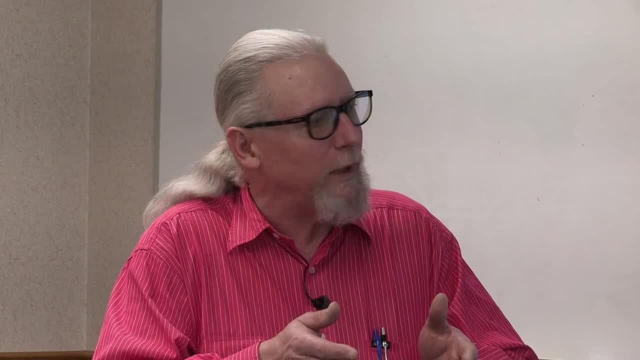 at that depth. As we descend deeper into the ground, those extremes get closer and closer and it's much colder. And then as we descend deeper into the ground, those extremes get closer and closer and it's some point we get a point where there's basically the warmest day and the coldest day. There's no. 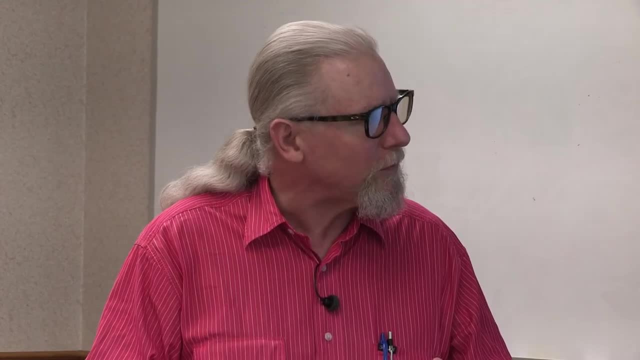 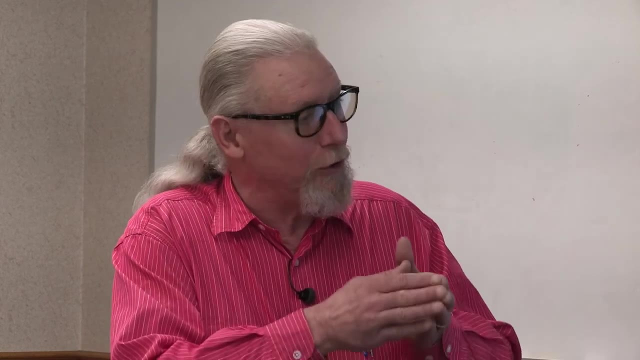 change year over year, throughout the year. I call that the depth of zero amplitude, which doesn't really mean anything except that at that point, that's what the temperature is. And then, as you go deeper, you start heading towards the center of the earth, where you got molten iron and nickel. 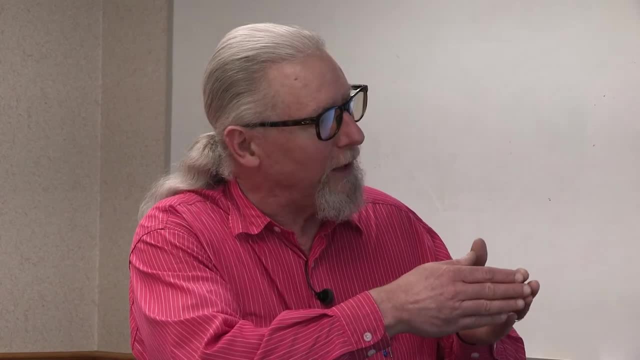 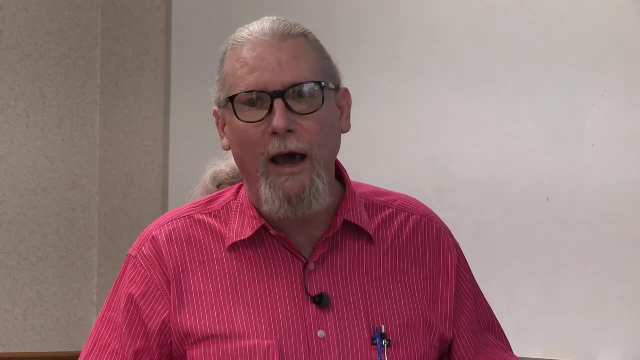 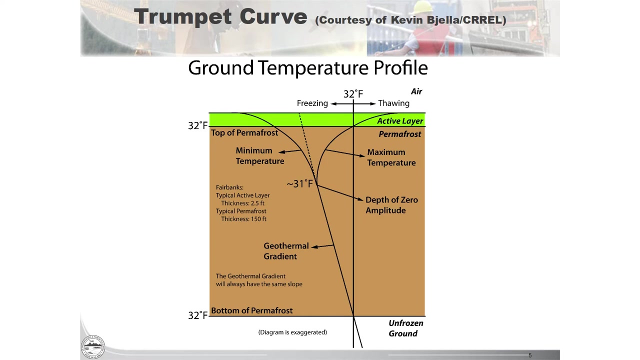 and stuff right, And so it's hotter, And so the ground has this geothermal gradient. So the deeper you go, the warmer it gets, until again you cross that 32 degree line And now you're out of permafrost and into thawed ground at depth. Now one of the interesting things here is, if the summer 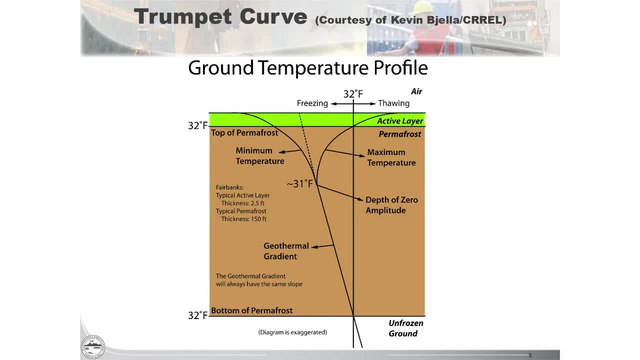 air temperature gets a little warmer at the peak of the summer, and if summers are a little longer, you can imagine that that upper right-hand curve is going to kind of shift to the right a little bit, which is to say warmer, And if the winter temperatures are not as cold as they used to be. 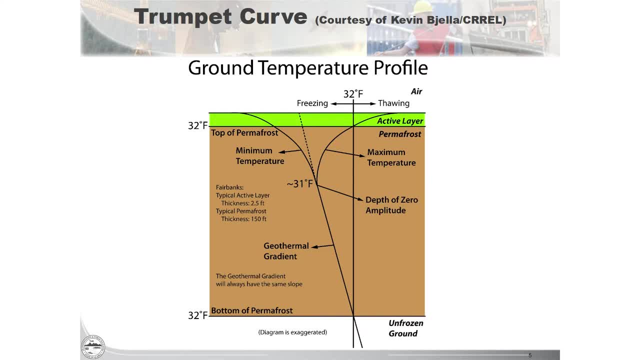 a little warmer and the winter is a little bit shorter, the left side of that curve is going to shift to the right a little bit, And so that whole curve is going to shift further to the right And so, but everything else is going to is staying the same there. So you can imagine that the 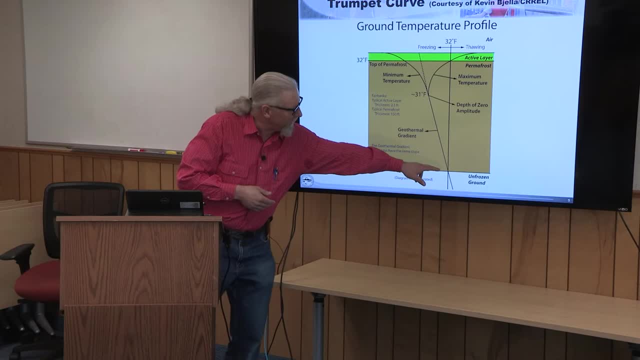 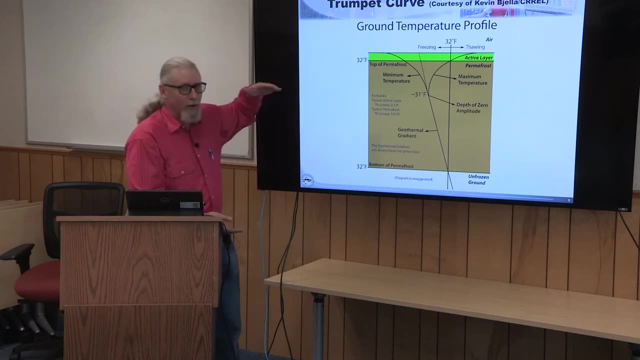 geothermal gradient. instead of running out of permafrost here, maybe it's going to start working its way up and thaw from the bottom up, And similarly the active layer is going to get deeper. So permafrost is degrading from the surface and from the bottom. 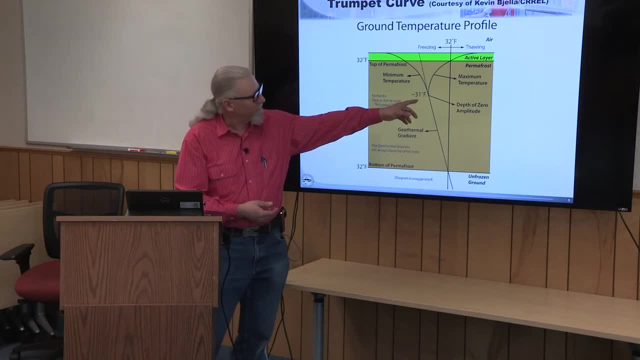 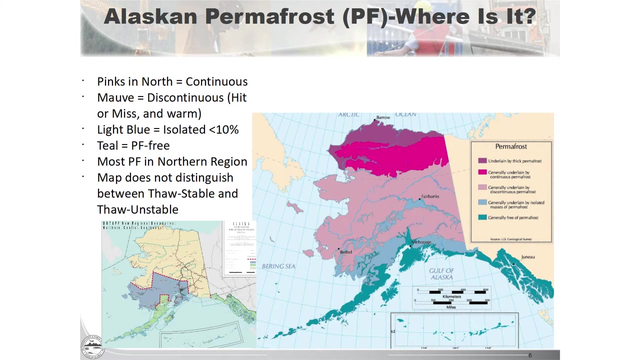 And this temperature, this depth of zero amplitude temperature, is going to work its way further and further And this whole area that's under the permafrost curve is going to become less. So here is a map of permafrost. That's not really right. It's really not a map. 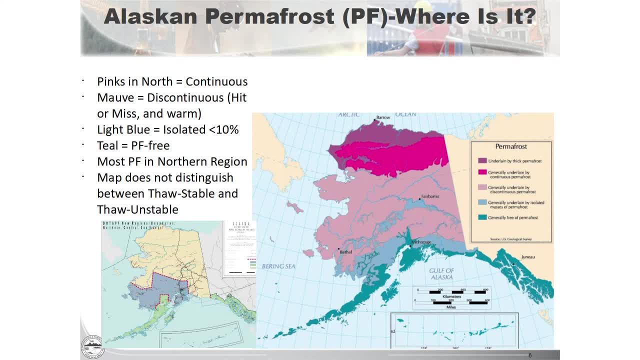 of permafrost. It's a map of permafrost probability or permafrost zones. The pink and rose color at the top that's continuous permafrost And the and the takeaway there is that's mostly North Slope. The takeaway there is: you go anywhere. 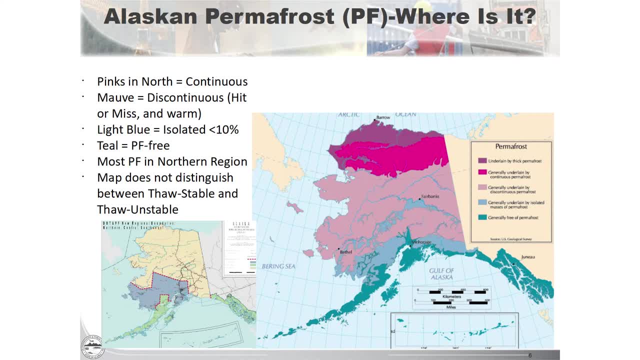 except maybe under a really big water body, It's going to be permafrost Pretty much a sure thing. The teal down near the coast is that is essentially permafrost free. There's very essentially no permafrost there. So some people look at this map and say wow. 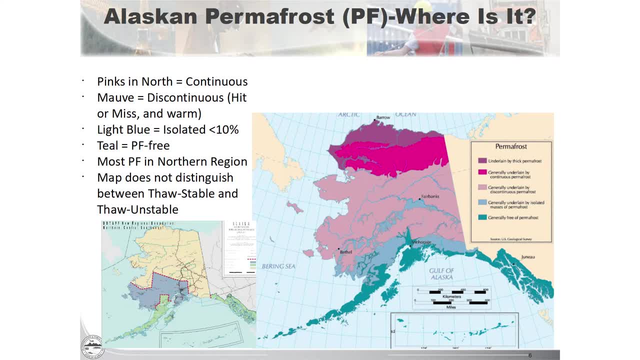 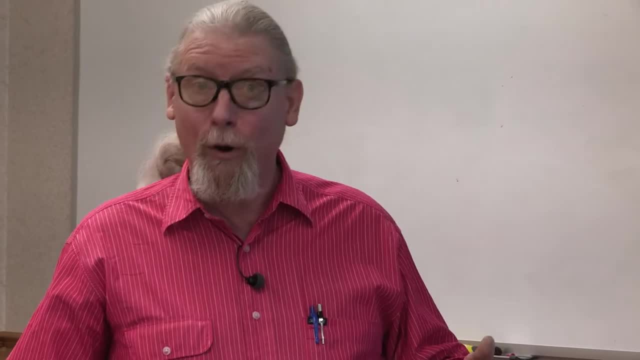 the teal stuff's no permafrost, Everything else is permafrost. Well, that's not really right. The blue, the light blue, that's isolated permafrost, which basically means there could be, but probably not. It's on the order. you know, 10% or less of that is frozen. 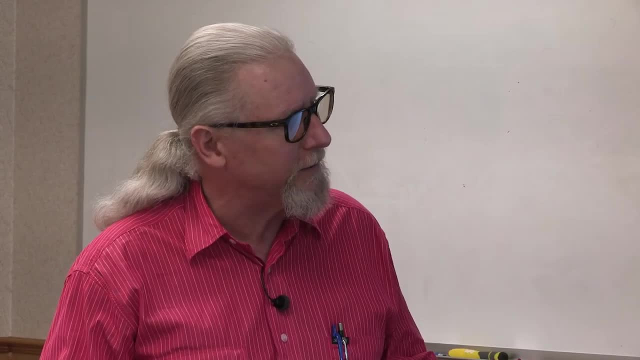 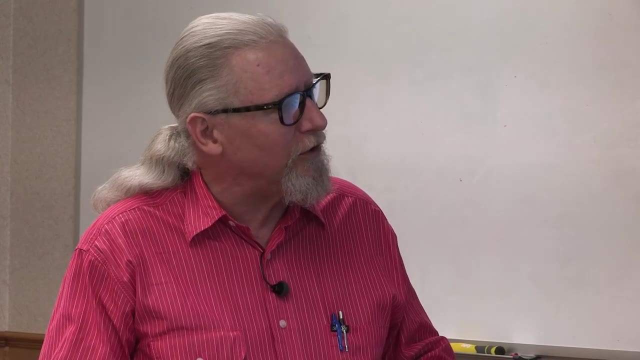 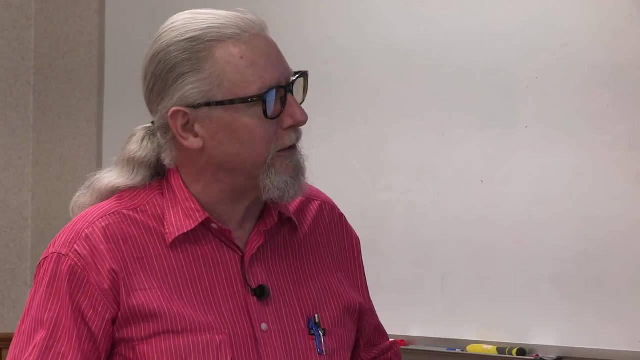 The mauve stuff in the middle, that big area in the interior Fairbanks that's discontinuous permafrost Might be. permafrost Might not be. So this doesn't suggest that almost all of the landmass of Alaska is permafrost, but more or less like the probability. 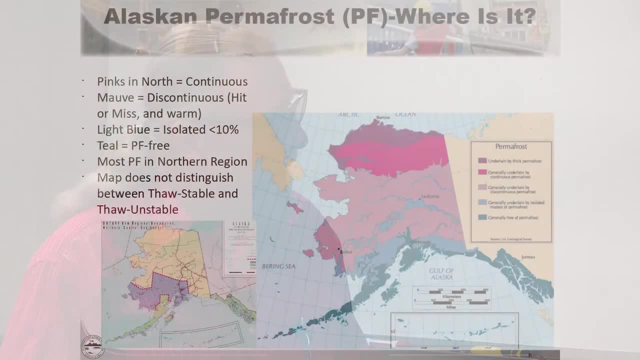 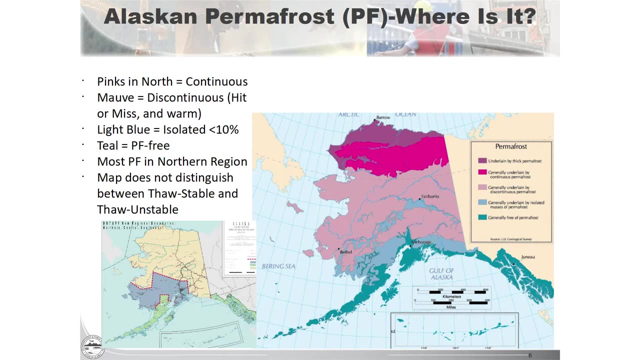 the probabilities of where it might be. Going back to our map of DOT you can see that the teal corresponds the no permafrost zone corresponds pretty closely with our south coast region. They were real excited when they got this little bit of YK delta and actually did get some. 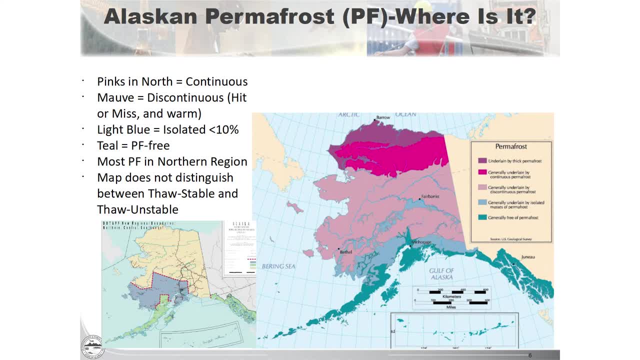 permafrost, but not an awful lot. There's actually quite a bit of permafrost in central region, but there isn't a lot of road system- excuse me, a lot of road system where there is permafrost, Bethel being exception. Chief Eddie Thompson Drive in Bethel is a notorious permafrost problem. 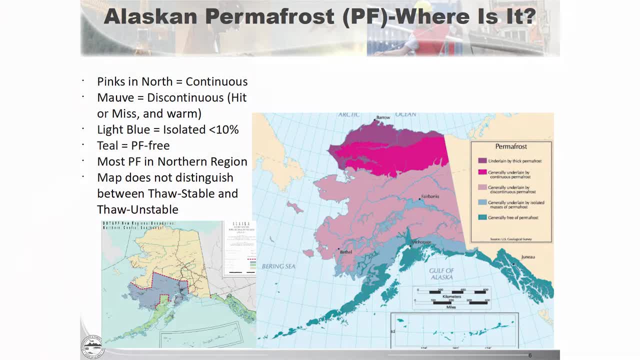 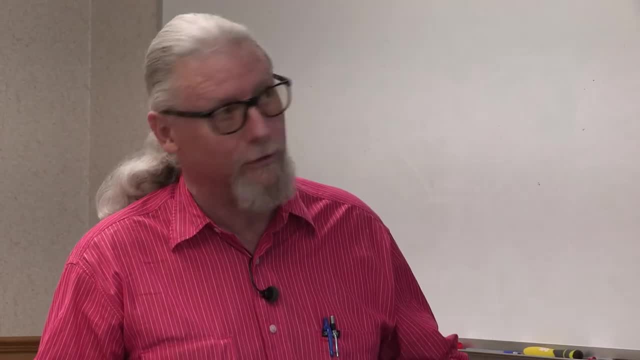 and there's some permafrost on the Glen Highway, in the parks as well in central region, But the vast majority of the permafrost in Alaska is in the northern region. The vast majority of Alaska is northern region And the other takeaway here is: this is basically telling you about. 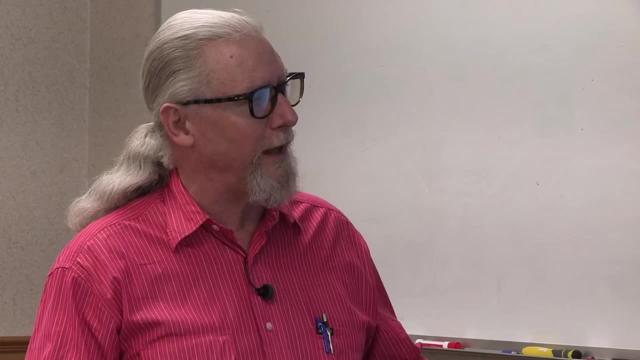 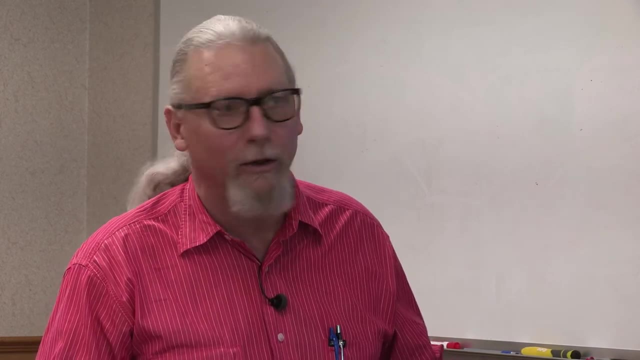 the thermal condition of the ground, the temperature. It doesn't say anything about whether that permafrost is thaw stable or thaw unstable. So don't let anybody show you this map and say, oh my God, all of Alaska is going to melt. because, number one, it's not all permafrost. 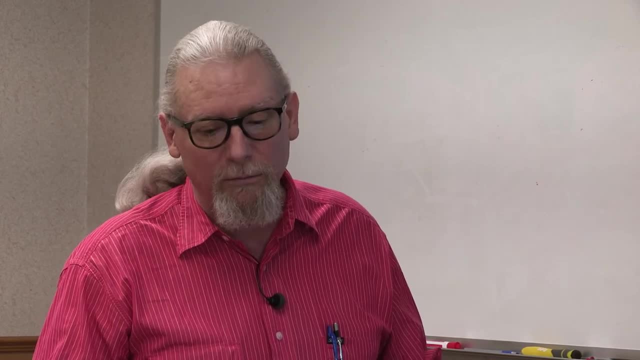 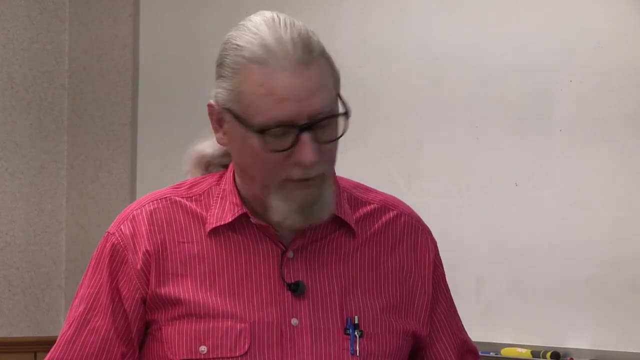 Those are probabilities. And number two: a lot of it is places that if it thaws, it won't hurt anything, But the thaw unstable stuff, the ice rich silt. that is a problem, And so why do we care about that anyway? Well, it makes it hard for us to do our job of keeping Alaska moving. 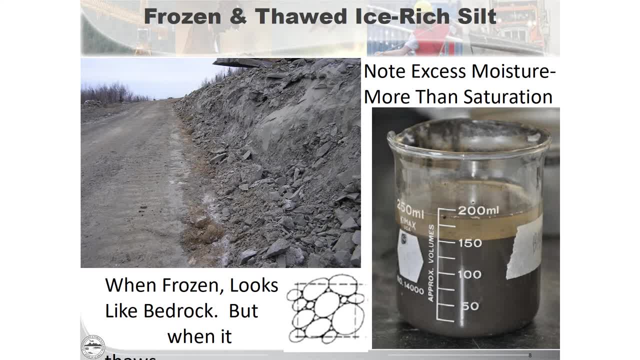 If you looked at normal soil, you know bedrock is basically continuous rock And soil is particles of rock And they could be silt or sand size, They could be gravel, It can be boulders, But the takeaway is is that you've got particles of mineral. 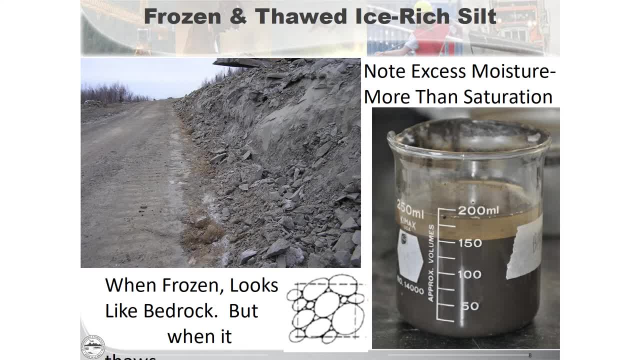 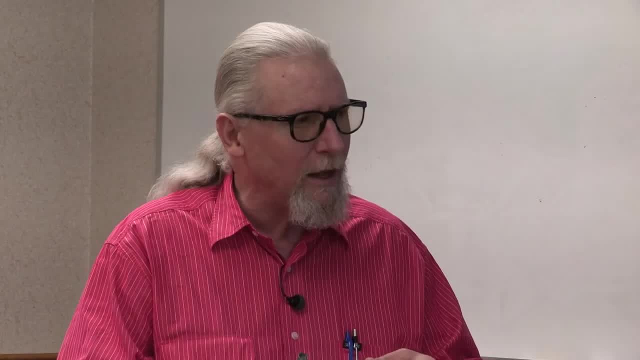 of rock, of whatever size, And between those they never nest back the way they you know to make them 100 percent solid, like they are in bedrock. There's voids And those voids can be filled with air. if it's dry, They can be filled with water. if it's saturated, They can be filled. 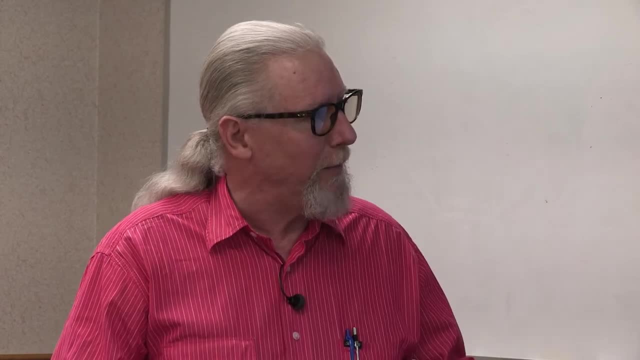 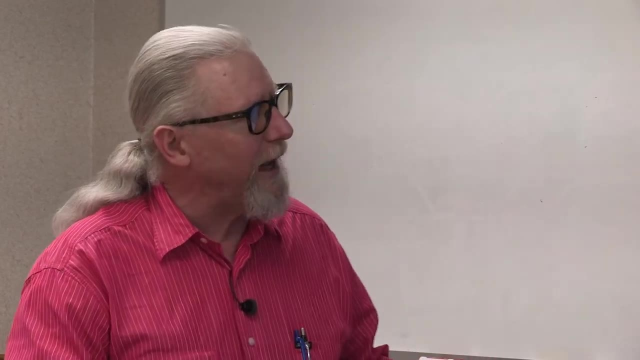 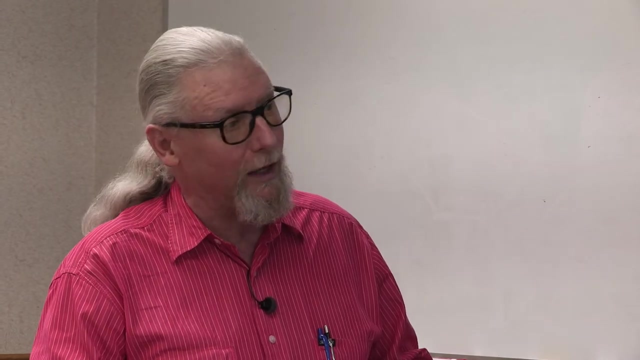 both if it's moist, And that's a pretty common case. But basically these particles are touching each other And then they're the void space. Well, if you were to excavate into ice rich ice rich, frozen silt and if you did it in the winter time, which would be the right time to do- 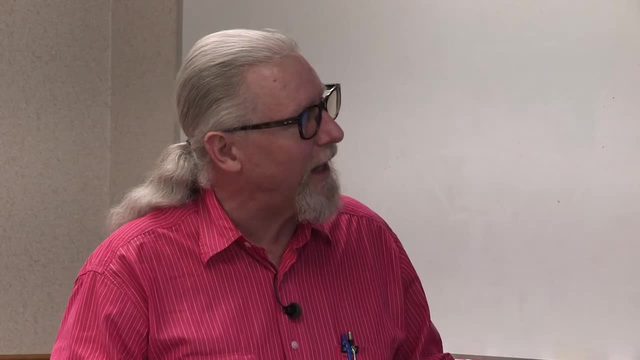 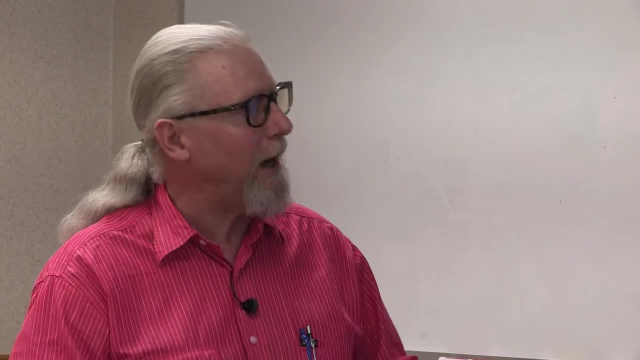 it, you would find that it behaves a lot like rock. It looks like rock. You'd have to drill it and blast it or rip it with a dozer, because it's not, because the ice is binding it together And so when it breaks up, it breaks up into chunks that look an awful lot like rock. But if you looked 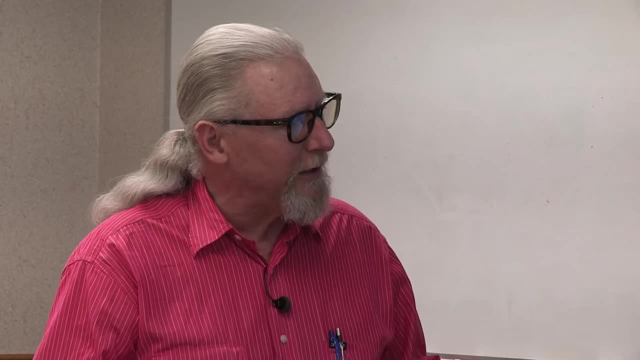 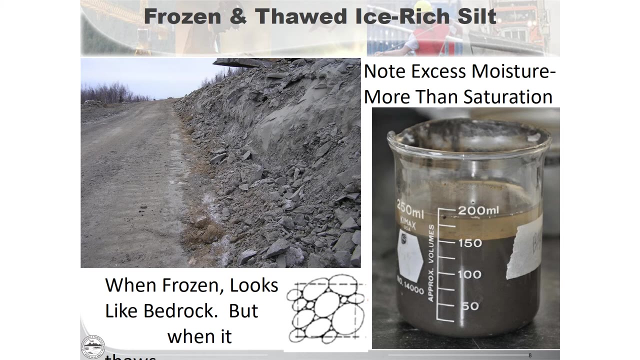 at it closely enough, you'd see that there's actually, instead of these particles touching each other, they're actually there's too much ice. There's more ice there than there is void space. if everything was touching each other And those particles are sort of floating in a matrix. 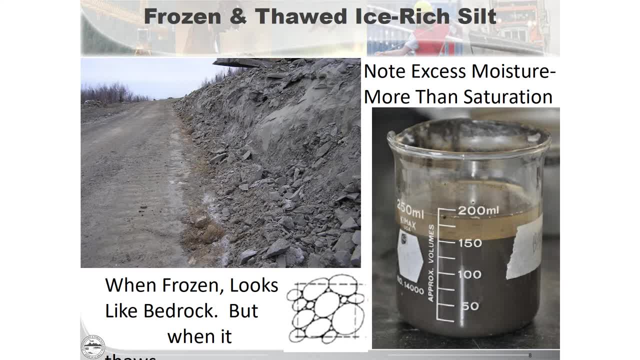 of ice. So if you thaw it out, look at the beaker on the right there, The stuff at the bottom is totally saturated, loose silt. It's basically like mud, But on top of that there's standing water. Something like 20% of the volume of that beaker is excess water, And so if you had 10 feet of this, stuff and you thawed it and you built a road on it and you thawed it. two feet of that is going to settle out just because of the excess water. But it's going to settle more than that because this unconsolidated silt you put a load on it. it's going to squeeze more water out of that. So if you 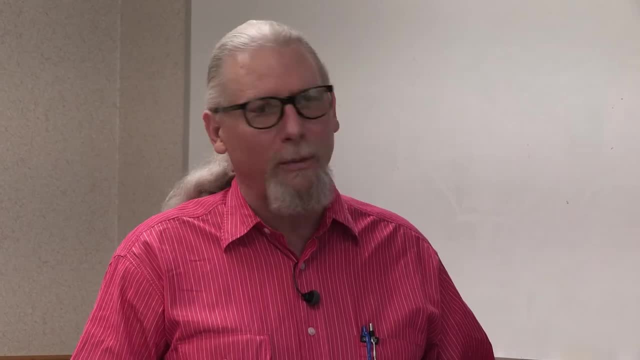 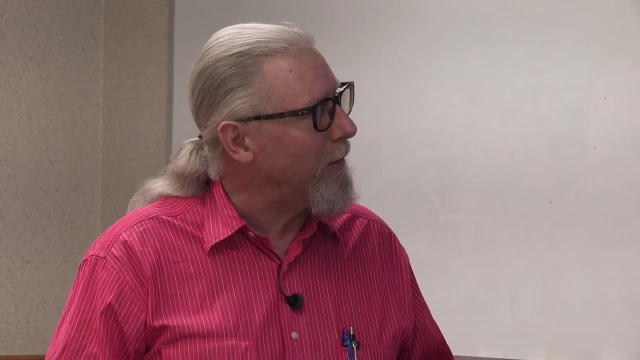 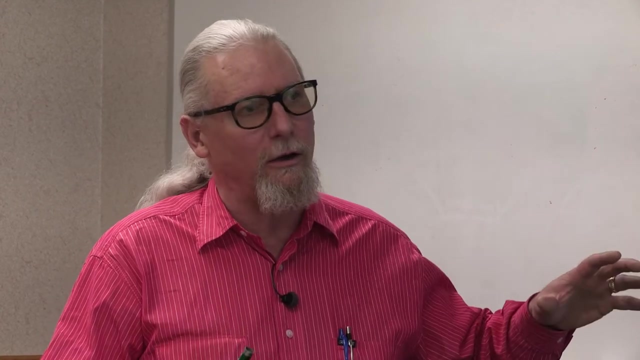 had 10 foot of the stuff on the right and you thawed it, you'd probably see three or four feet of settlement of anything that was built on top of it. Now, that's bad enough, But if all this was uniform, if it was equally had an equal moisture content everywhere, and if it thawed all the same, 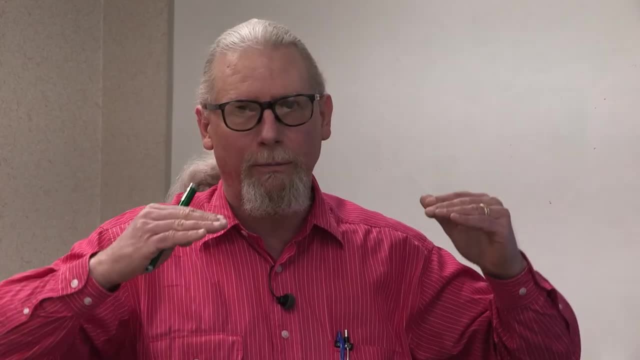 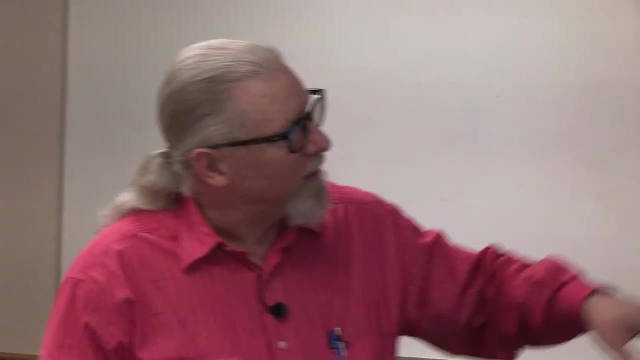 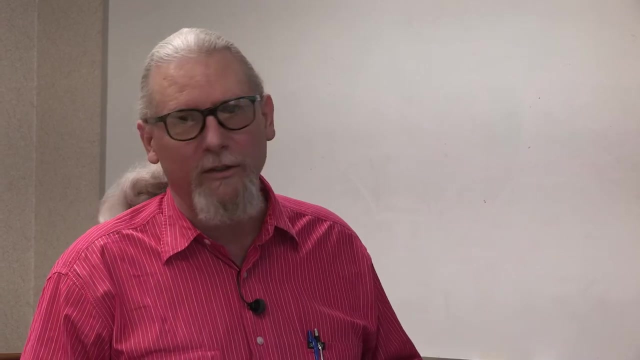 at the same rate at least, maybe your road would all settle at the same pace, And that sometimes happens. But sometimes we have massive ice And if the silt is thawing and settling- 30%, 40%- how much do you think the massive ice settles? Well, it settles 100%. 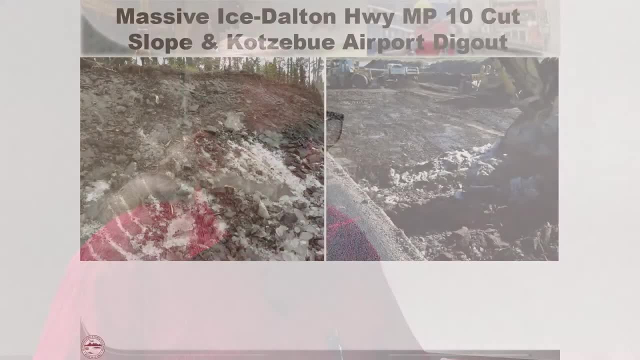 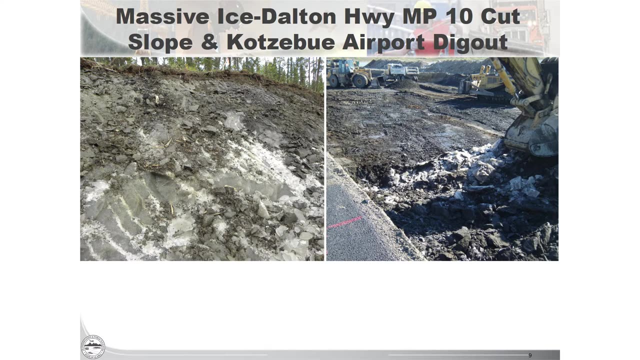 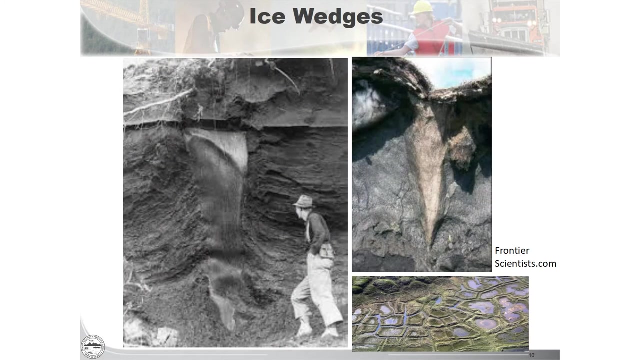 right. So now you've got differential conditions where it's thawing. The settlement is not uniform, and that gives us that differential settlement. There's a lot of different kinds of ice, that we can have different forms of ice, one that we deal with quite a bit, and 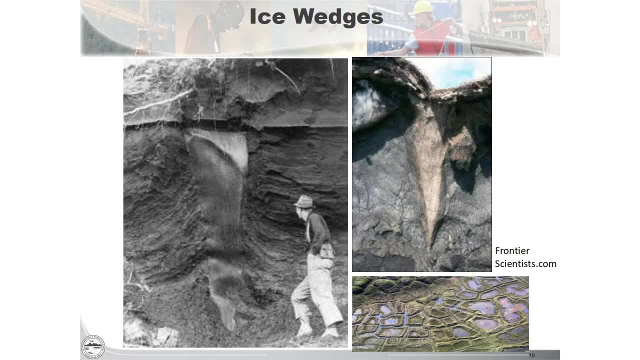 is really kind of interesting is wedge ice. It's this carrot-shaped structure. It looks carrot-shaped in this view because we're looking at it end on. But this goes back into the page and the slide on the bottom. that's what we call polygonal ground, And each of these lines 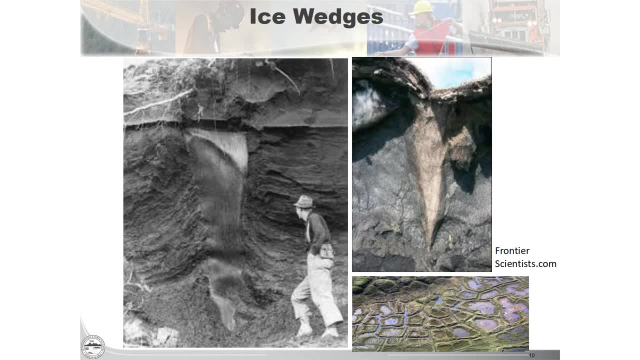 each of these linear structures is an ice wedge intersecting in with other ice wedges. So when you can see this, it's pretty clear And this is, like I say, very diagnostic of ice wedge country and common on the North Slope and other places as well. But this one on the left 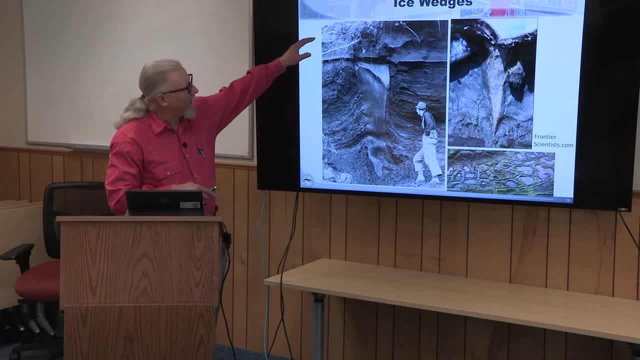 there was an ice wedge here that formed, but it got buried by overlying silt. It's windblown silt lust, probably that buried this, And so now you may not see this kind of, you would not see this kind of expression on the surface And you might not be able to tell at all that there was an ice. 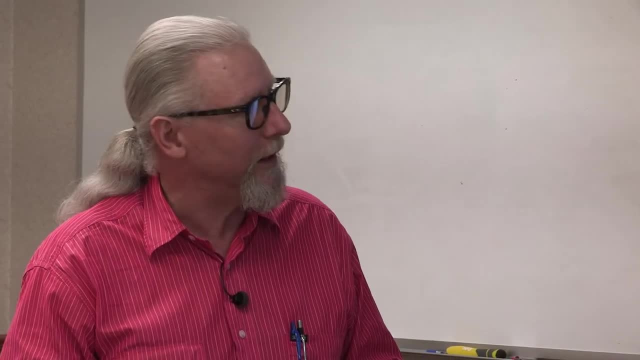 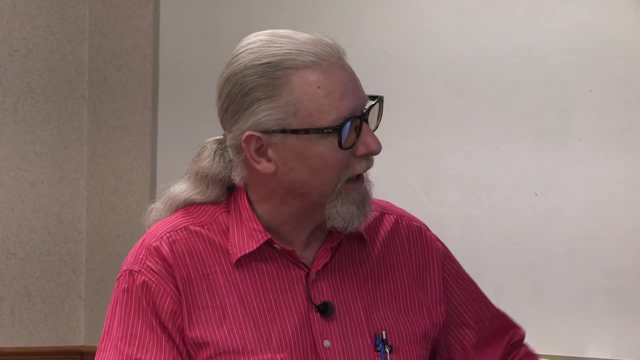 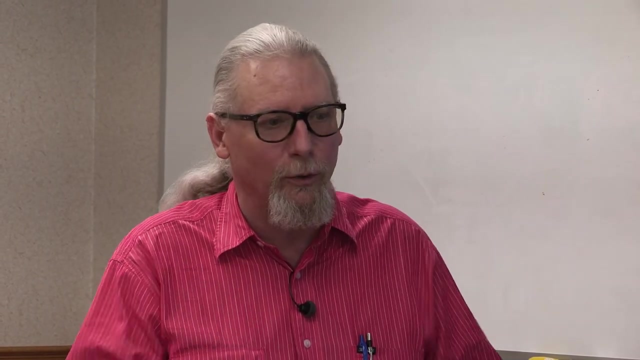 wedge here. When we were drilling on the Dalton Nine Mile Hill project, we drilled through places we went through 80 feet or more of pure ice. This is just a little guy here: 80 feet of pure ice And there was no way of seeing that from the surface. There's no visible, And that happened. 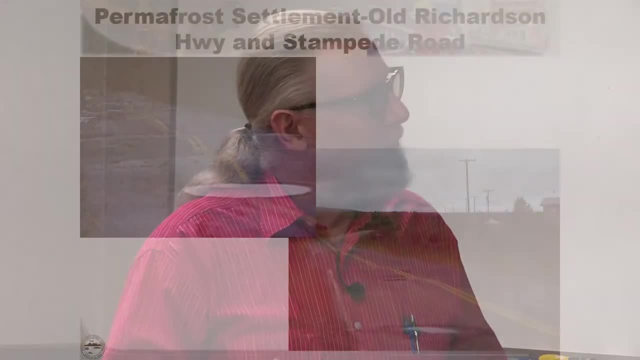 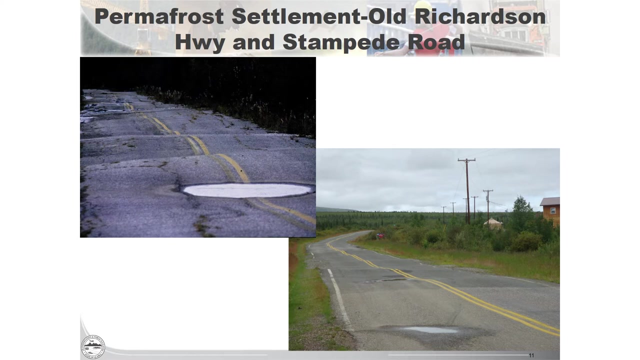 several times. This picture here is really famous. That's why I showed it twice. It has been used for a lot of presentations and it is including as an example of frost heaving. It's not frost heaving, This is permafrost thaw. In fact, you can almost imagine those ice wedges. 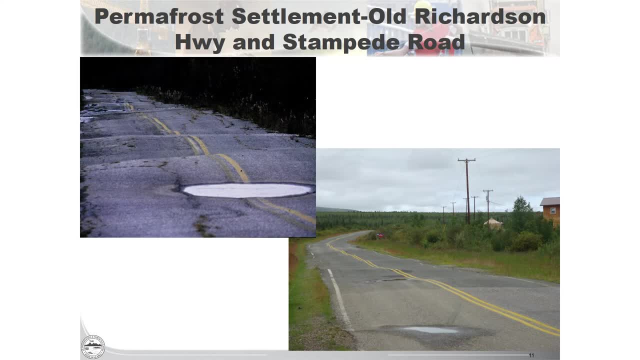 that polygonal ground and those ice wedges thawing out. We see a similar behavior in other places, but this happens to be on the Richardson Highway out towards Delta, the old Richardson Highway. This section of road is closed, by the way, And we didn't build it that way. 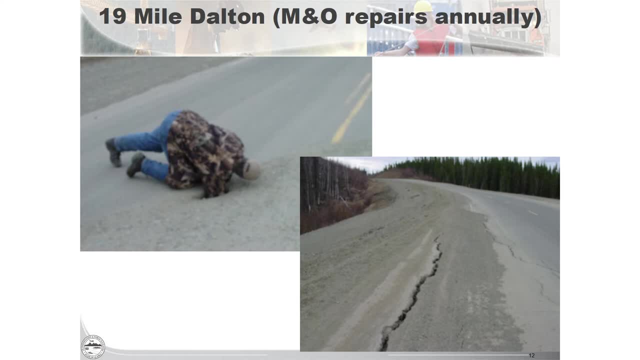 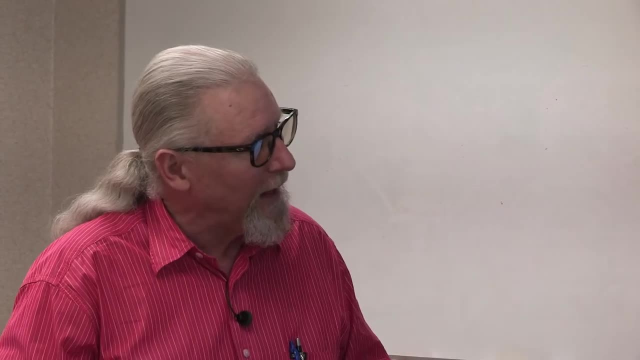 Here's a place where we built the road, built Dalton Highway over through a valley fill. That's where you build a road from one hilltop to another across a valley And there's massive ice underneath there And it's settling due to thaw settling vertically. It's also creeping. 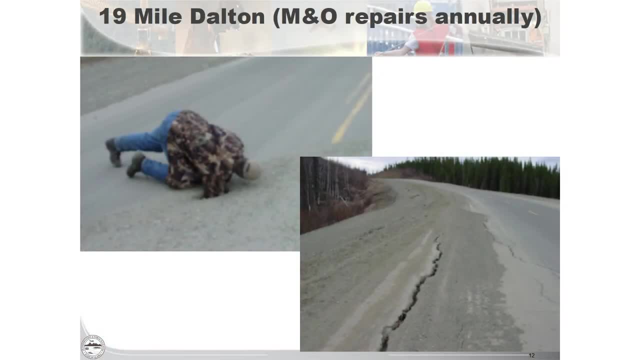 downhill And our maintenance and operations folks have to work on it every year hauling in a lot of gravel. And yet right up the road here you go through a bedrock, cut As you get out of that fill and off the ice into bedrock. that pavement has been there. They paved this in 2004,. 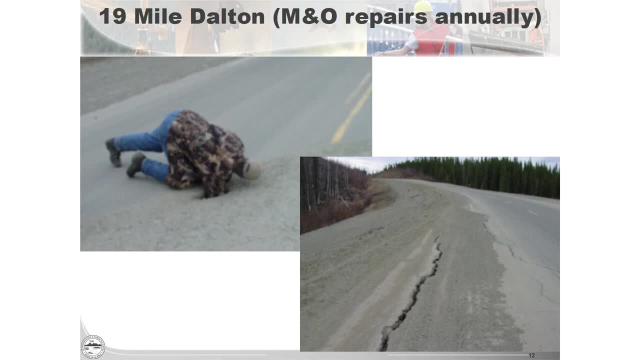 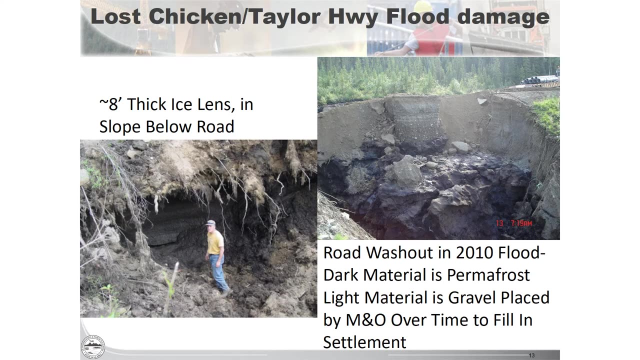 and it's great. It's smooth and the original striping is still in place. This is up by on the Taylor Highway, up a little past Chicken. This is a roughly eight-foot-thick ice lens. It's not a vertical structure, It's a horizontal structure. 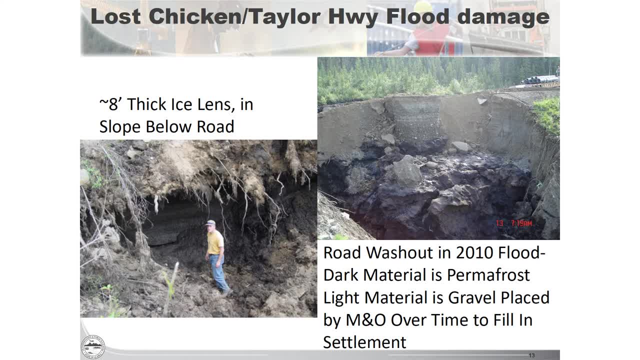 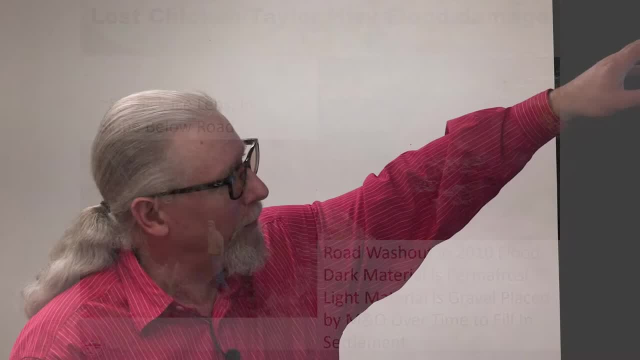 It was exposed by placer mining in Lost Chicken Creek, And what you can't tell here is that the road is right up here, And between the ice lens and also just probably ice-rich permafrost thawing, it used to settle to the point where our M&O folks had to haul in a. couple feet of gravel every year for a couple hundred-yard stretch to keep the road open. Interestingly, in 2010, we had a lot of flooding up on the Taylor Highway and the road washed out here- Not necessarily related to the permafrost, but it exposed it. 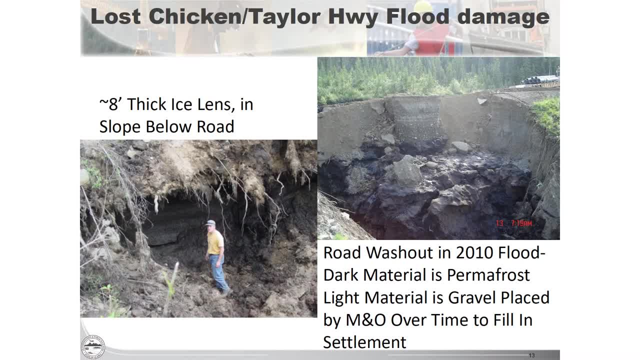 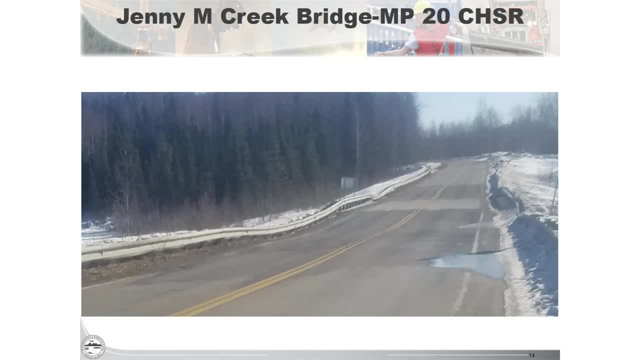 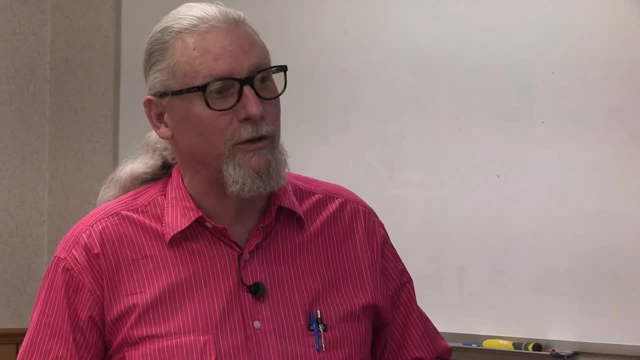 And one of the interesting things here is you can see the old permafrost at depth and the different gravel layers that have been built up over the years to keep the road in place. Bridges tend to do pretty well. We build bridges on piles unless the ground conditions are really. 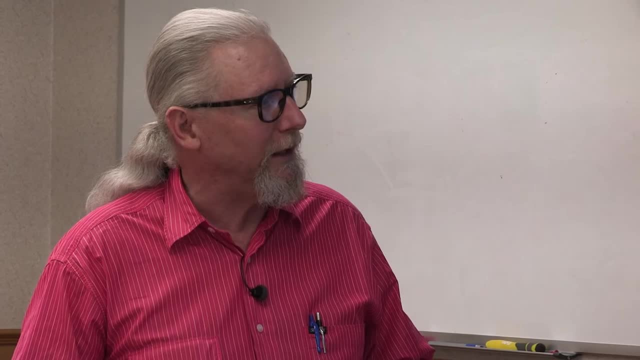 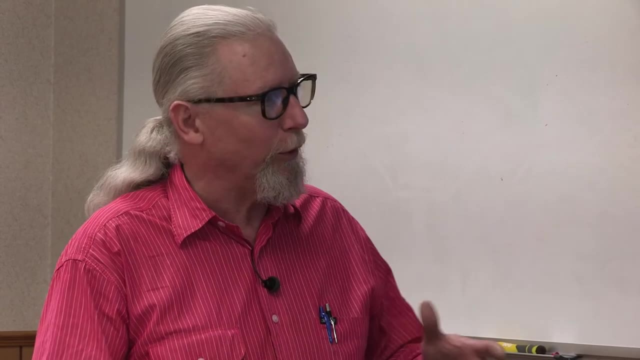 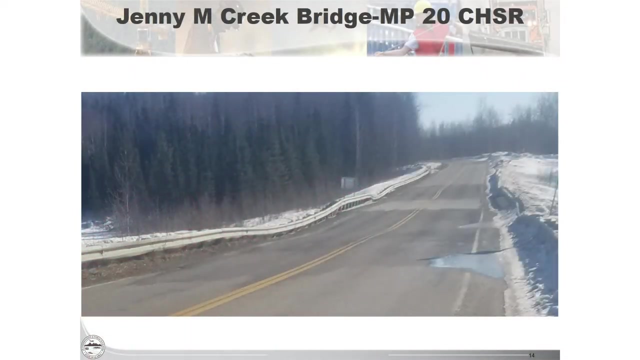 good, And we put those piles pretty deep. They either go to bedrock or they go to thaw-stable material, into gravel, very dense material, And so the bridges don't move, The approaches, on the other hand, not so much, And the guardrail is really an interesting thing to look at because 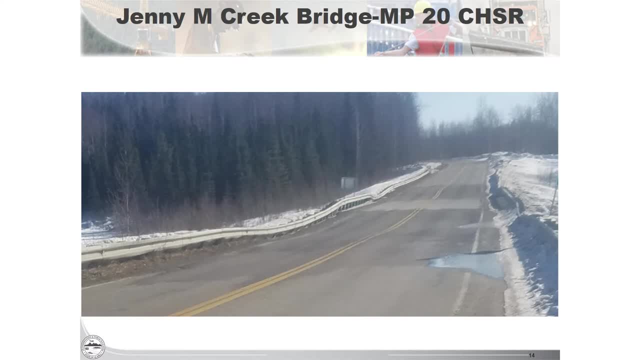 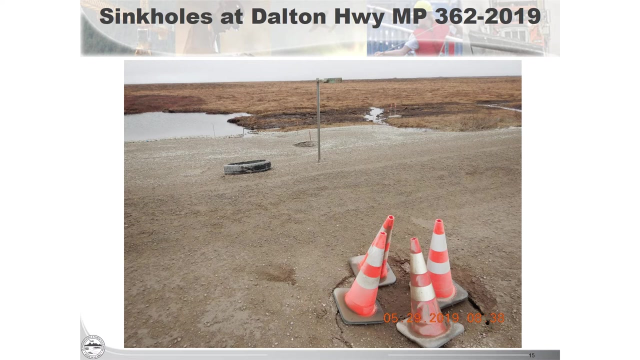 you can tell a lot about what's going on in the ground, But the ground is a little bit more much on the side of the bridge, where the approaches are settling. This is up on the Dalton Highway. This picture was taken in 2019.. The embankment was built in 2018.. 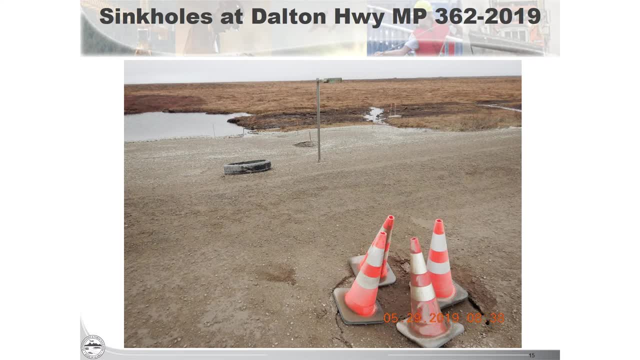 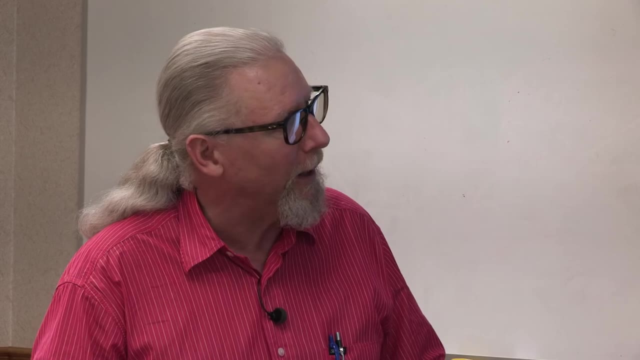 There's a series of linear sinkholes along the road here And our maintenance guys are grading this and filling them back in, which is why you don't see so many right there. But a takeaway is linear pattern and after this photo is taken, another linear pattern of sinkholes opened up. 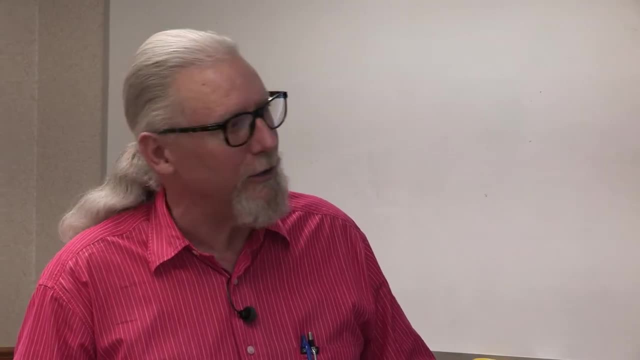 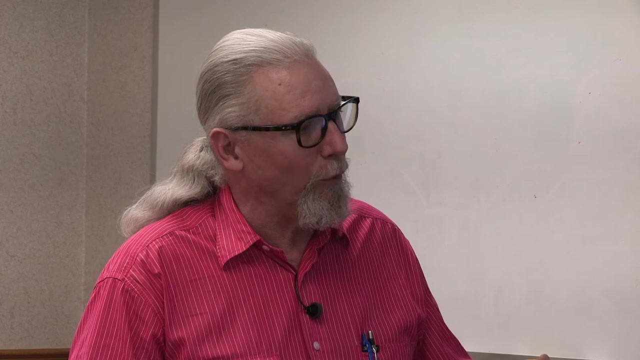 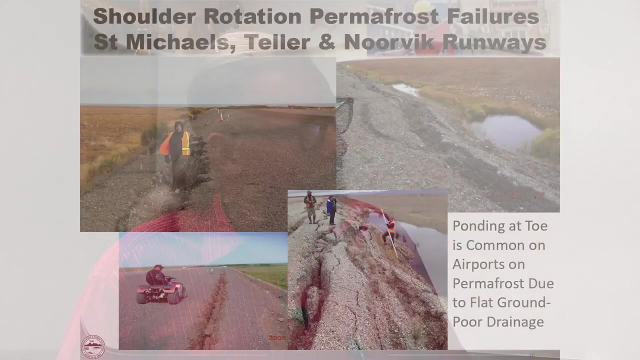 in the same general area. If you were to look at this from the air, you'd see the polygonal ground in the area. So what we've got is a road over ice, over ice wedges, and, for whatever reason, we, it must have initiated some thawing in those. These shoulder failures on airports on the west. 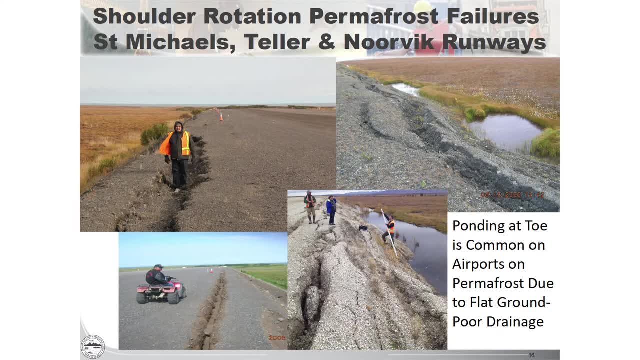 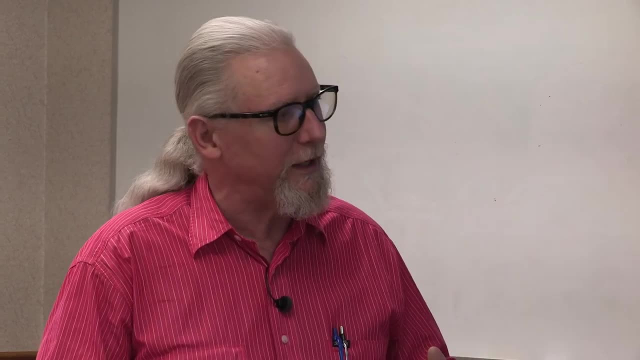 coast are ubiquitous. I show this is just three runways, but I could show you many others. What happens here is these airports are built pretty well. They're pretty thick, They have foam insulation in them most of them, and the runway itself, the center of it, is thermally. 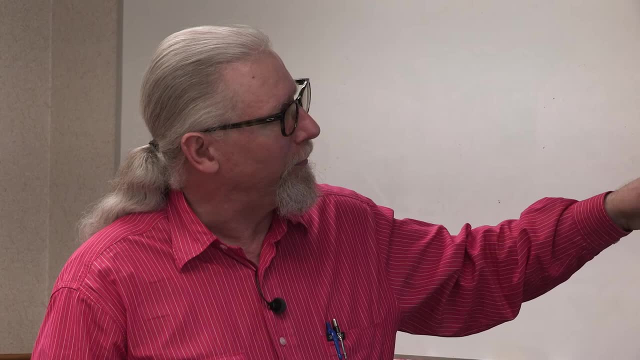 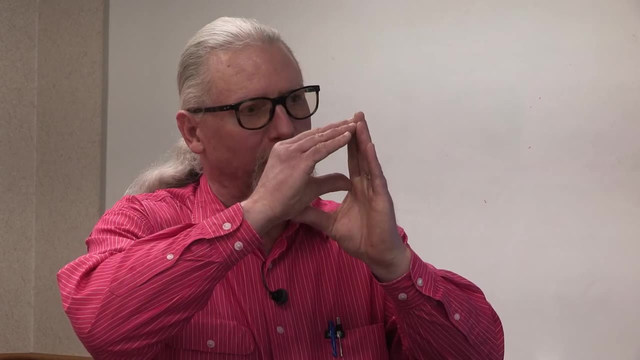 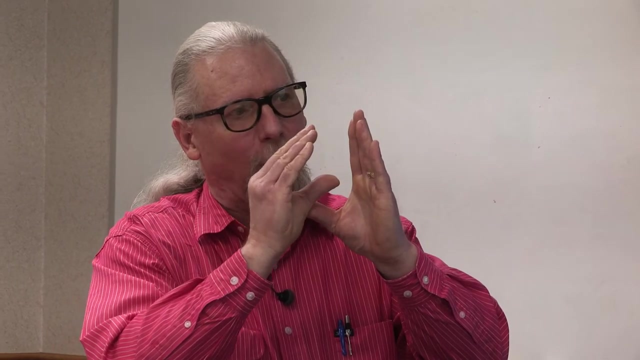 stable. But what happens is the worst thawing occurs on the slope and at the toe of the slope, and so as that toe of the slope and the permafrost underneath it warm up and thaw, The slope starts settling down and and rotating out, so it ends up becoming both as vertical and 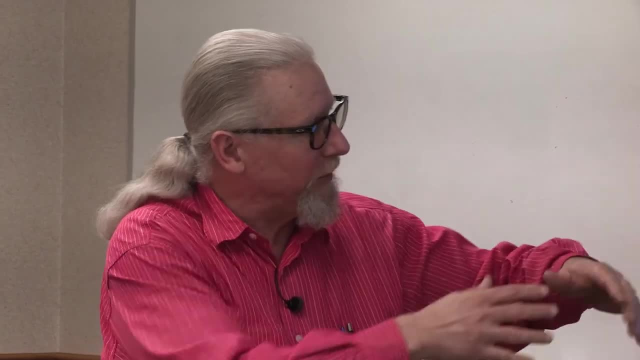 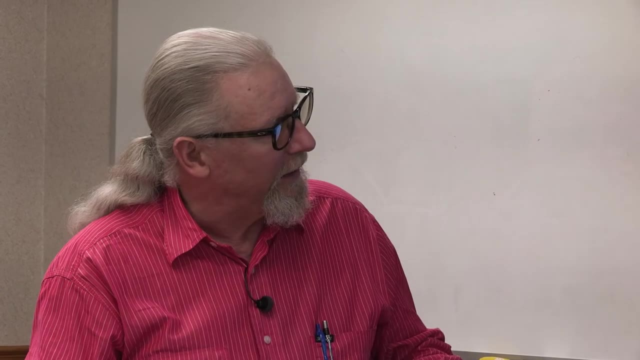 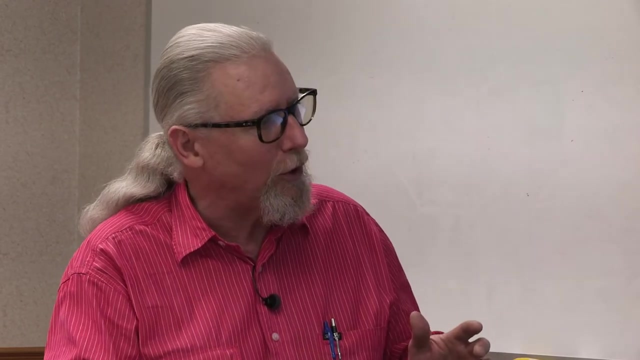 horizontal motion and that's what opens up these cracks, and so there's, like I say, both a vertical and a horizontal component to that, that motion. Frequently, these runways are built in flat ground and so, as the toe and the surrounding area right around the toe thaw, they create ponds and standing. 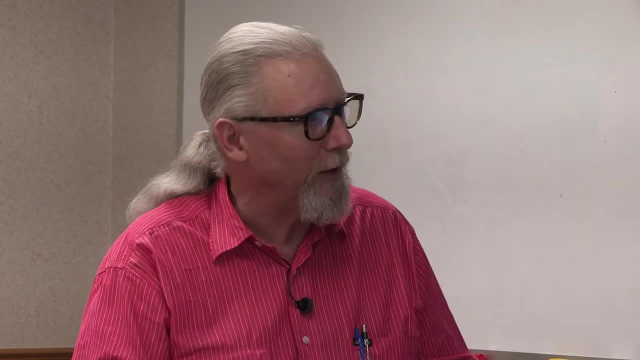 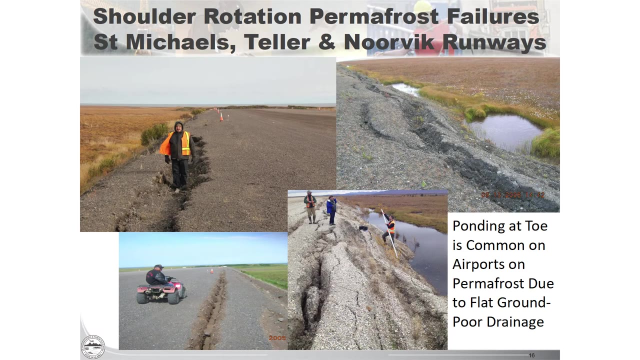 water. Water is a great way of thawing permafrost, It's a great way of imparting heat energy into the ground, and so that exacerbates the problem and it just becomes a vicious cycle. Our standard policy when we- when we do work on one of these things, is to try to fill that pond up and displace the water. 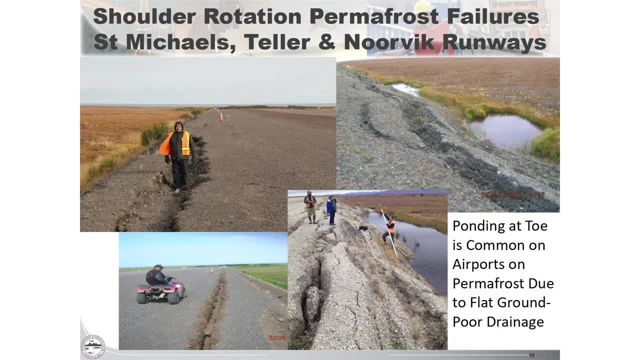 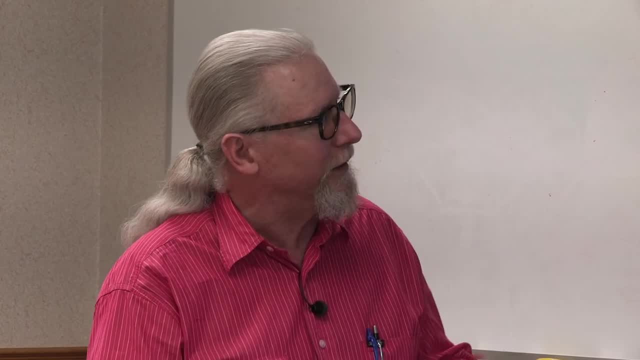 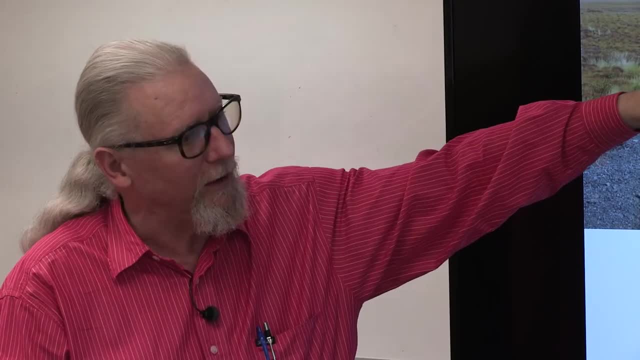 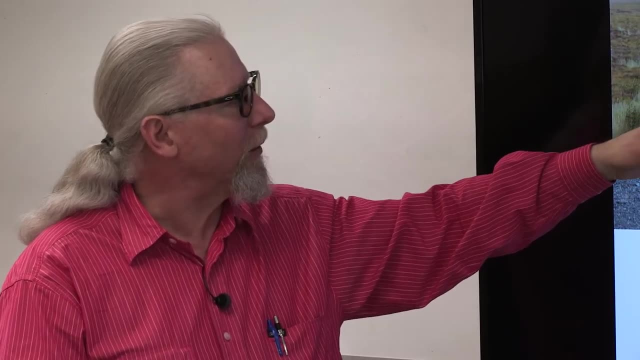 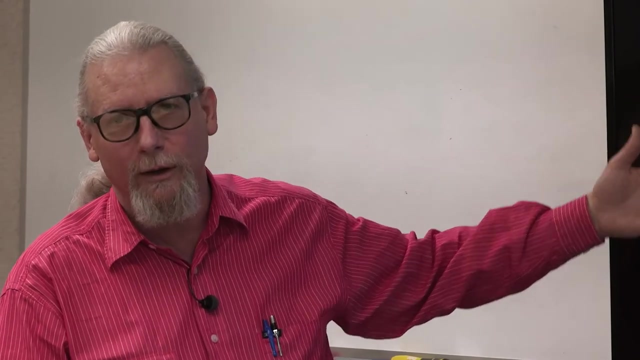 The main air main runway. then there's this flat safety area. so if they get off of the main runway they are still on flat ground. If they get so far over here to where they catch a wheel on this thing and flip over and do a ground loop, they were like two more feet from falling off the edge of the embankment and doing a ground loop anyway. 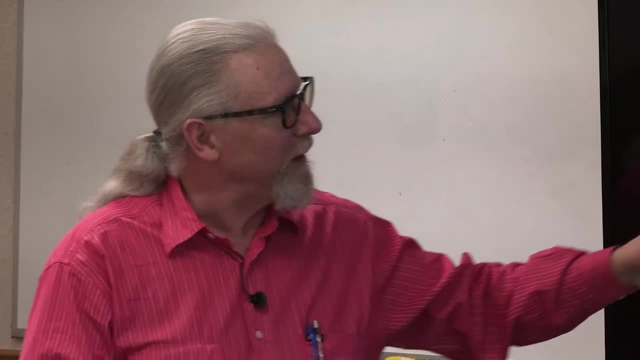 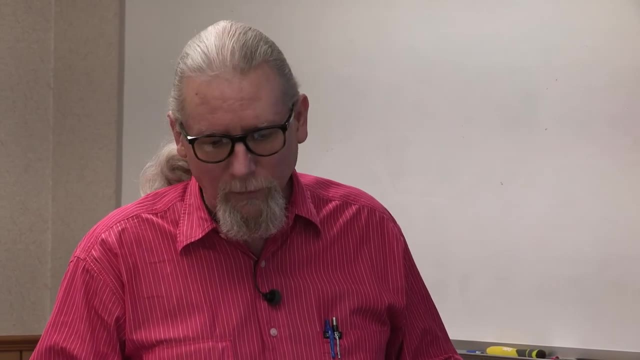 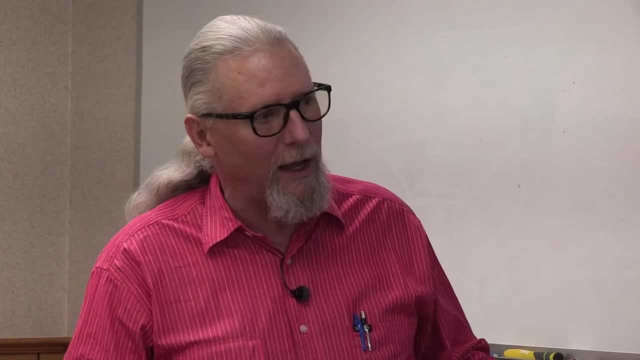 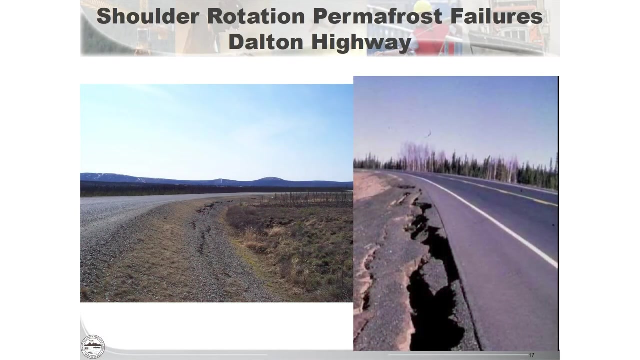 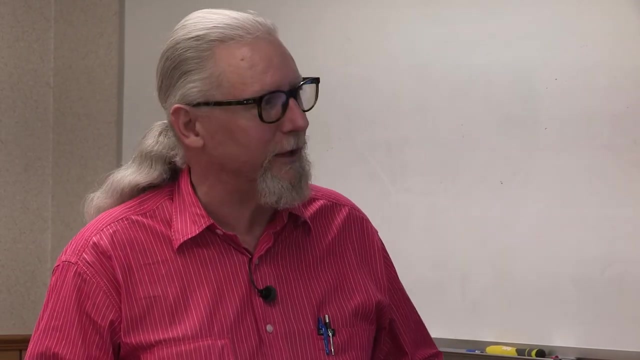 So these are not operationally that critical, unless and until these cracks start working their way up into the lighting system or start affecting the nav aids. On the highways, on the other hand, that's a little different story. we don't have a 75 foot wide safety zone, safety area on the highways, and this doesn't look terribly bad. if you got ran off the road here you could probably make it to the bottom one on the right that that shoulder is probably four feet or maybe six feet wide, so that crack is at least four, at least a foot wide. if you caught a tire and that going off the road at 60 miles an hour. 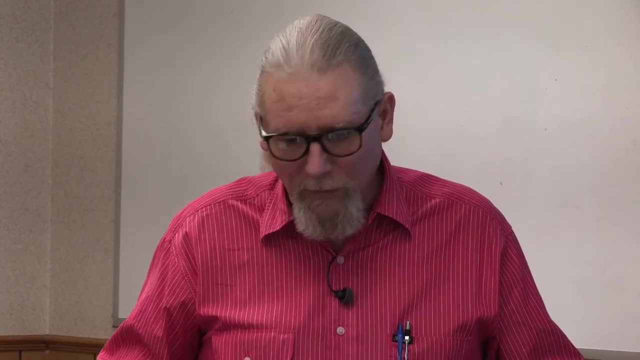 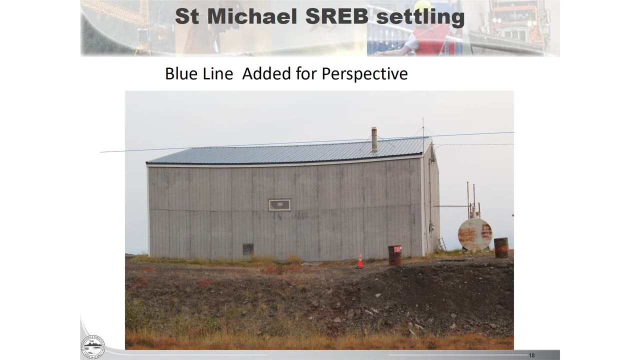 Boom. Remember the PF and DOT- and PF is public facilities- got to have a picture of a building. this is actually not that dramatic. the ground out here is not especially bad and the embankment was built pretty well. but it was built in 1983 and over the years it has settled and you can see the bow in the back of the, in the roof of that building. So what causes permafrost to thaw? The single biggest thing, the single biggest thing that's going to cause permafrost to thaw is the permafrost to thaw. The best thing you can do if you want to do thaw permafrost is to do what DOT does: build something on it. construction disturbance, particularly using conventional techniques, is the single worst thing we can do. I mean, first thing you do is you cut down the trees that are providing shade in the summertime, right, and then you strip off the moss and the vegetation which is what is insulating it in the summertime to keep that that summer heat out. and, yeah, you maybe make a low spot so you can collect water and pond water. 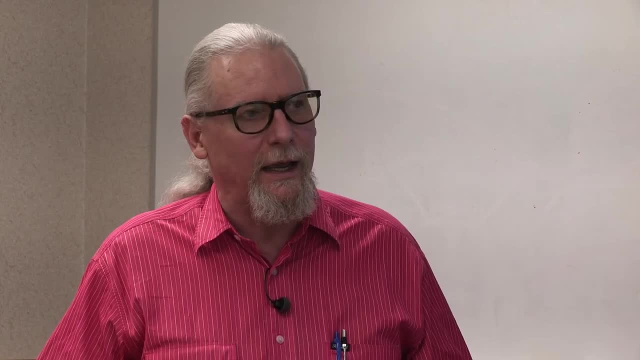 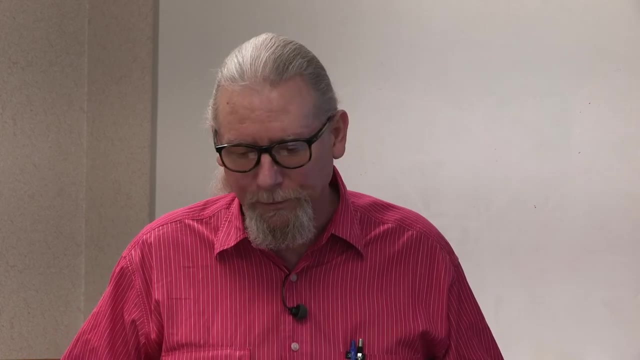 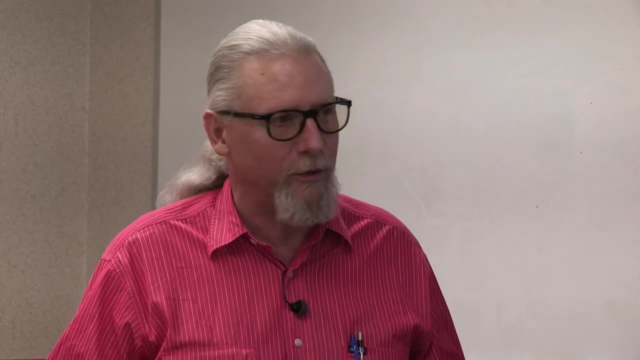 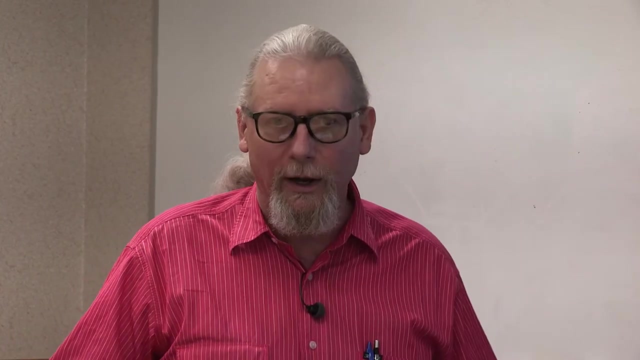 We already talked about this. water's got a lot of specific heat and it's a. it's a great way to impart heat energy into permafrost and thaw. it was talked about that a little more later. You replace the organic soil with gravel. maybe you do it in the summertime. you probably do in the summertime if you're using, you know, conventional techniques. so while you're doing all these not so good things for the long term, you're also exposing the ground to all the solar radiation and the warm summer air temperature. 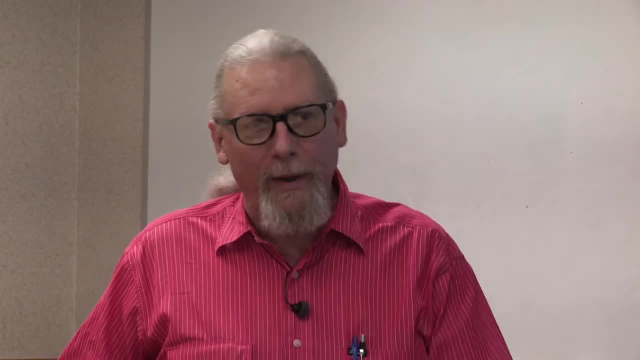 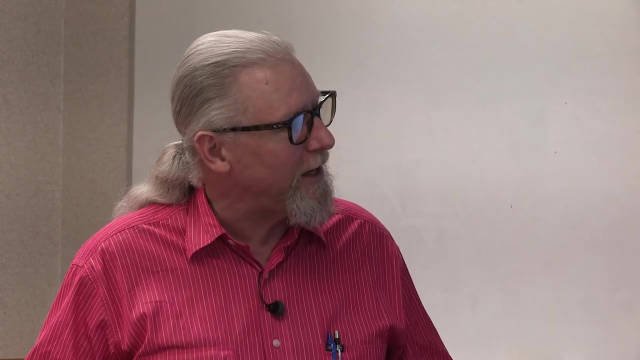 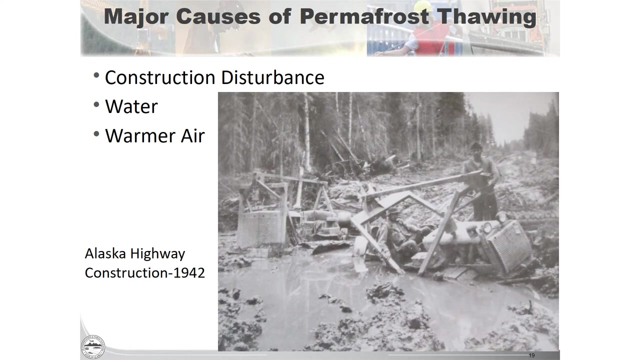 Then, If you really want to finish it off, you paint it black by putting asphalt on top of it so it can collect solar energy. so that the takeaway here is that the impact of construction, particularly if it's if it's poorly, poorly done, poorly coordinated, can be order of magnitude more significant than the air temperature raising by by a degree or two. still, air temperature does matter. 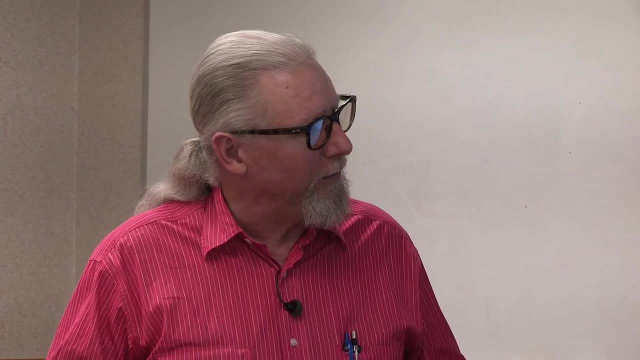 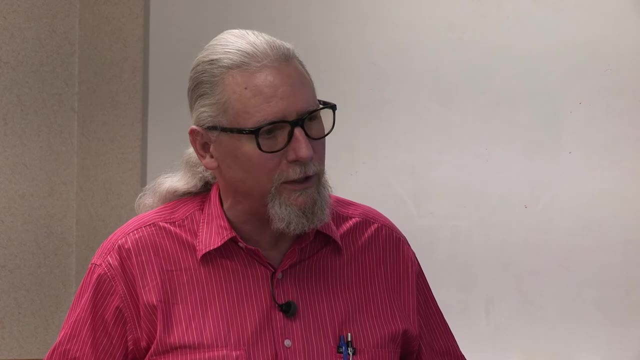 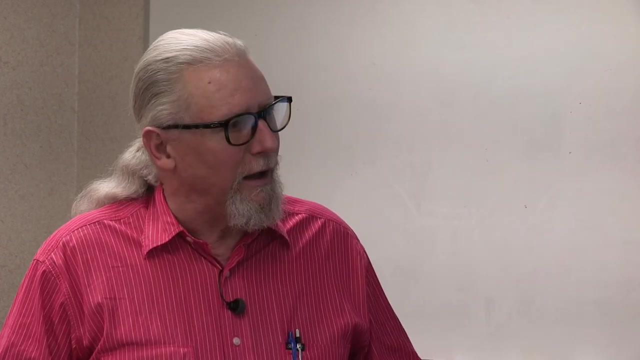 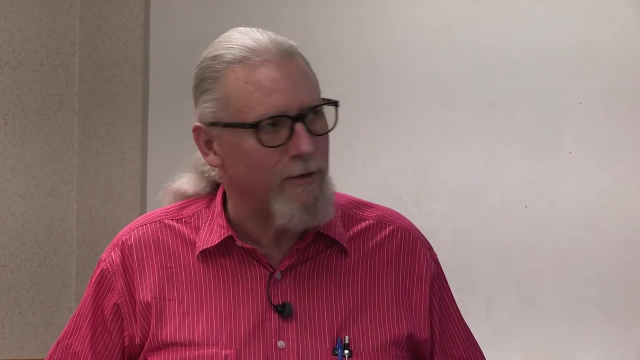 And you can upset the, the apple cart, particularly permafrost that is in this warm zone, this discontinuous zone around Fairbanks, and is sort of in this quasi equilibrium state. I promise some discussion about climate change. I'm not a climatologist, I'm an engineer, and I know a little bit about permafrost and infrastructure. I know a little bit about climate, though, and I 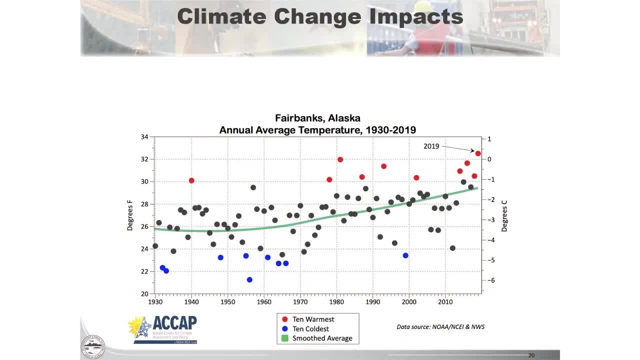 Couple of takeaways here. Each of these, each of these dots, represents the annual temperature for a given year in Fairbanks, from 1930 to 2019. so it's 90 years of record right? Couple key takeaways here. the red, the red dots represent the 10 warmest years. 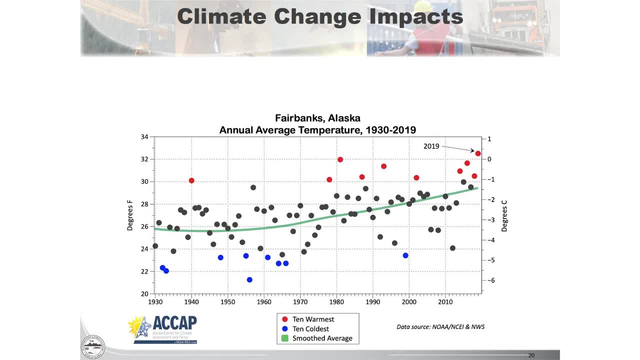 During that 90 year record, and nine of those 10 occurred since 1976, and the other one occurred in 1940, which is actually significant. let's keep that in mind. The blue dots represent the 10 coldest years and sorry, Rick, I think this one's supposed to be blue too. so the seven- seven of the 10 coldest years on record occurred between 1944 and 1976. 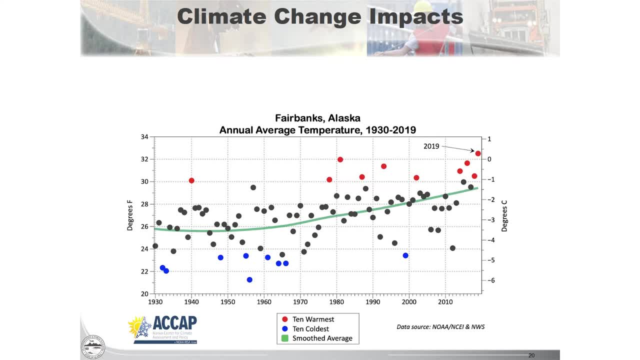 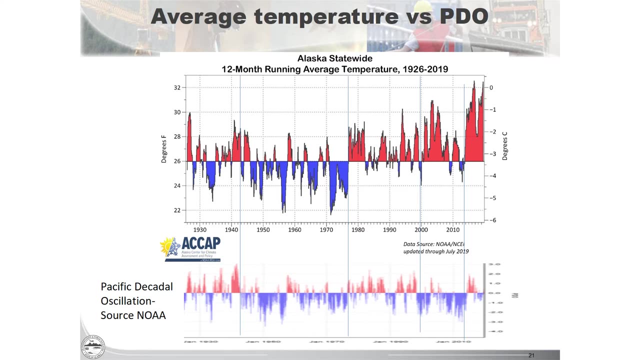 Then this blue curve, this smooth average curve, shows this trend sort of doing a curve curve regression. This is similar data here. Now this is Alaska statewide data, not Fairbanks. they're they're very similar. the patterns are extremely similar, but it's not exactly the same thing. from 1926 to 2019, which is roughly the same period of time- 90 some years, and this figure on the bottom is the Pacific decadal oscillation. I had to stretch it to make those scales match and truncate it because the record goes back further for the, for the PDO. 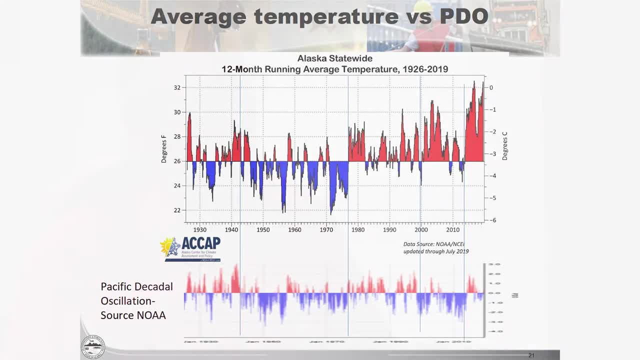 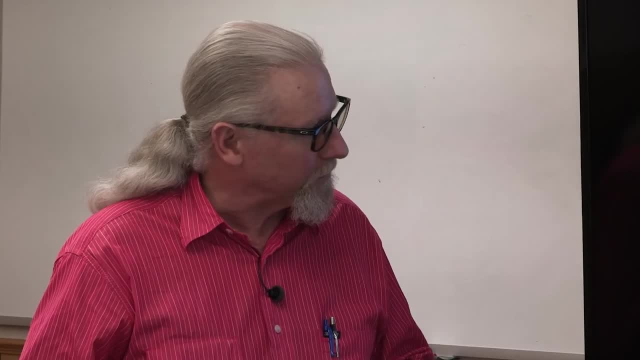 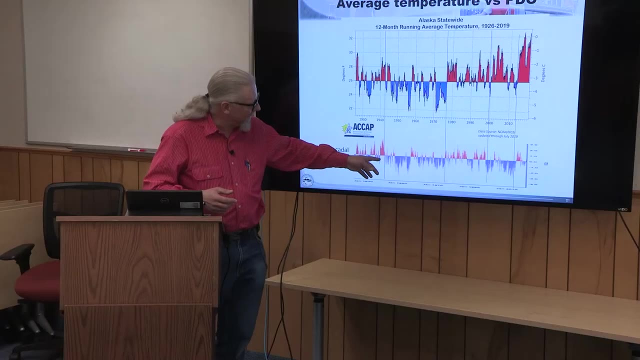 So Decadal oscillation, But the takeaway PDO is sort of like a decades long El Nino or La Nina trend and if you look at this, somewhere around 1944- 46, something like that- we went into a substantial negative, negative PDO index and at the same time we went into a anomalously low negative PDO index and at the same time we went into a anomalously low negative PDO index. 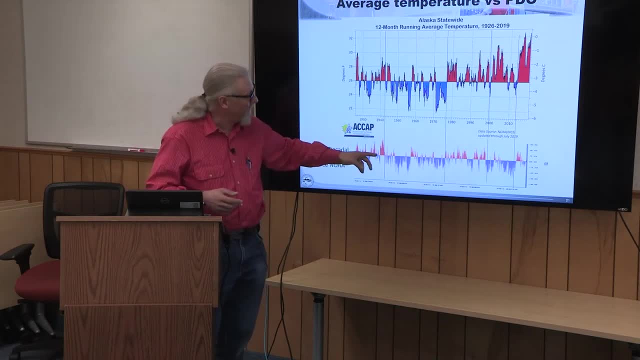 So this is the PDO, below 26 degree annual state temperature and even, and, and if you look at even the, the places where where there's high spots, they match high spots in the PDO. Similarly, prior to the night, that 1944 period, you've still got this, the same patterns and and this generally warm trend. in 1976, something pretty radical happened. 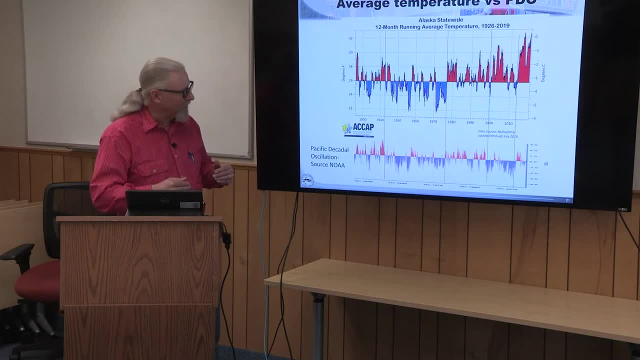 There was a- it's a step function. The temperature, the average temperatures, jumped up. You know several degrees, And so did the PDO, And again you can even see the localized differences. But the general trend was high for the PDO and for the annual temperatures. So some of us were thinking: 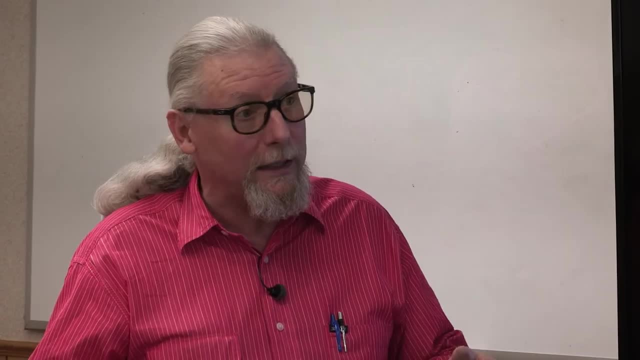 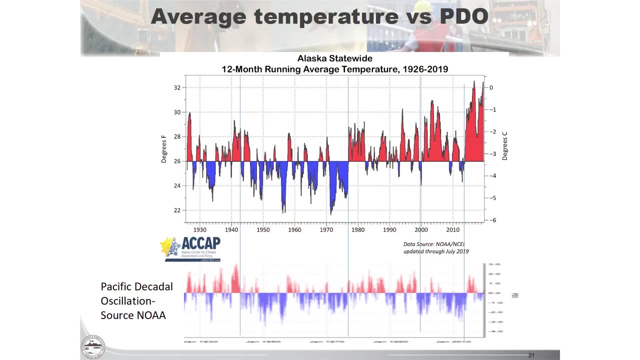 hey, somewhere around 2000,, 2005,, something like that, the PDO ought to switch back and everything ought to cool off again. Well, sure enough, the PDO did go back down the general trend, but the temperatures didn't go down. In fact, maybe they went up a little bit. 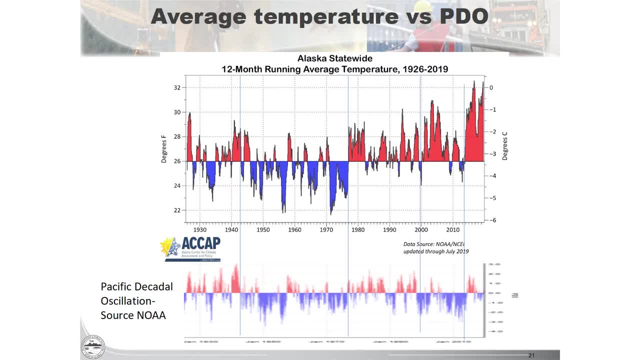 And so this is some of the warmer temperatures that those of us who've been here for a while remember the difference between Then, in 2014,, the PDO went up and the temperature spiked up again. So I'm not saying this upward trend isn't real. It is, but it's not this nice. 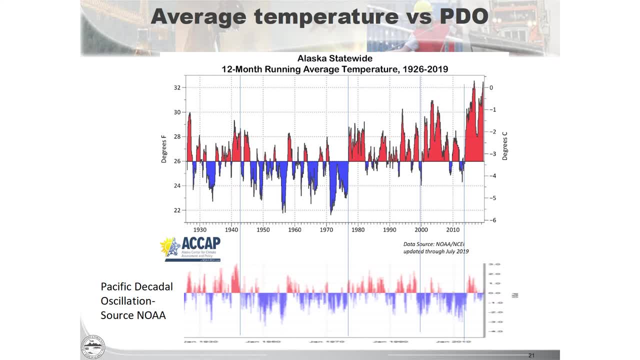 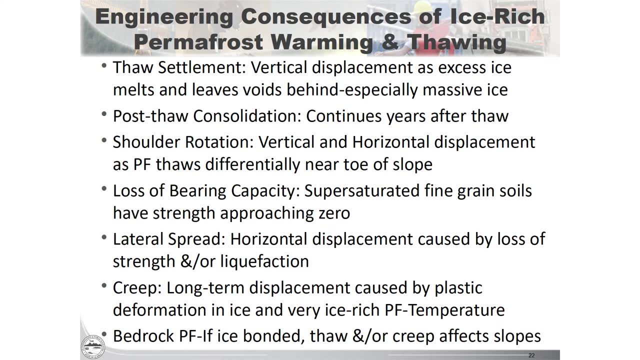 smooth curve or linear trend. There's a stepwise function in it And a lot of it's controlled by the temperature of the Pacific Ocean. So engineering consequences of building on ice-rich permafrost and then having it warm up and thaw- Probably the single most common and 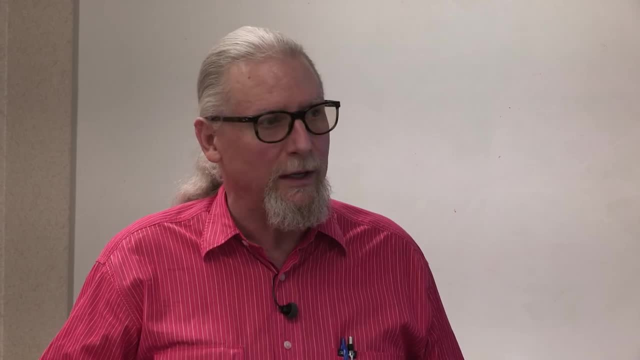 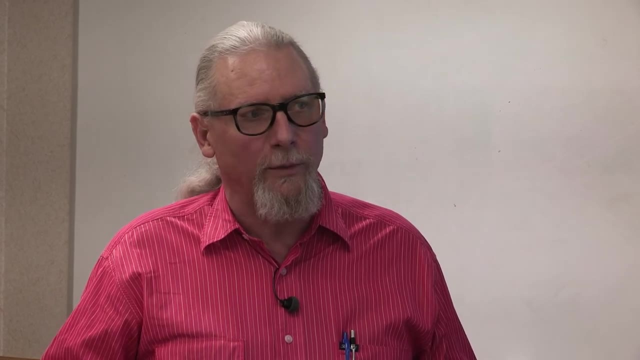 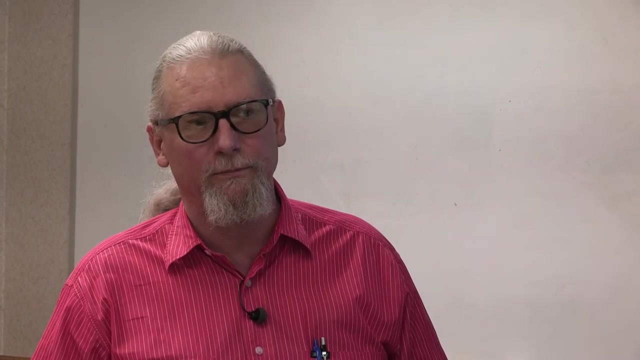 dramatic observation is this vertical settlement, particularly when it's differential settlement. If you drive out the Sties Highway, from time to time you'll see M&O having to fill in the roller coasters on the Sties Highway. There's places out there where the asphalt's probably 15 feet thick. 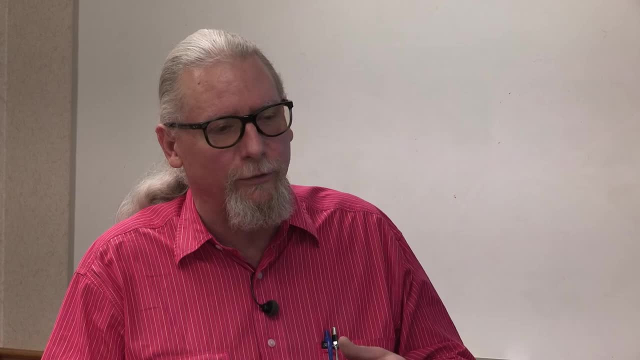 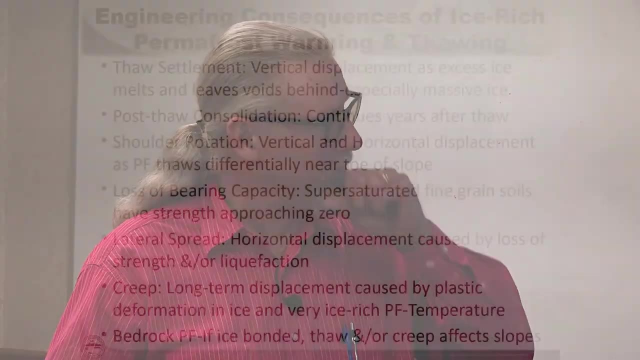 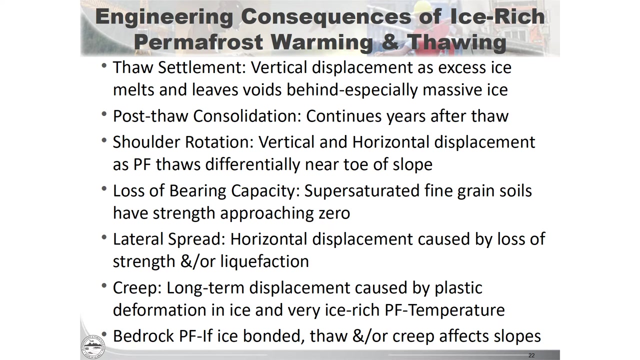 And that's due to that ice, whether it's excess ice in the frozen silt or massive ice thawing and leaving a void in the ground, the road simply settling down After the thaw occurs. you can still have additional settling as that previously ice-rich material consolidates. 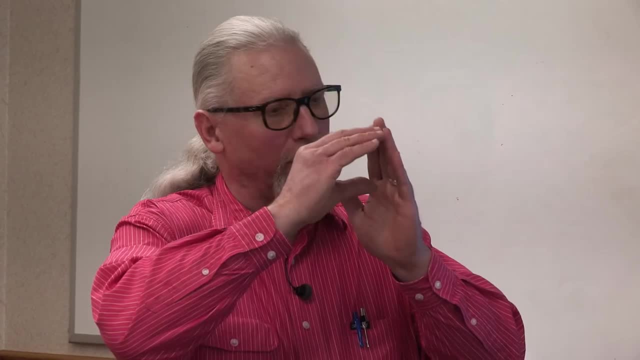 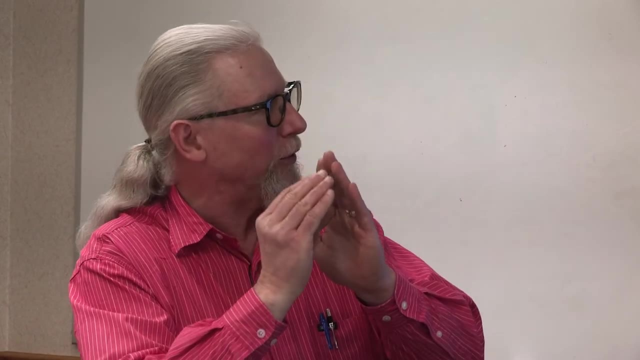 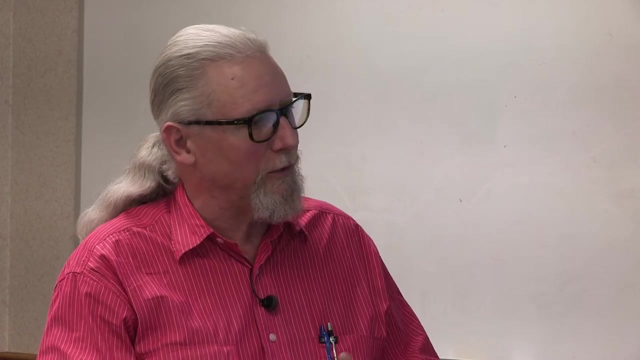 We talked already a little bit about shoulder rotation. That's where the toe of slope differentially settles, thaws and settles and the slope rotates out and creates those cracking That thawed ice-rich silt as it thaws and drains, before it drains, in particular. 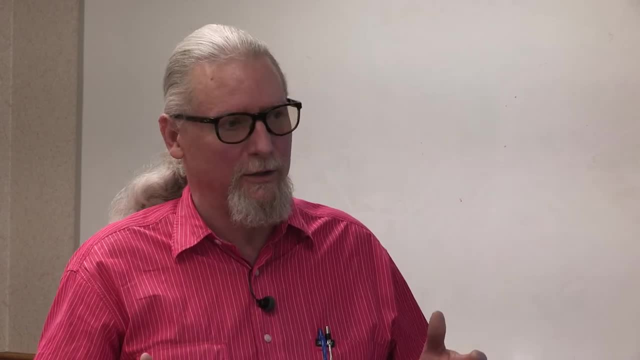 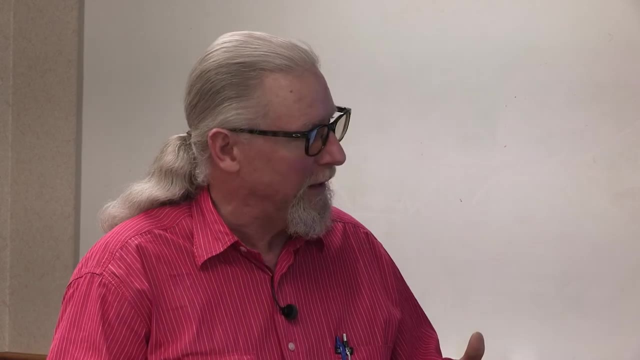 as it's saturated, has essentially no bearing capacity. It's like mud, It's like soup, And so if it's contained, constrained in the ground, that's when we get this vertical settlement. But if there's somewhere for it to go, it's kind of like building a road. 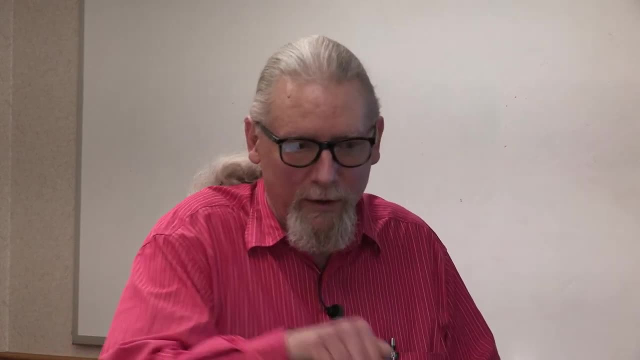 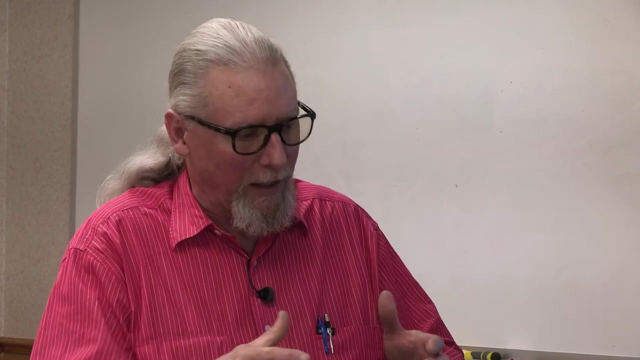 on a tube of toothpaste, The volume doesn't change, but where you squeeze it it squishes somewhere else, And so you can have that kind of issue, and that can lead to this lateral spreading, where the road is literally spreading out wider as it sort of squeezes out towards. 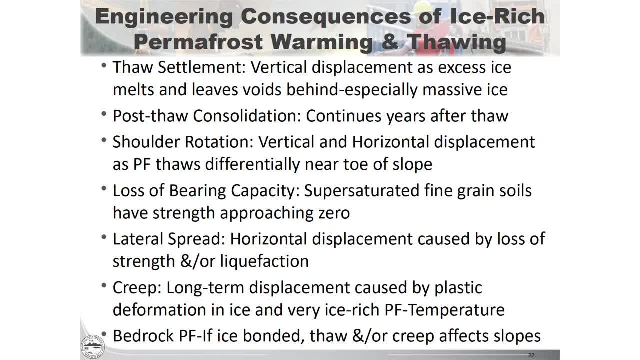 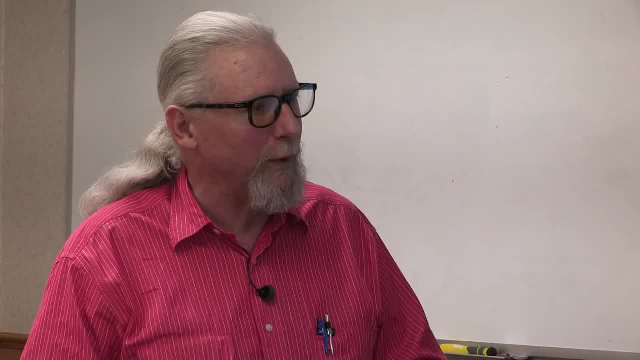 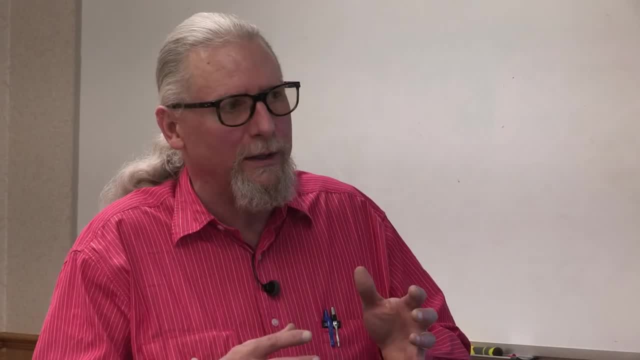 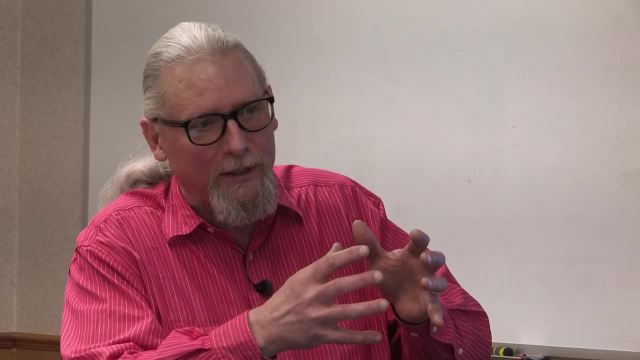 the sides And you'll see that manifested sometimes as longitudinal cracking in the middle of the road. Ice and really ice-rich silt can creep. That's like a sort of a slow-motion plastic flow, And so if you build something on a slope with ice in it, that ice just literally deforms. 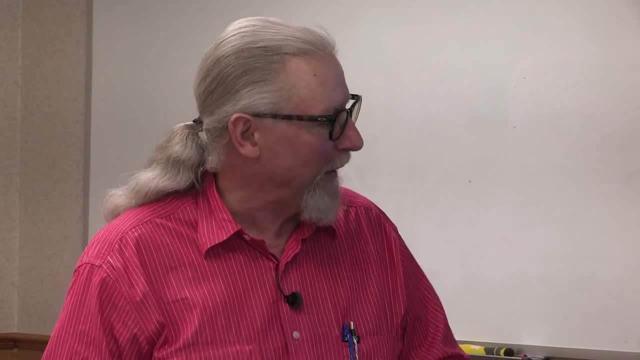 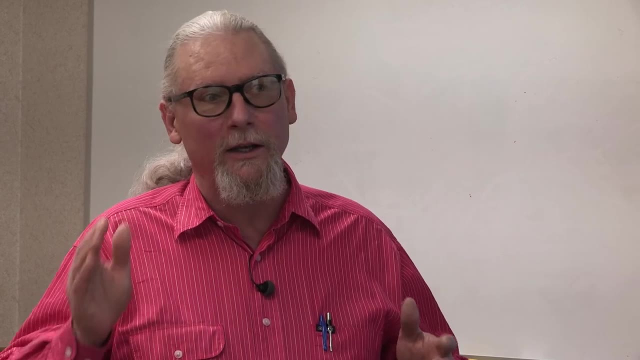 slowly over time and you can have that creep motion. And then the other thing is bedrock. I said bedrock doesn't care whether it's frozen or not, and that's true from the standpoint of settlement. But if you cut into it and you've 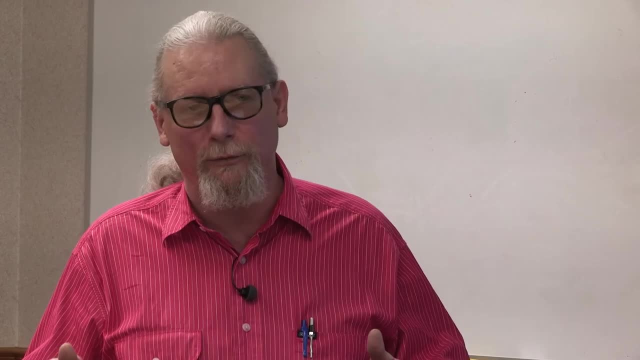 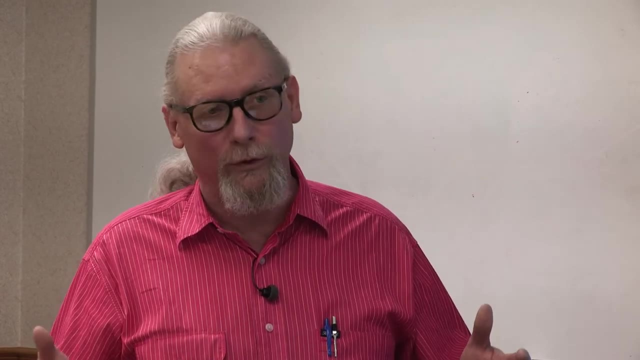 got a steep slope and the bedrock is crummy, it's broken, fractured or it's highly weathered and it's got moisture in it that's frozen and that's what's holding it together. Well, if what's holding it together? 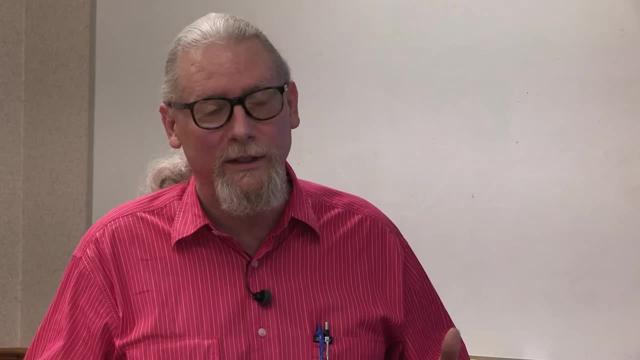 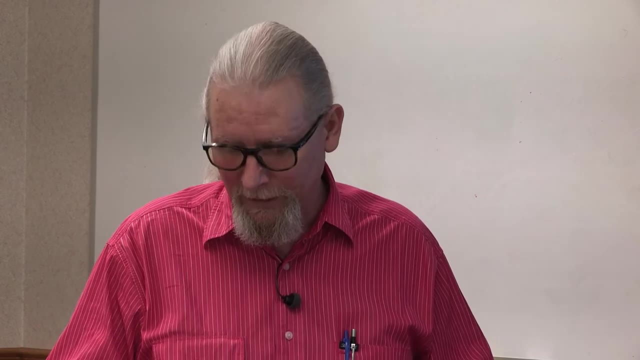 is the ice binding it and it thaws. well, now you've got nothing holding it together, and that is a big element of what's happening on the Denali Park Road in the pretty rock slide. So what does DOT do about it? when we need to build on permafrost, First thing we do. 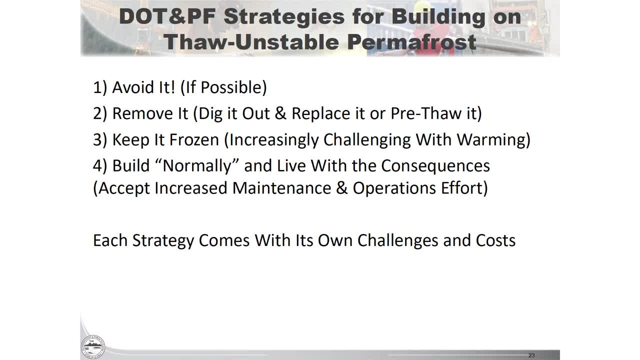 if we can, is we try to avoid it. That's a great strategy, but it's frequently not possible. We can try to remove it. a couple ways of removing it. We've spent a lot of effort and time and have been pretty effective at keeping it frozen. 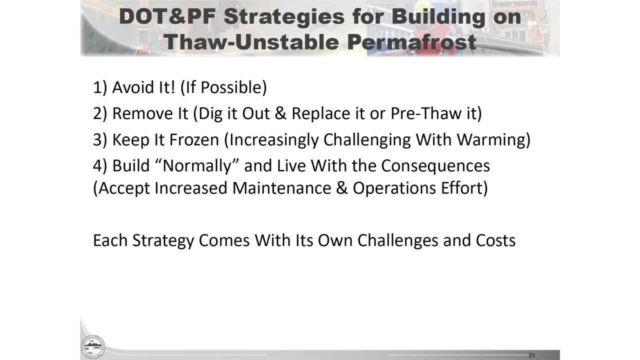 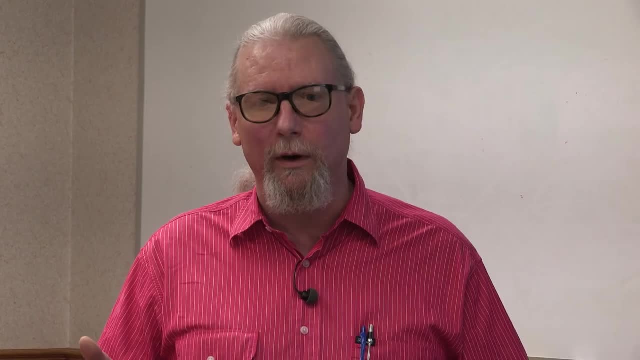 But that's becoming harder and harder because, as we'll discuss, it really is contingent on temperature. And the last technique we use- and this may sound stupid, but it's actually a really good strategy for some facilities some of the time- is just build the road the way you would build it anywhere else. and live with the consequences and accept that you're going to have to do stuff with it. That's basically how the Dalton Highway was built, and it has performed its function pretty well for a long time. Every strategy has its own challenges and has its own costs. Some of the problems with these different strategies, or the challenges with these strategies, is that we don't build a lot of new roads. We do occasionally, but most of the roads we have that we work on, we're trying to maintain the roads we've got. 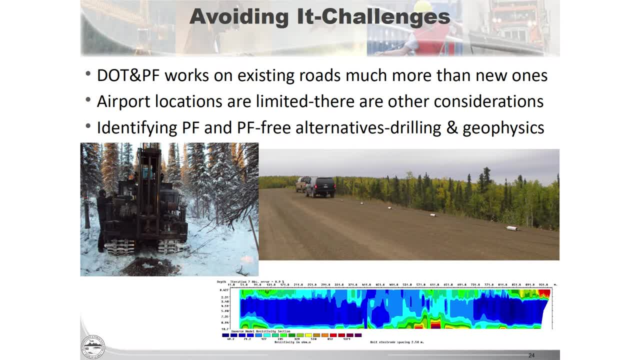 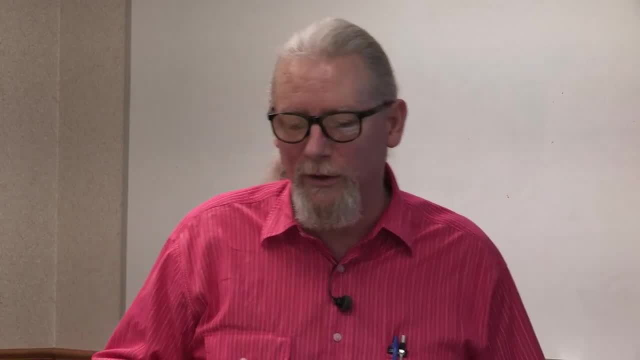 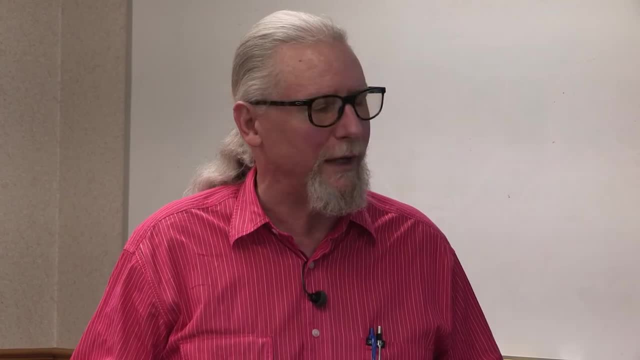 And some of the things we sometimes try to do is improve the geometry. We try to flatten some of the hills or flatten out, widen some of the curves to improve the geometric standards. So you take a road like the Dalton Highway. it was built in the 70s. it's pushing 50 years old now. and where it has been for a long time. yeah, it's been a high-maintenance road, but in a lot of places it's not. In a lot of places it's starting to. the maintenance is slowing down in some respects. because it has thawed to the depth where it's not progressing as fast as it did originally. So now you go and move the road over to the side to widen a curve, or you cut the ground down closer to the permafrost. you reset the clock and you start reinitiating those problems Airports: we do occasionally build new airports and we do try as much as we can to put them on the best foundations we can, but there's a lot of constraints on airports. There's airspace constraints so you can't put them in some topography and airports have to be close enough to the village that they're supporting to be practical, and a lot of times where they are there just aren't really good alternatives. 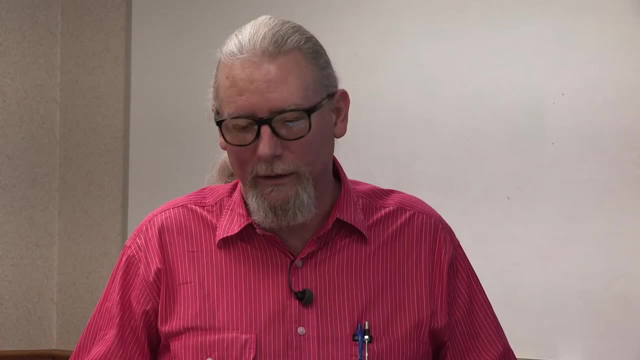 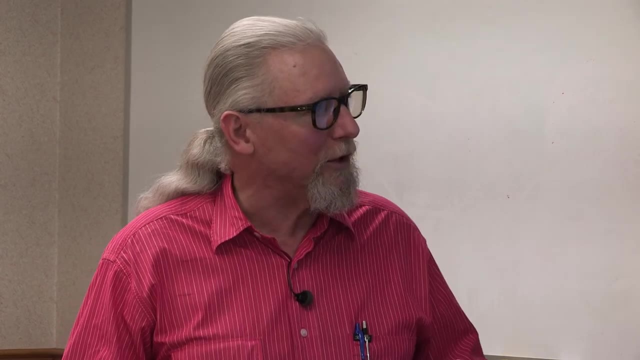 Part of being able to avoid permafrost means you've got to find out where it is and where it isn't, and we're using some new techniques to do that. Traditionally, we use drilling. Drilling is a great way to know what's going on at a given location, at a specific point. 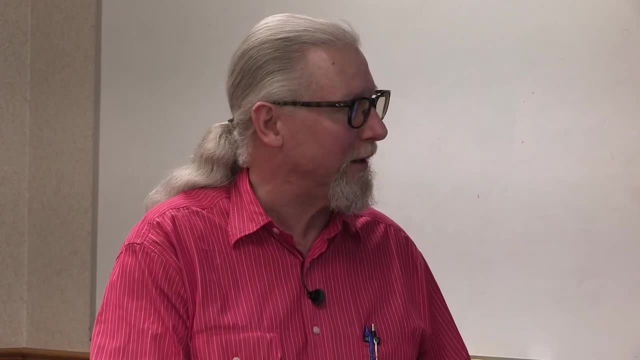 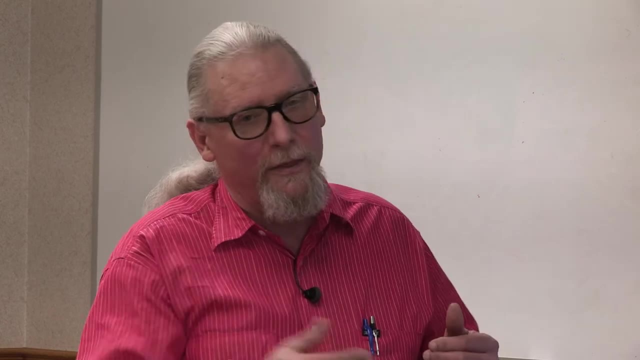 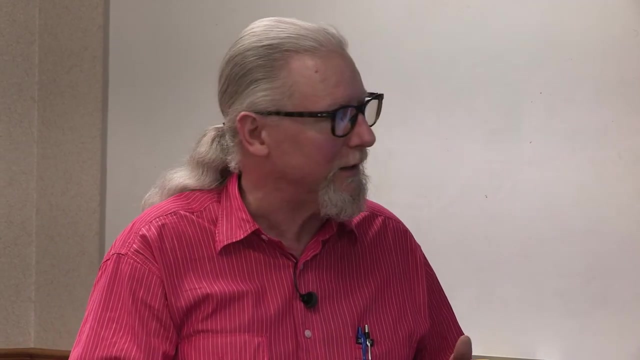 You drill a vertical hole and you know an awful lot about the ground right there, and if that ground is homogeneous and doesn't change between that and the next hole, then that's great. you know an awful lot about the ground there, But with massive ice in particular, and with varying ice contents, 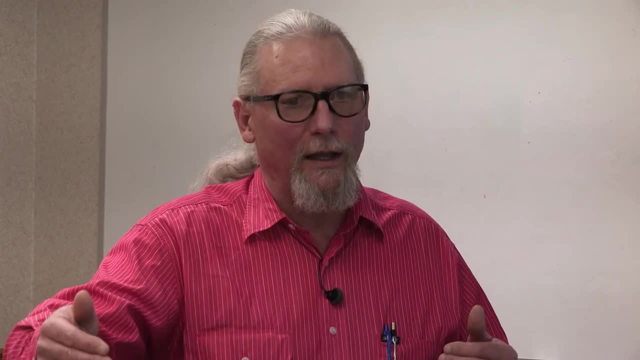 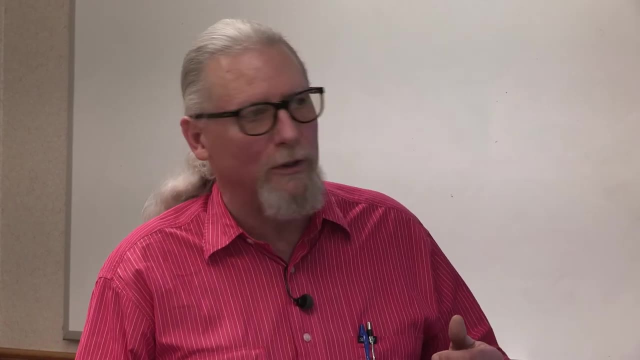 what you might find in one hole. you go 10 feet and it could be an entirely different condition. So what we've been doing lately is using geophysics to help fill in the gaps and also to help us target our drilling more effectively. 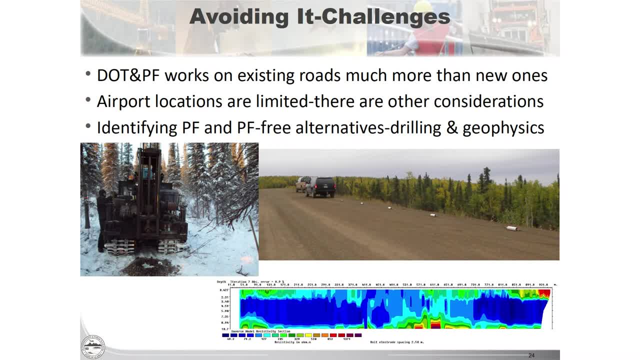 What you see over here on this right. this is a product called OMapper and this is the Coal Regions Research and Engineering Laboratory doing this work for us on the Dalton Highway. This is kind of the output on the bottom. We have recently acquired the same kind of equipment ourselves and we're able to do this ourselves. 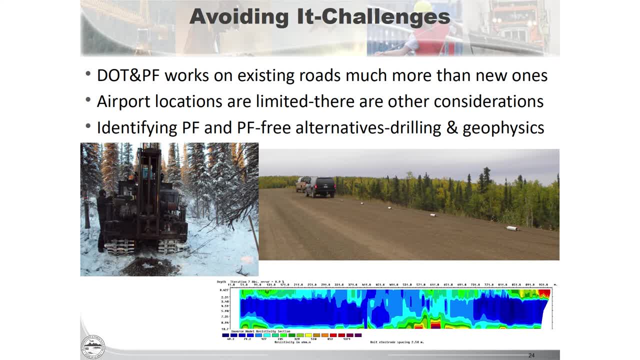 The significant thing here is that ice is highly resistive. this is an electro resistivity method, and ice is very resistive, and so what these hot colors down there represent? in fact they are ice, and ice rich permafrost is pretty high resistivity. 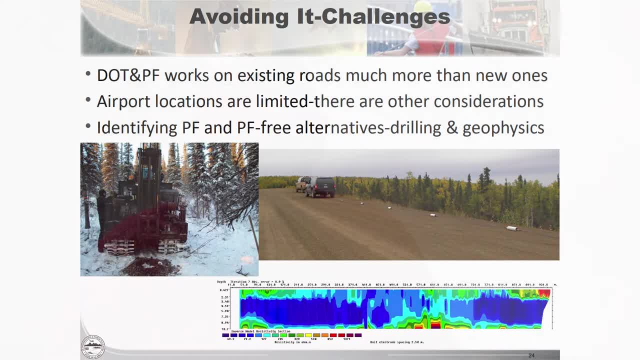 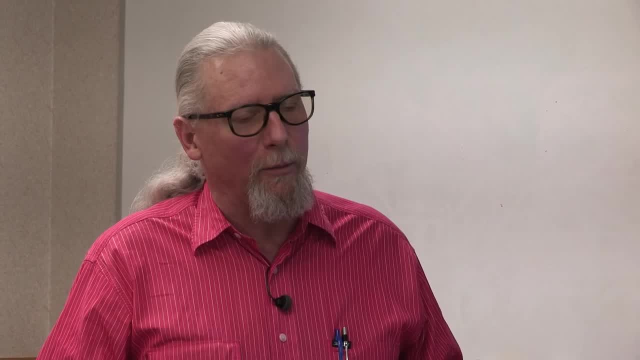 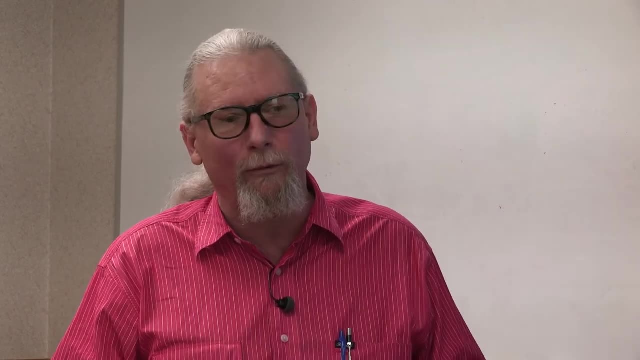 and then other materials have different properties. One of our strategies is to remove permafrost, and if the ground, if the bad permafrost is really bad but it's really shallow and there's something thaw stable underneath it- bedrock or gravel or even permafrost- that just isn't nearly as ice rich. removing the really bad stuff and replacing it can be a good strategy, but it's got its own challenges. You've got this ice rich stuff that you've got to get rid of, and you need to do it in the winter time, because if you do it in the summer time it just turns into a big sloppy mess. so you need to do it in the winter time. then you've got to replace that with thaw, stable fill gravel or something which you don't really want to do in the winter time, but you want to fill the hole back up before it starts thawing out. so you kind of have to. It becomes a fairly expensive proposition because there's a lot of excavation, then there's a lot of material you've got to bring back. It's really whether it's viable or not really depends on the thickness of the bad permafrost. 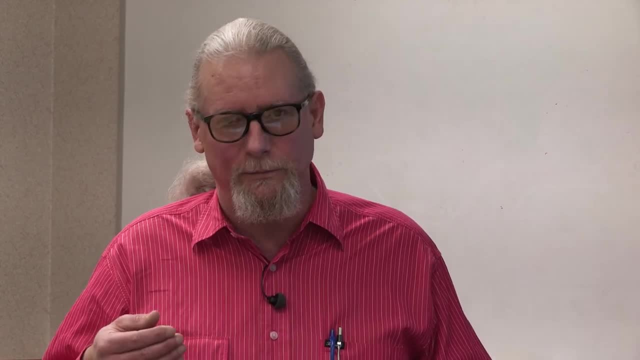 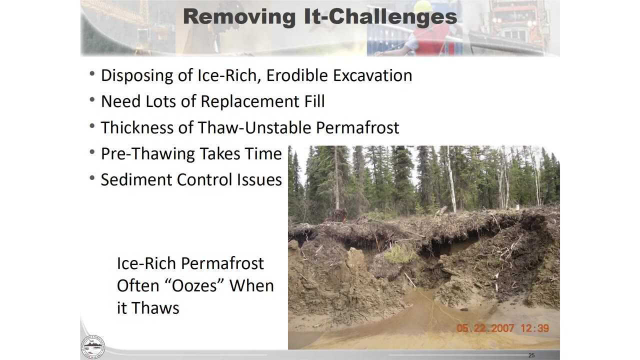 the unstable ice, rich permafrost, the availability of thaw, stable fill to backfill it and a place basically to put that stuff. Another strategy that we have not used very much but that we actually are working on a research project with Transport Canada. 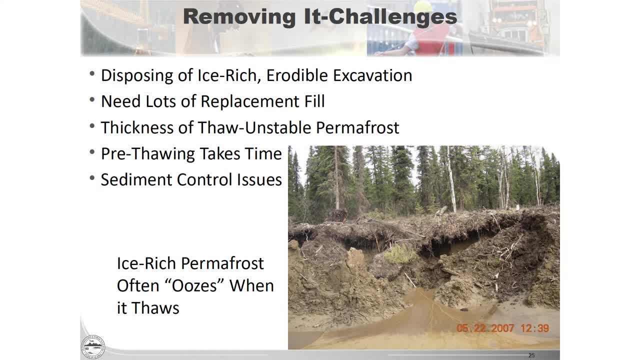 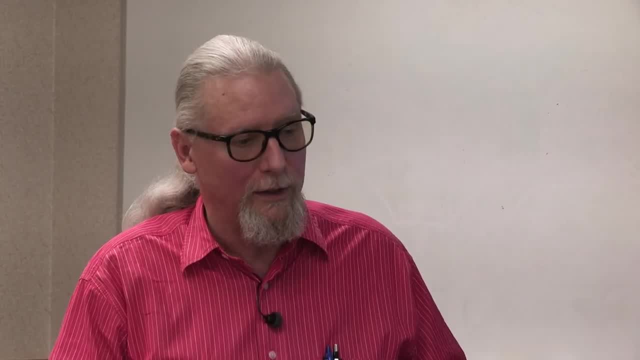 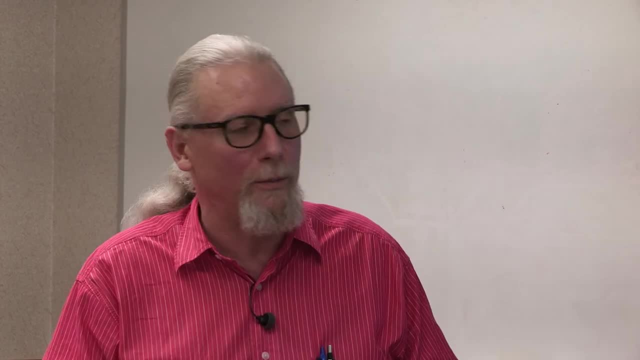 and the University of Laval is the idea of pre-thawing, where you deliberately thaw the permafrost in advance of a project, let it thaw out, probably surcharge it to try to squeeze out that extra moisture and basically prepare the ground before you build a road or a facility there. 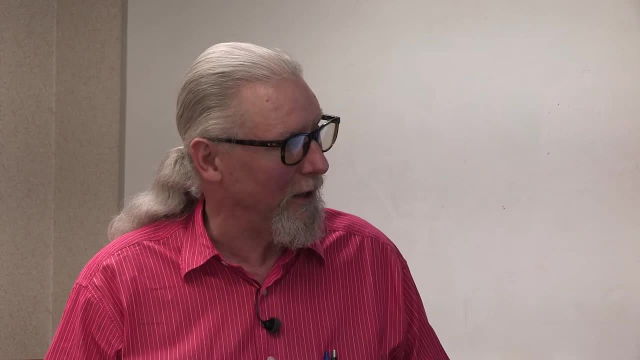 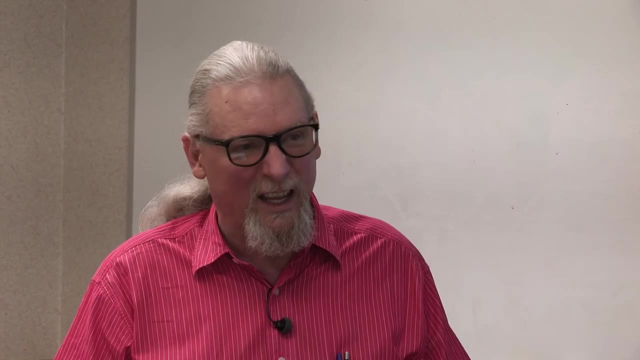 Like I say, it's something we're looking at. it's got its own challenges. Number one is the sediment control. Frequently when ice rich permafrost thaws, it oozes, it makes a sloppy mess and there are sediment control issues. 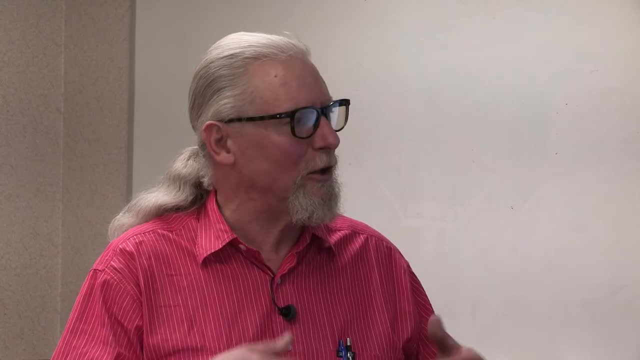 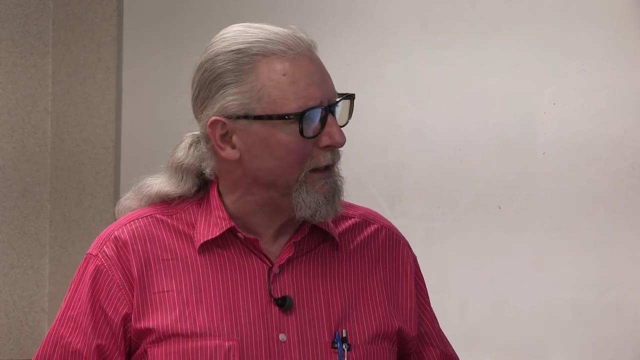 And the other thing is the construction sequence timing. It takes a long time for this to happen. we're talking years perhaps. unless you actively, if you do natural thawing, it takes years for this to take place and our highway construction sequence. 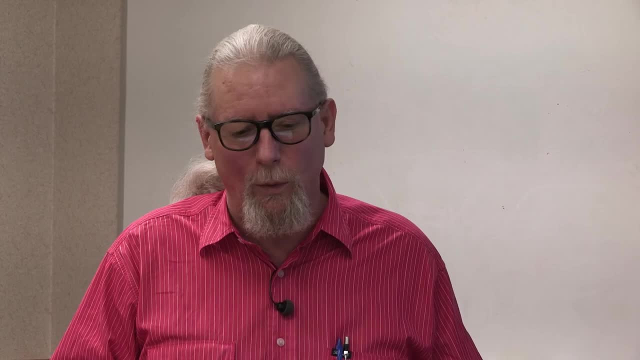 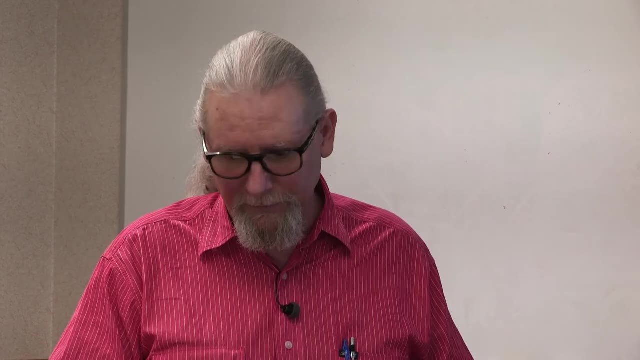 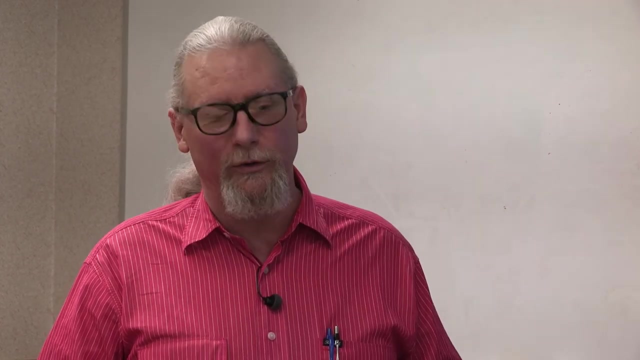 doesn't lend itself very well to working on something for a little while, forgetting about it for ten years and then coming back and building something later. So another strategy that we have used with pretty good success is the keep it frozen strategy. 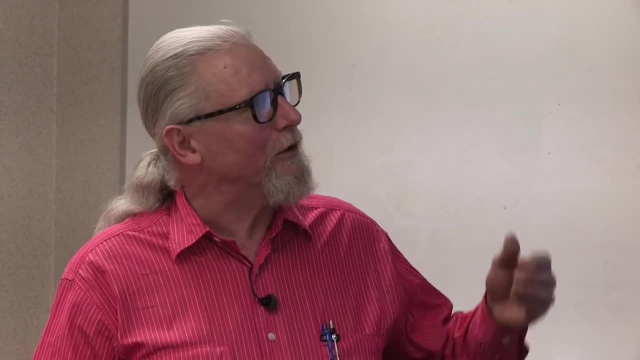 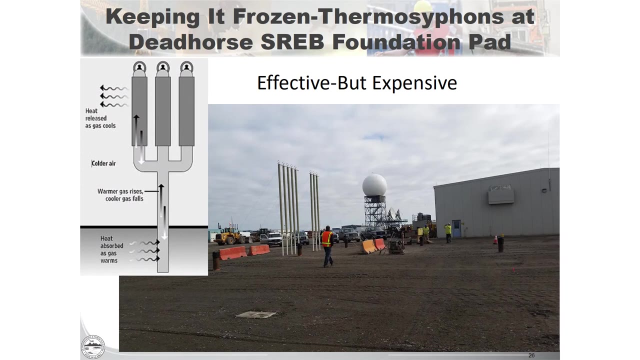 And one of the coolest things- this is brilliant- is a thermosiphon, and we use these routinely for building foundations, particularly on the north slope. that's where this is in Deadhorse. the way these work is: essentially you've got a pipe in the ground. 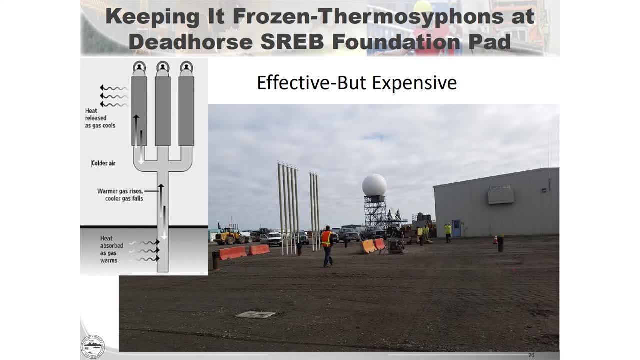 it's filled with a compressed working fluid, ammonia, carbon dioxide. in the winter time that permafrost, cold as it is, it's relatively warm compared to the air temperature. maybe the permafrost on the north slope is 25 above. 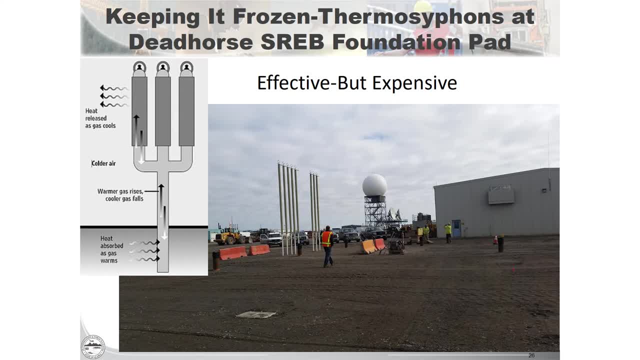 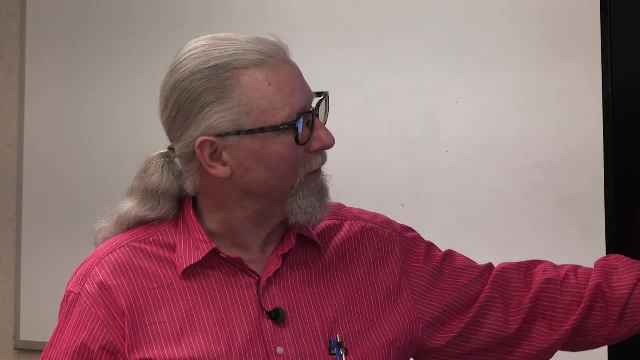 maybe the air temperature is 25 below, So in the winter time the relatively warm permafrost boils this compressed liquefied working fluid into a vapor. vapors are light, so they go up this tube, up the pipe. 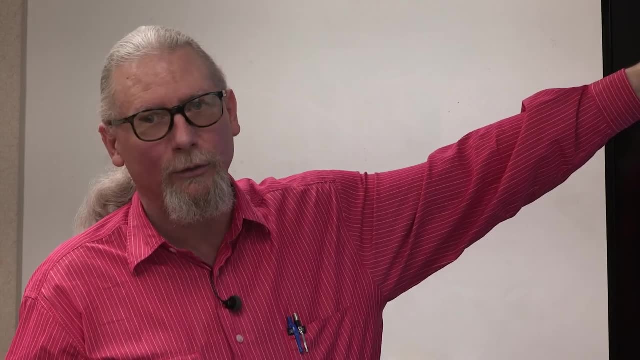 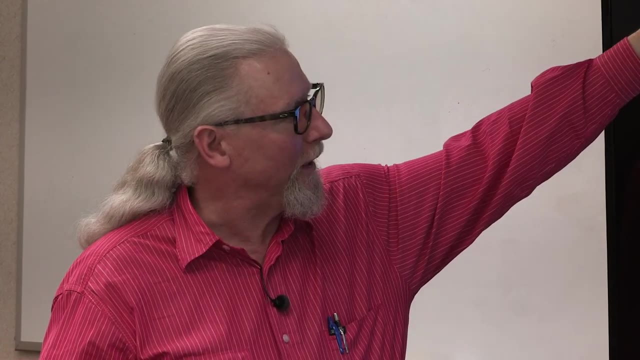 into this condenser. the condenser is colder because it's up in the natural air at 25 below or whatever it is. sheds that heat to the air, cools the vapor into a liquid, condensing it. liquids are heavy. 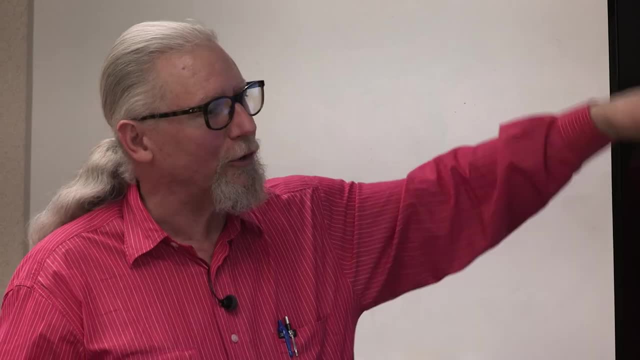 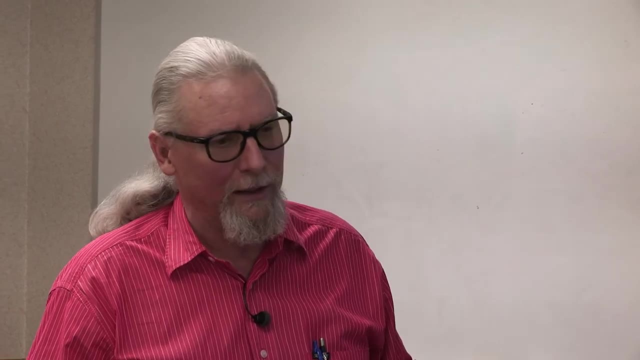 so they sink back down here and you get this internal cycle that is working on gravity and phase change and it's super effective at extracting heat. The Trans-Alaska pipeline has thousands of these things in the vertical support members that hold the pipeline up off the ground. when it goes over permafrost They're very effective. they're expensive and so we use them on buildings which have a high cost per square foot, high unit cost. You can't use them on airports because you don't want planes crashing into them. and they're kind of squirrelly on highways too, because they're in the clear air, they're in the clear zone and there's maintenance issues associated with snow plowing and things like that, but they do work. A similar concept that we've been using. 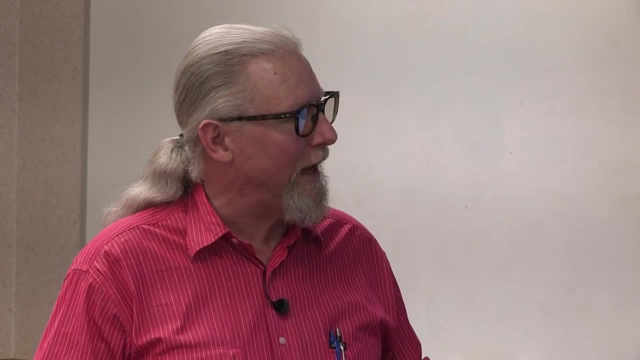 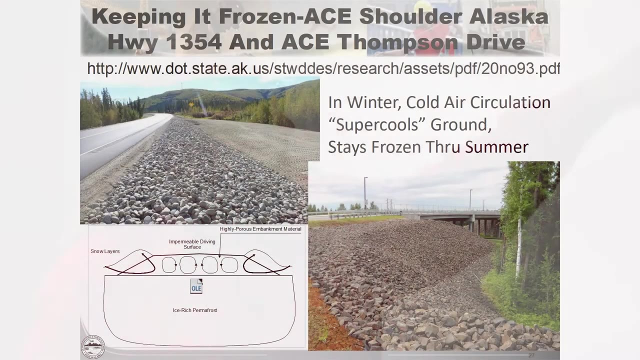 with pretty good effect is the idea of an ACE embankment or an ACE ventilated shoulder treatment, and I bring your attention to this web link here. that is the brand new newsletter. it's brand new in June, by the way, not in August. 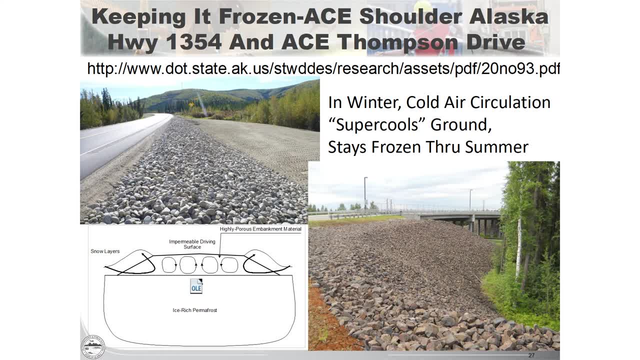 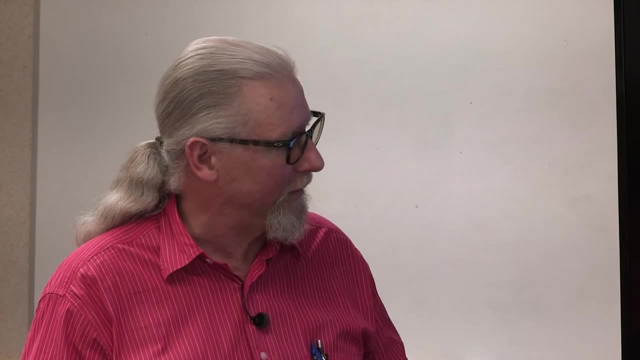 for the DOT and PF's Research in T2 newsletter. it's got a great article on how these systems work and the research that we've been working on trying to optimize them and make them more cost effective. The takeaway is in a true ACE embankment. 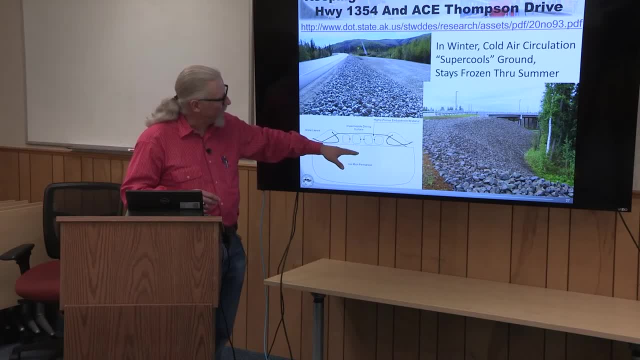 you've got this area. you're trying to keep cold permafrost, maybe warm permafrost. in Fairbanks you've got this driving surface pavement on top that you try to make as thin as possible, So in the winter time 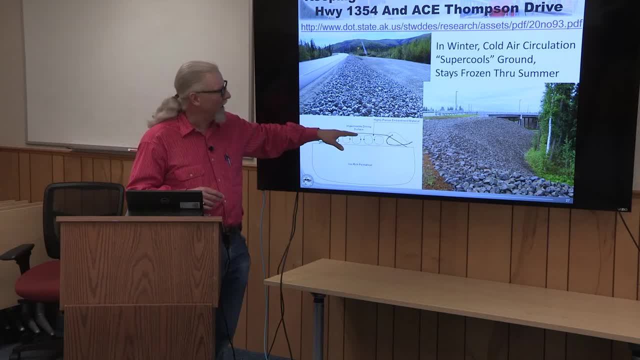 this pavement surface. you're plowing the snow off of it. it's exposed to the air. this gets pretty doggone cold. it gets pretty close to air temperature at the top, and so maybe this the air at the very top of this permeable rock. 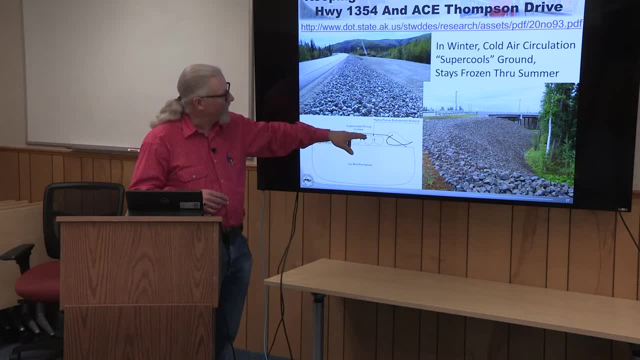 this coarse permeable rock is, say, 10 below zero. Down here the ground is 31 degrees right Because it's warm permafrost. So relatively speaking, this air down here is warmer than the air on top. 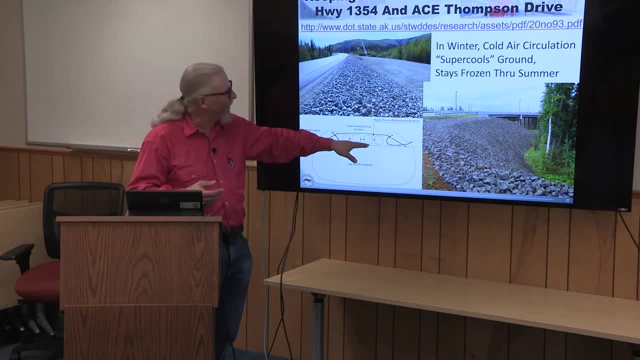 Well, warm air is lighter than cold air, so this warm air on the bottom tries to climb up through this porous rock to this ground surface, where it cools off. Now it's cold air, so it sinks back down and we get these convection cells. 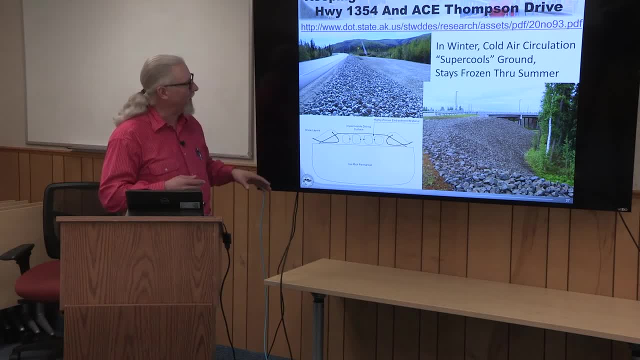 within the embankment, and so you get a net cooling effect in the winter time, And then in the summer time the warm air is on top, the cold air is on the bottom. nothing really happens, except that this rock makes a pretty good insulator. 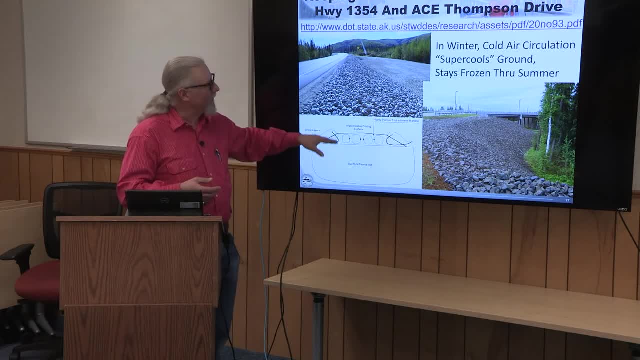 a better insulator than a gravel embankment. and so, year over year, just like the thermosiphons, there's no phase change taking place here, it's just air as a working medium, but you're extracting heat, The other technique here. 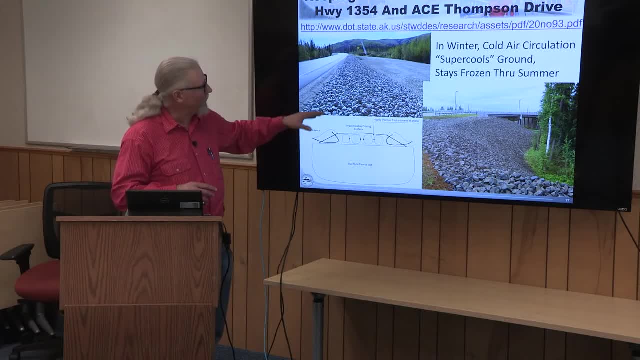 the other strategy is these ACE shoulders, these ventilated shoulders, and in those cases, all you're doing is building a regular embankment, maybe with some insulation in it, and then putting this rock treatment, this porous rock treatment, on the shoulders. 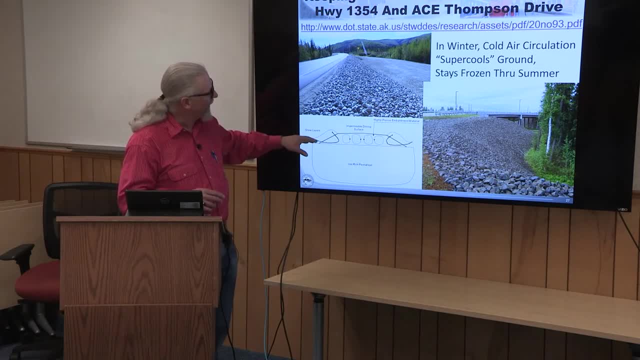 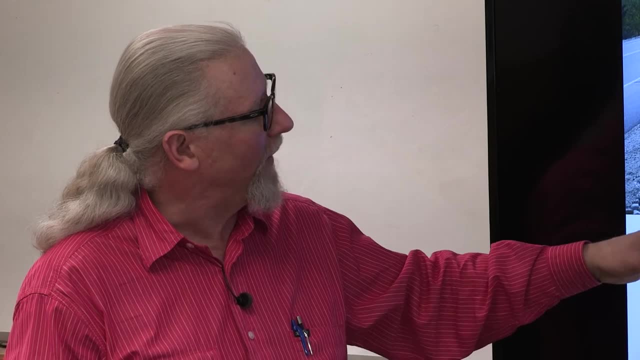 so that in the winter time cold air can penetrate that rock and the relatively warm embankment compared to the air temperature warms it and you get this chimney effect that promotes circulation and extracts heat, and this is actually quite effective. 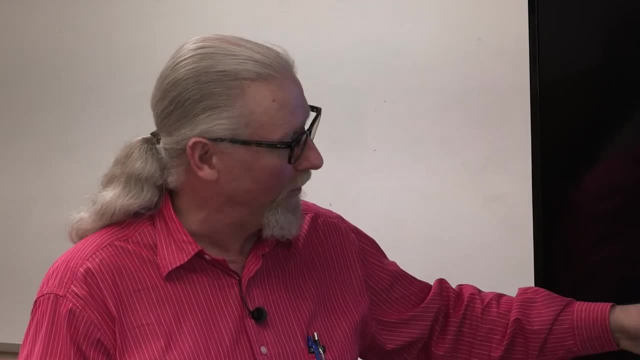 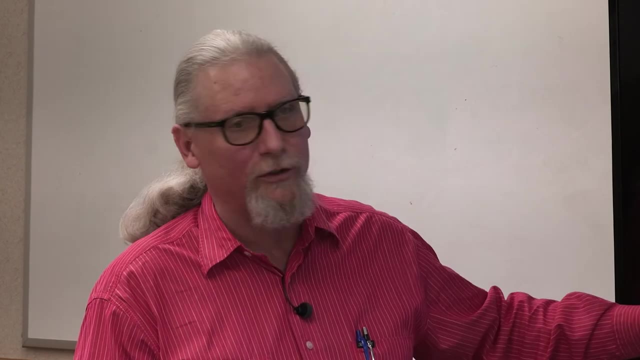 and super cools the toe of the embankment, which ultimately helps freeze back everything. Remember, the toe is the part that tends to thaw the most in the summer time, so this is a way of freezing it back more in the winter time. 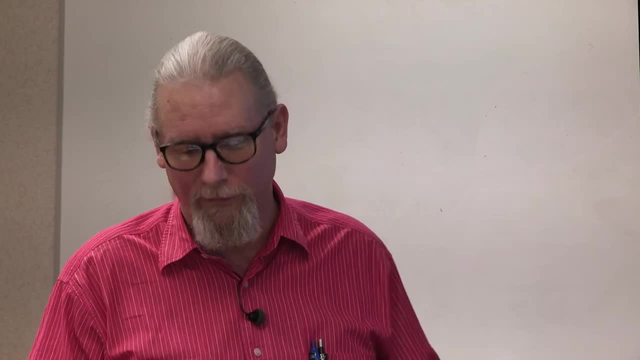 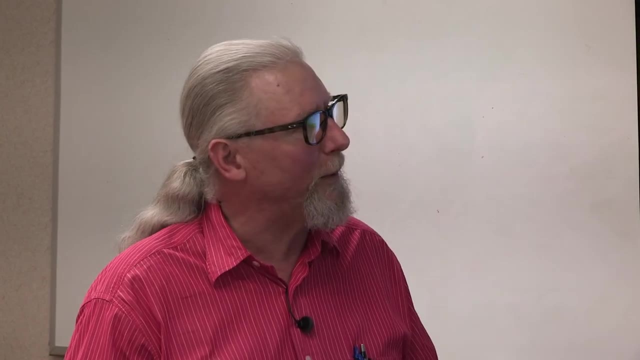 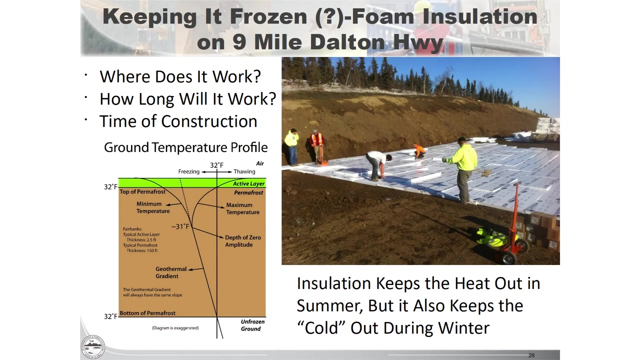 and we have research that is showing that this is very effective. Another technique to keep it frozen, maybe, is using foam insulation. Foam insulation is not magic and it doesn't make things cold. it retards heat transfer and it's just like an ice chest. 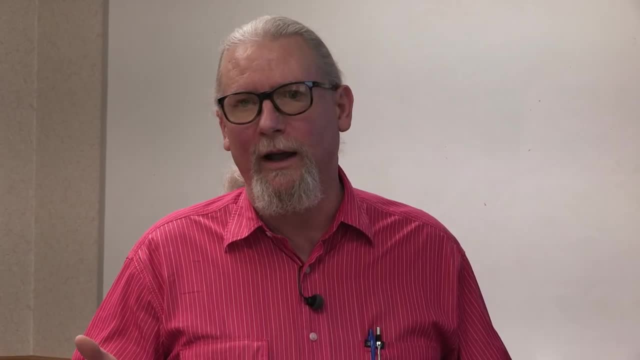 If you had two growlers of beer and you put one in an ice chest and you put one in a milk crate and you threw them in the back of your truck in the summer time, which one is going to heat up first? One in the milk crate right, Because the insulation of that cooler keeps that beer colder longer. But now you do the same exact thing in the winter time and you want to get home from the brewery before anything freezes. which one is going to freeze first? Well, the one in the milk crate is going to freeze too, because that cooler is keeping the heat that's in the beer from extending into the outside air temperature. In the beer case the cooler works both ways, But in permafrost 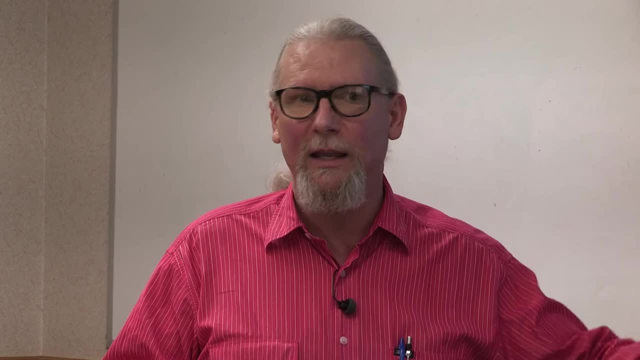 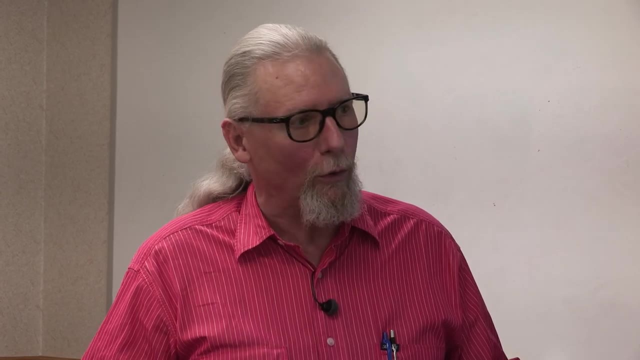 what we really want to do is to make it cold in the winter time and keep the heat out of it in the summer time. And insulation. it's a double-edged sword. it works both ways Up on the north slope, where things are cold. 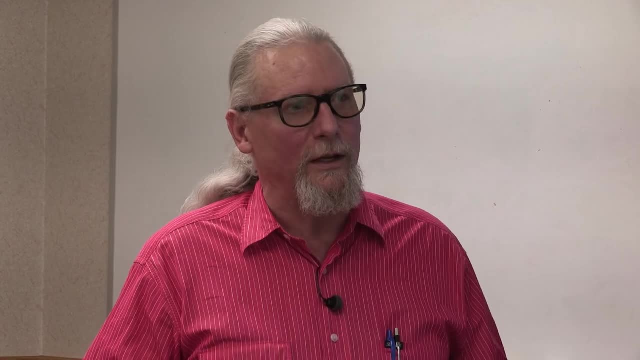 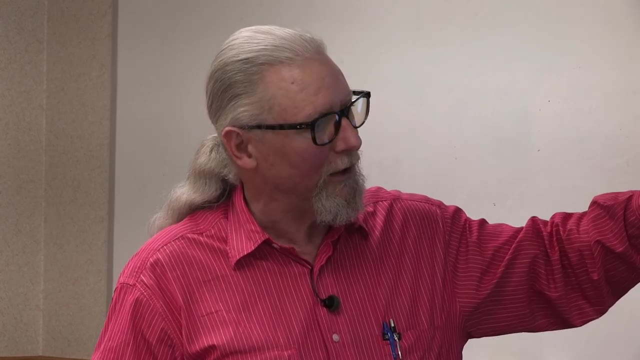 insulation still works. It works pretty well because the winter is long enough and cold enough to freeze more than it thaws in the summer time, and so what that insulation does is just keeps that depth of thaw out of the ground in the winter time. 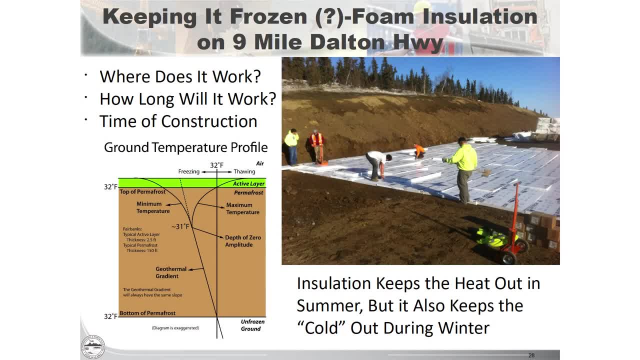 in the summer time. In the interior, on the other hand, where things are thaw and stable or perhaps degrading- already- I mean 2019,- we were above freezing right In Fairbanks. What this does is it slows the rate of thaw. 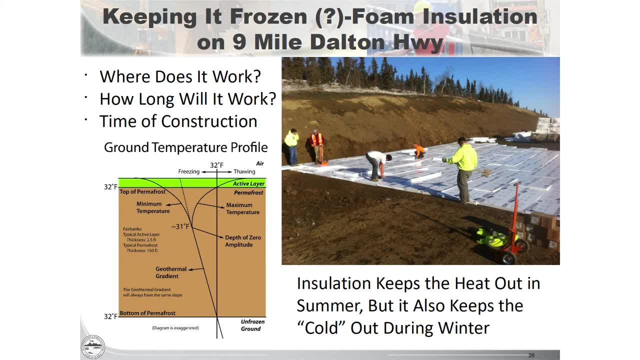 but it also kind of prolongs the misery. So you're experiencing that longer time and again. I've got another diagram of the trumpet curve. As you can imagine, as this trumpet curve moves to the right, this is going to continue to work less and less. 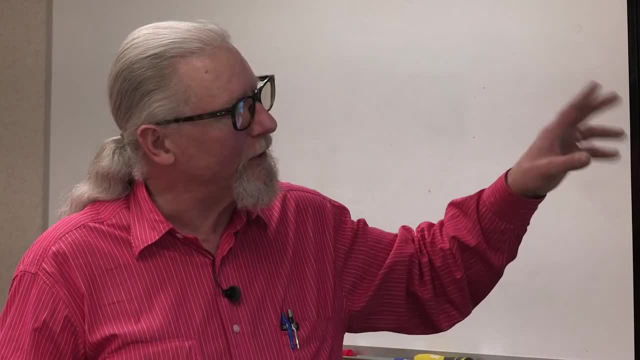 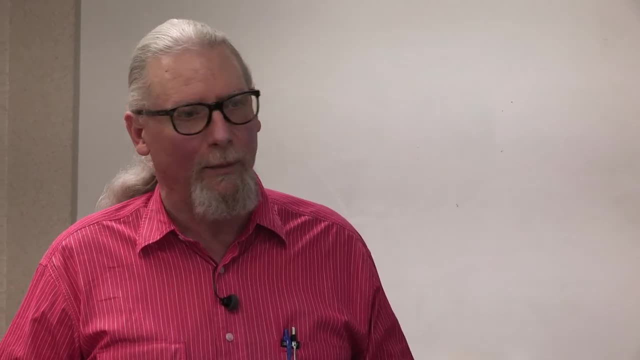 and the time of construction is really critical. with insulation, if you're going to use it at all, The ideal time to build is in the spring time. You've got maximum frost penetration from the winter and everything is as cold as it's going to get. So if you excavate quickly, put your insulation down and backfill on top of it quickly, right around break-up ideally, then you're trapping the coldest conditions in the ground. You're over in this area here and so, like I said, 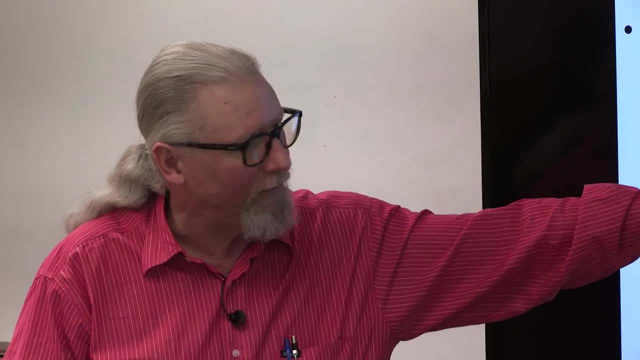 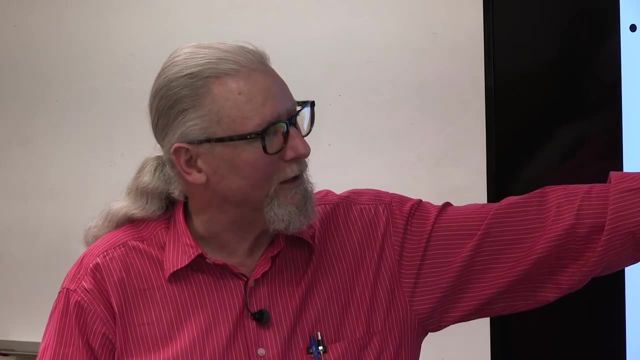 that's the best scenario. A bad scenario is to do it in the fall. Then you're doing the exact opposite: You're trapping, you're trapping in all the summer heating and you're putting insulation on it. so you've sort of shifted that curve to the right. But the worst thing you can do is to excavate in the spring and then walk away, Then come back in the fall and then insulate it, Because then you've done both. Not only have you, you've accelerated all that thaw. 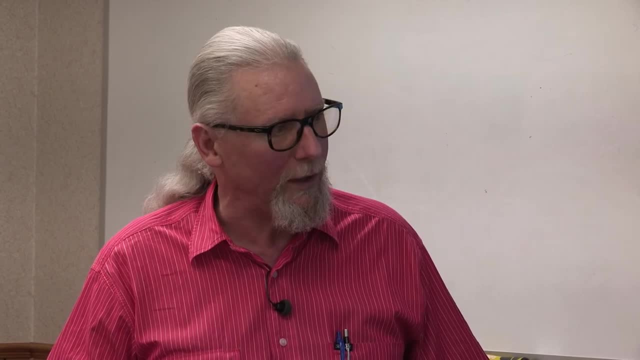 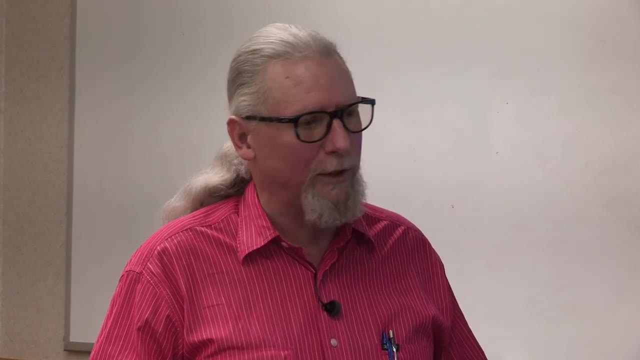 One of the things we do at DOT is thermal modeling. That's how we determine what the stability of an embankment is going to be. It's challenging. We've been doing it for many decades. We used to use a one-dimensional DOS-based program. 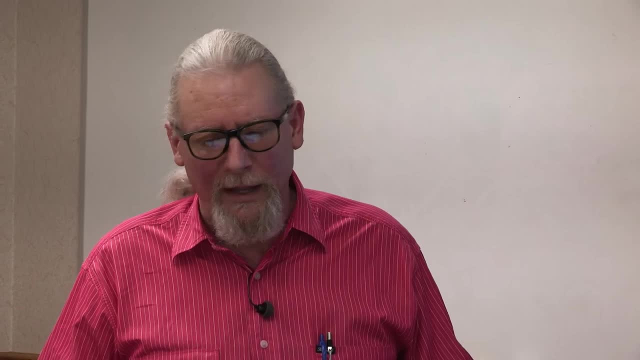 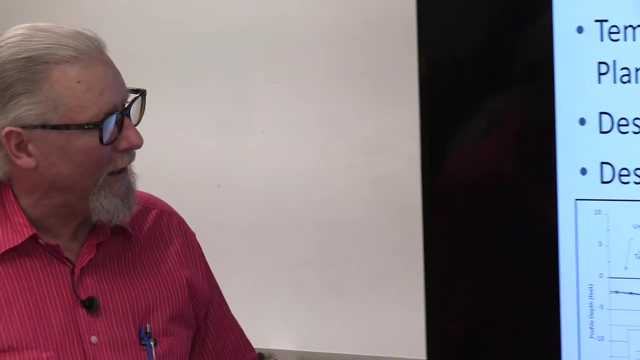 Anybody remember DOS, But it worked actually quite well. but it was a one-dimensional program so it looked at thawing in a vertical manner And that actually works quite well in the middle of an embankment or the center of a runway. 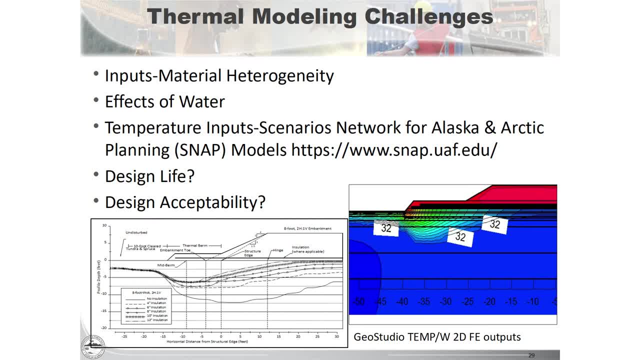 But, as we've seen, the toe of the embankment is really frequently the more critical part, And so we now use a two-dimensional finite element program called TEMP-slash-W that allows us to model temperatures with different scenarios, And it's tricky. 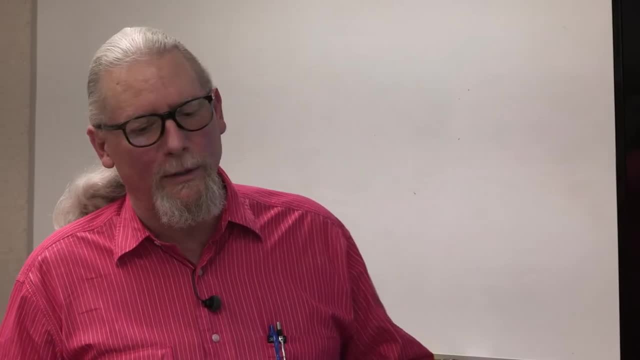 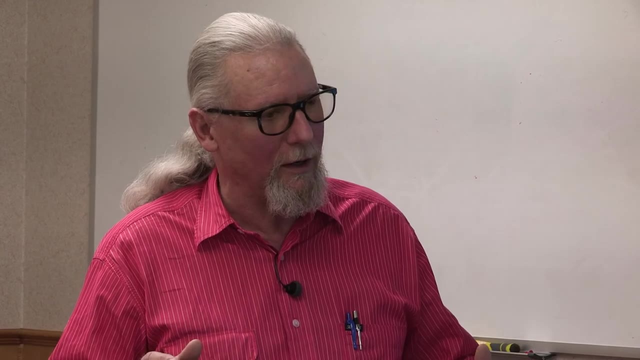 There's a question of what material inputs you should use. And again, if everything is really homogenous and you know exactly what the conditions are, that's great. But frequently, if you've got ice wedges and then ice-rich soil and then ice-poor soil, which one do you model? It's tricky. Modeling for water is very tricky. Water has a high degree of thawing capacity. We do have a research project looking into that too. The temperatures are actually one of the things we have a moderately good control over. 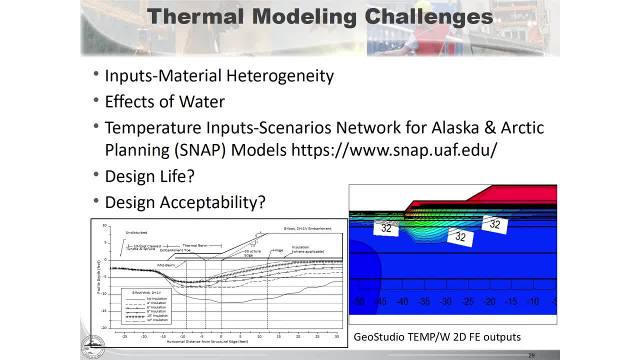 and we have been using the IPCC RCP 8.5 models that we get through SNAP up at the university. That's our current protocol for modeling into the future. We started out using the 6.0, because it was sort of the middle-of-the-road model. 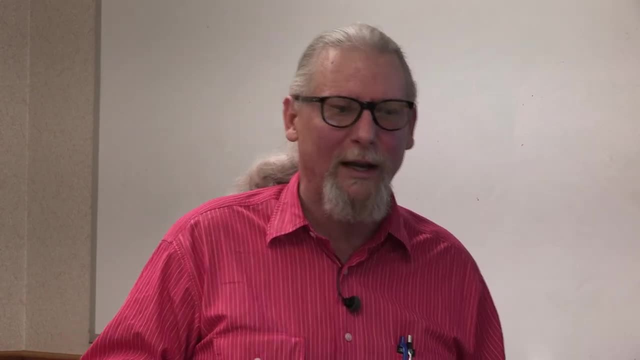 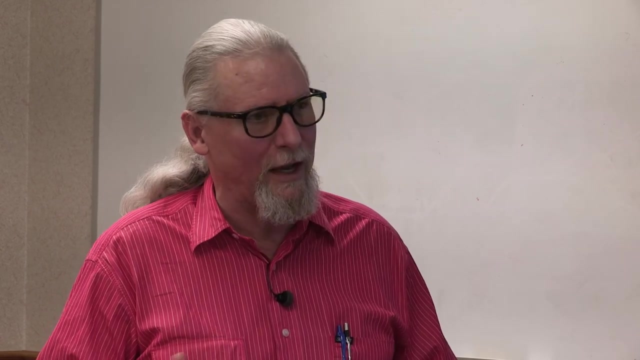 But as it turns out, the 8.5 model actually seems to be tracking pretty well with what we're actually observing in Alaska. There's a couple philosophical questions about thermal modeling too, and design in general, The design life of a project. 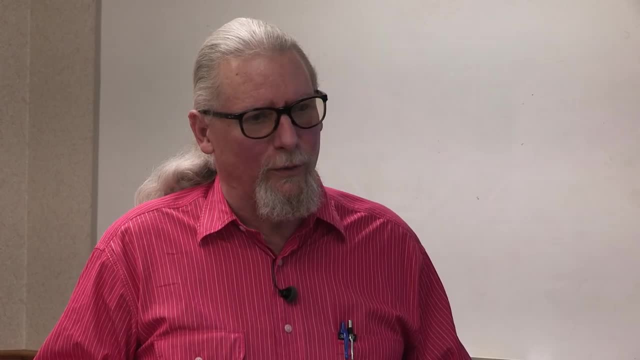 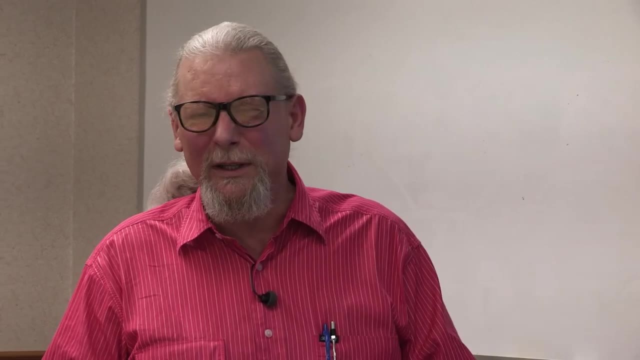 of a piece of infrastructure. that's how you design a project And historically we've used maybe a 30-year design life for roads. But that's really looking at the needs, the capacity needs, whether you need to add another lane. 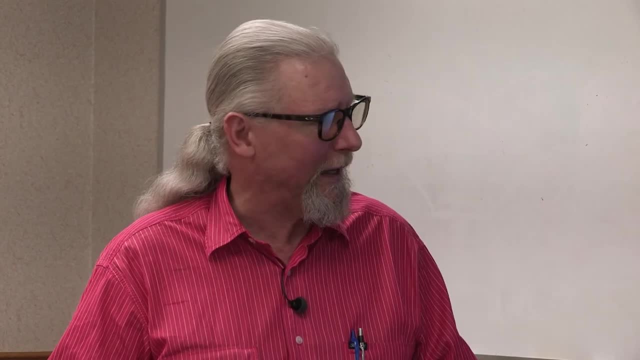 or when you're going to have to rehabilitate the pavement or something like that. It's really not the idea that, well, it's thermally stable for 30 years and then, after that, it's going to start falling apart. and the maintenance requirements are going to go up exponentially. If you were to try to design a road or an airport based on the current RCP 8.5 modeling to be stable in the year, say, 2100, it just wouldn't be cost-feasible to do that. And we don't. But what that design life ought to be. that's sort of a philosophical question and it really comes down more to policy than to engineering. Another question is: what constitutes an acceptable design If it thaws and you get some settlement on the shoulder? 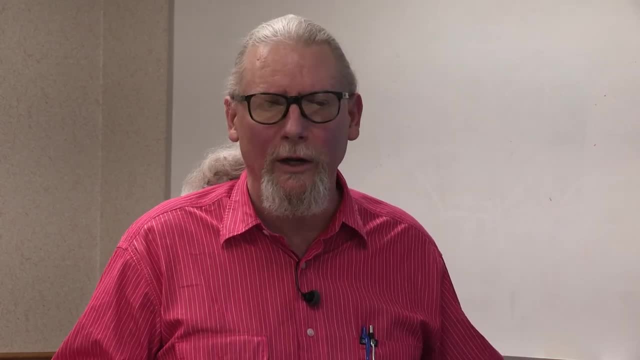 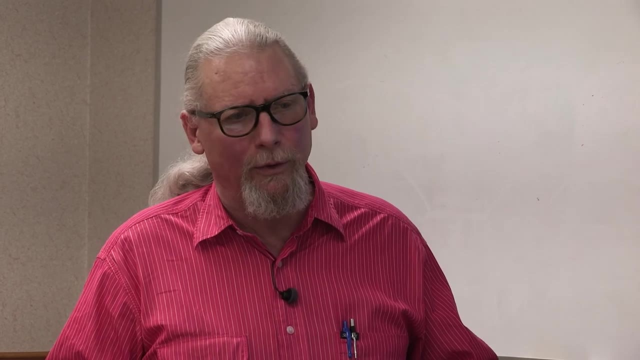 is that okay? Yeah, I think it probably is, at least on those airports where it doesn't affect the operational activity, On a low-volume road, the road to Tanana, for example, or say an air road. well, we can tolerate a fair amount. 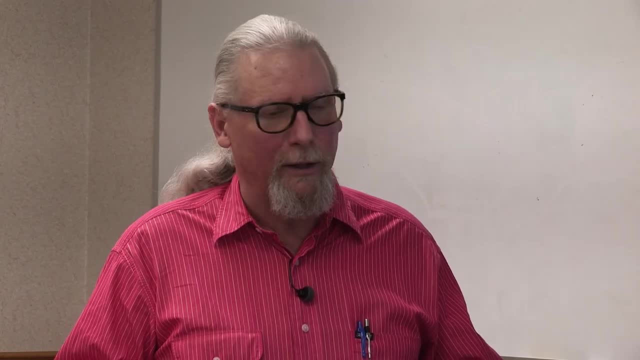 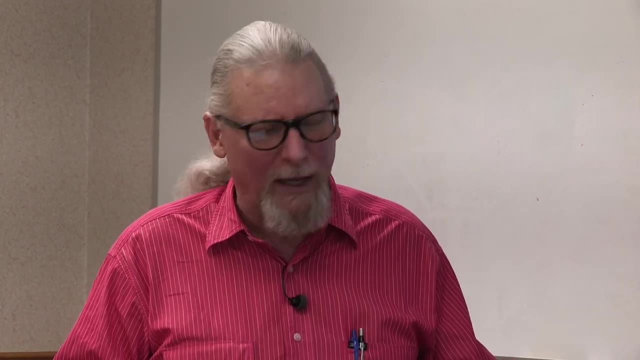 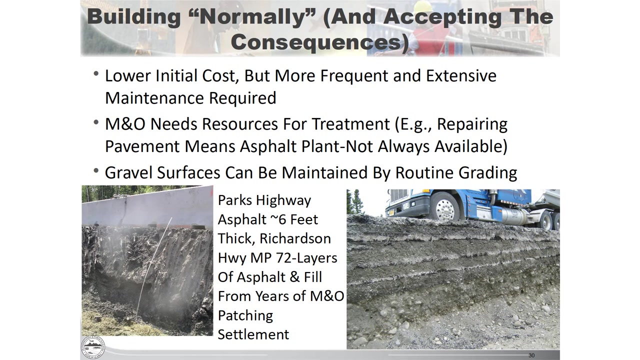 of misbehaving in that road On the Parks Highway, Mitchell Expressway? no, not so much. We don't want settlement there, So it really is. It's an interesting point to debate. Our final strategy is just to build the way we would normally build. 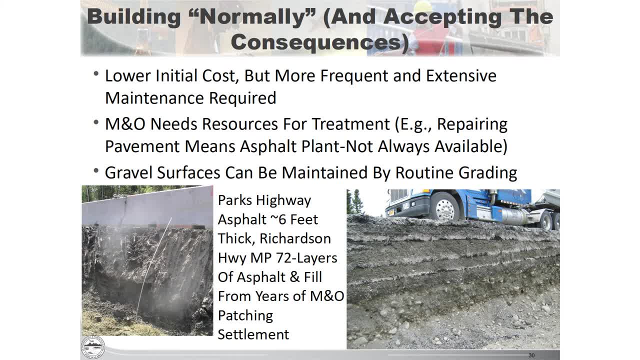 Like I say, it's worked pretty well on the Dalton Highway. It's a cheaper way to build it in the first place usually, but you can anticipate more work required in the future And when you do this you kind of have to consider. 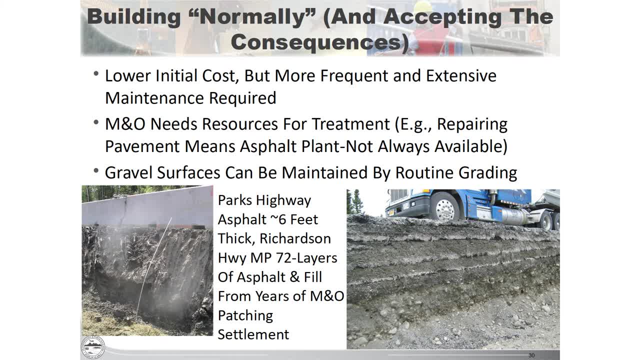 what is M&O going to need to do that? You know, if you've got an asphalt-paved road and it starts falling apart, you've got to fix it with asphalt. Well, that's a problem and maybe that's a good strategy in Fairbanks. 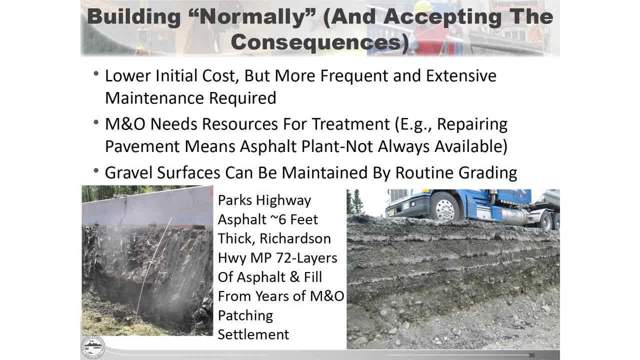 where you've got asphalt plants in the summertime. but up on the Dalton Highway, where you're 400, 500 miles away from the closest asphalt plant, that could be a real challenge. Gravel surfaces: I'm a big fan of gravel roads for a lot of facilities. 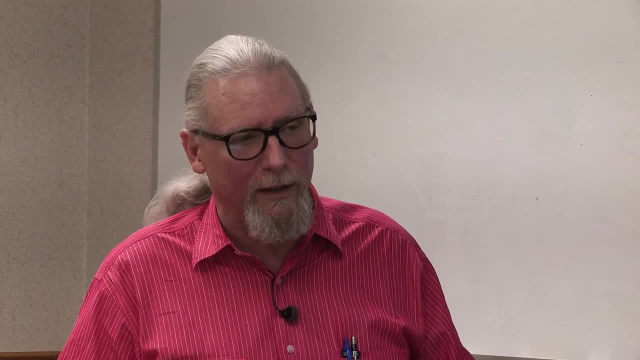 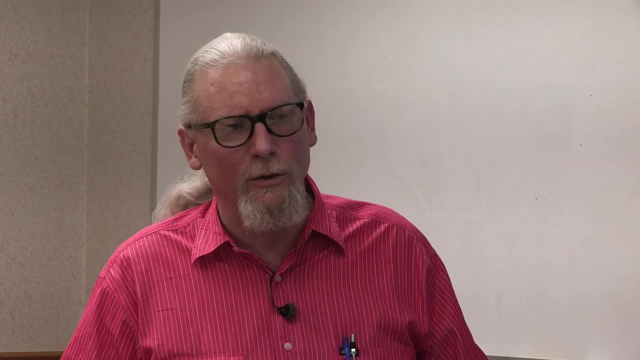 They can be maintained with grating and they may require a fair amount of maintenance, but it's something that is. It's pretty doable, and when something does settle to the point where it needs to be filled in, you can haul in gravel. 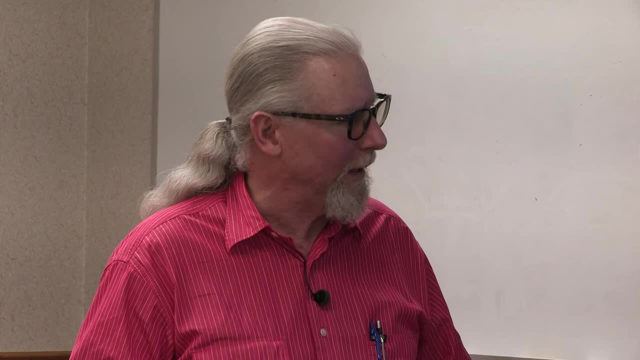 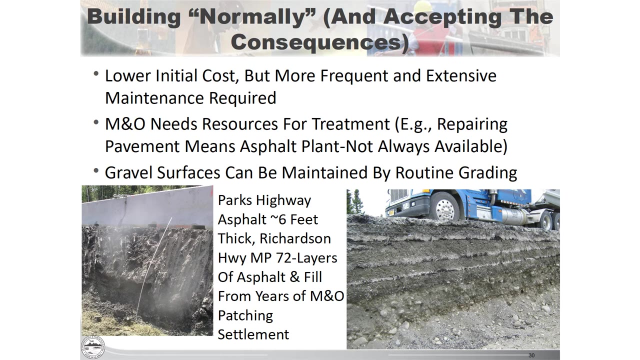 which is something that our maintenance and operations folks do. anyway, I've got a couple interesting pictures here. The one on the left here is a section of the Richardson Highway where there's about six feet of asphalt, where it has settled, M&O has filled it in. 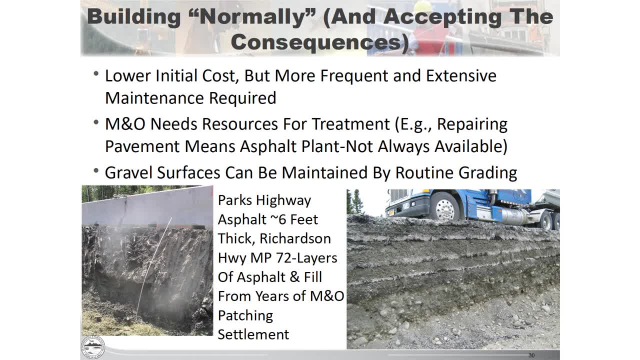 settled and filled it in, probably not uniformly over the years, but it's continuous asphalt. On the right on the other hand- I'm sorry, that's the Parks Highway. On the right, on the other hand, is an area where it probably was not super ice rich. 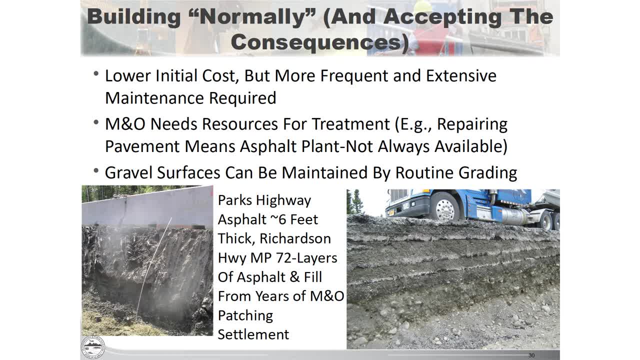 and it probably was pretty uniform and settled uniformly, because we've got this layer of the original embankment and asphalt pavement, another layer of gravel and asphalt, more gravel, another layer of asphalt, another layer of gravel and the current layer of asphalt. 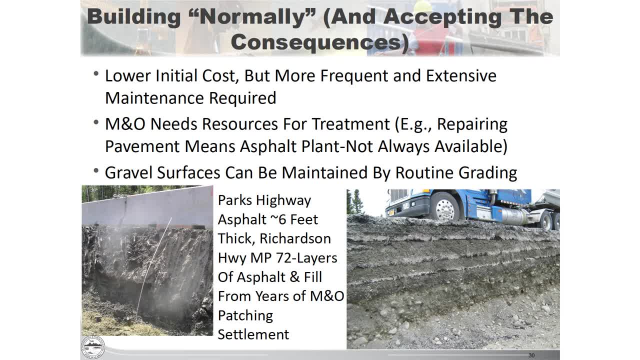 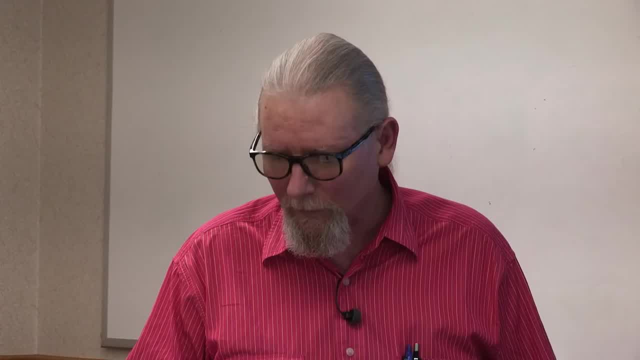 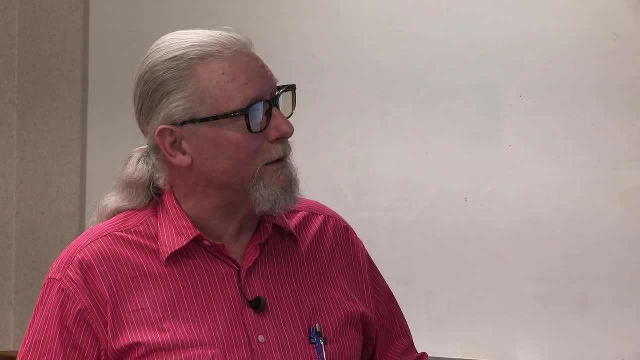 So that's one strategy there, just to keep building it up when it starts getting too low, if everything settles uniformly, which doesn't always happen. Oh, so some final thoughts. It is reasonable to expect that our maintenance is going to increase. 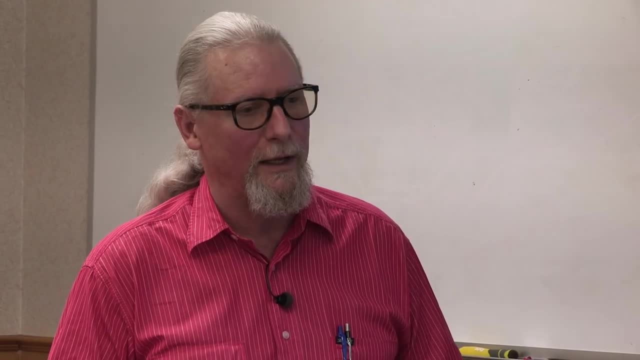 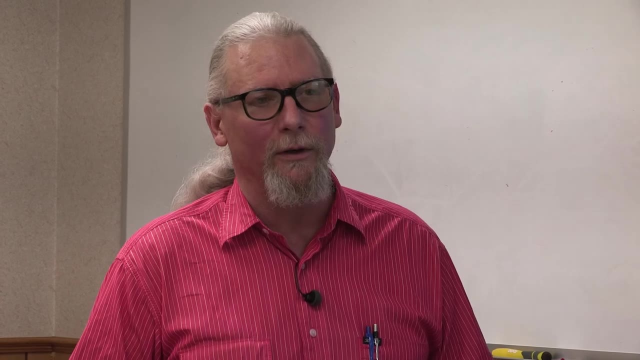 I've talked to a number of our DOT superintendents and they have told me anecdotes, and they've gotten numbers to show it too, that over the last oh, 10 or 15 years, the amount of effort, the frequency of the repairs, 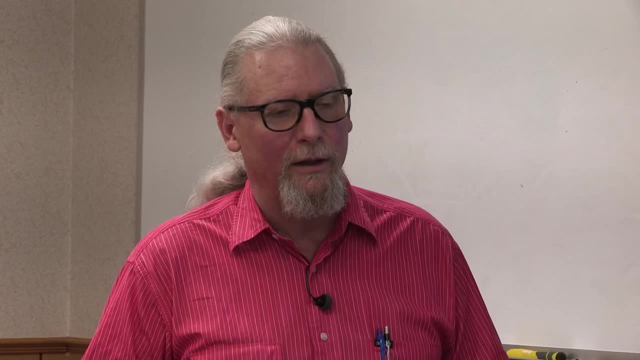 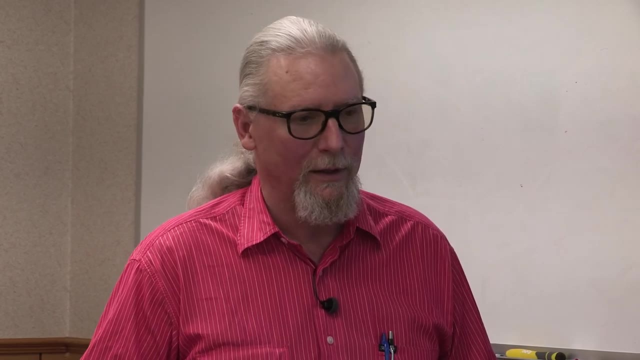 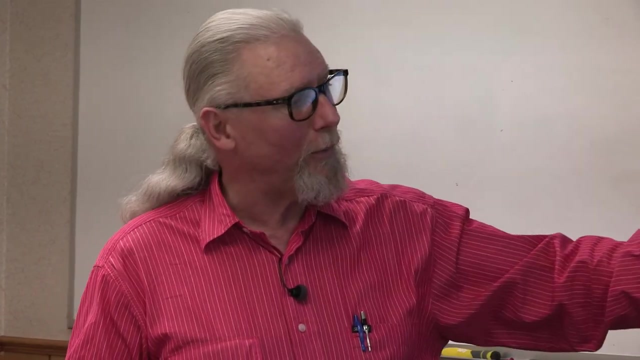 the extent of the repairs has gone up And they attribute this to the warmer temperatures that we've all experienced over the last oh, 10,, 20,, 30 years. I say generally increase. There's going to be some places. where the maintenance actually goes down. If the permafrost thaws and drains and stabilizes in those isolated permafrost areas, things may actually get better. But there's more to go. there's more areas that can get worse than there are areas that are going to get better. 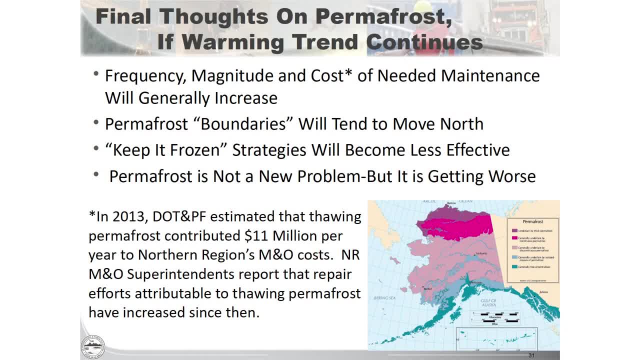 any time soon, These boundaries of where discontinuous permafrost and isolated permafrost are going to tend to move north and the percentages are likely to change, And that discontinuous permafrost, if it's currently, say, 50-50,. 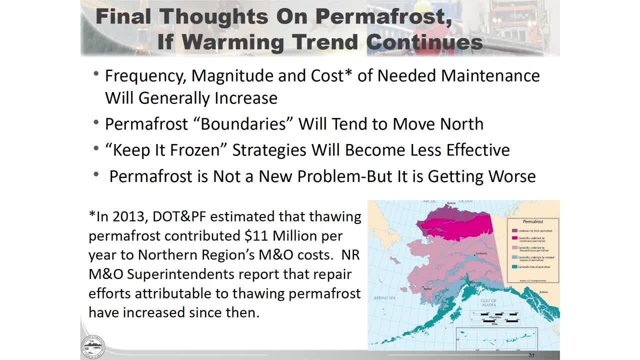 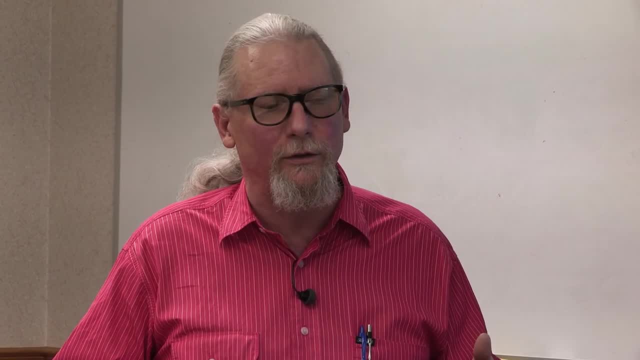 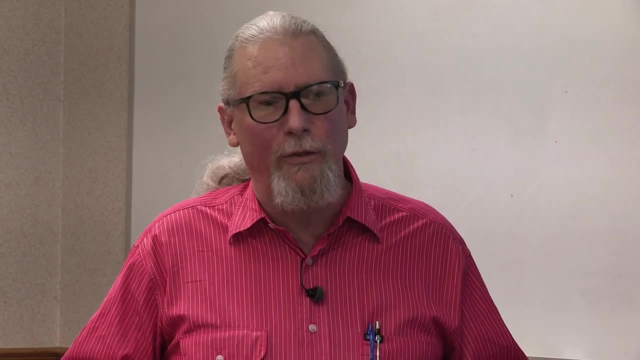 30 percent, 70 percent. those isolated areas are going to tend to dry up and go away. The keep it frozen strategies all rely on winter to freeze things back. The takeaway on all these strategies is: you're counting on enough freezing taking place to drive the thermosiphons. to freeze the ground back or to make the ACE convection cells work or the shoulders work, or even where you're using insulation to hopefully have a net freezing effect, like, say, on the North Slope, And the less winter we have and the more summer we have. 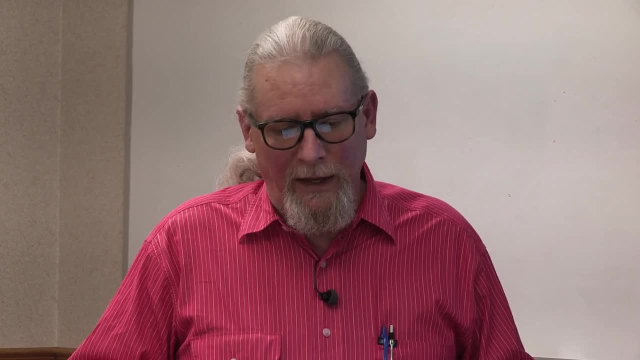 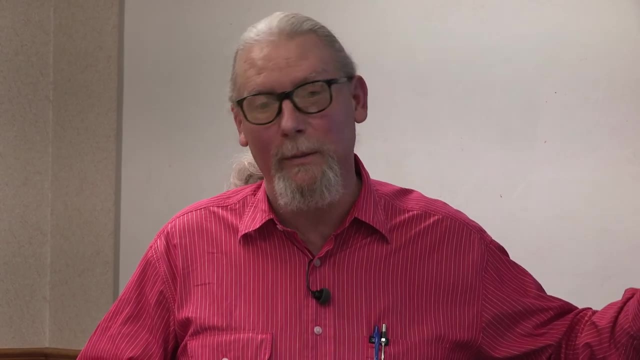 the less effective these techniques are going to be. And the final parting shot is: permafrost is not a new problem. I showed you the picture from 1942 of the Alaska Highway, but it is a problem that's getting worse, Thank you, 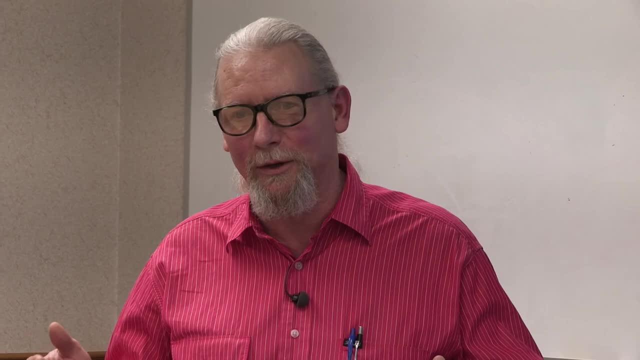 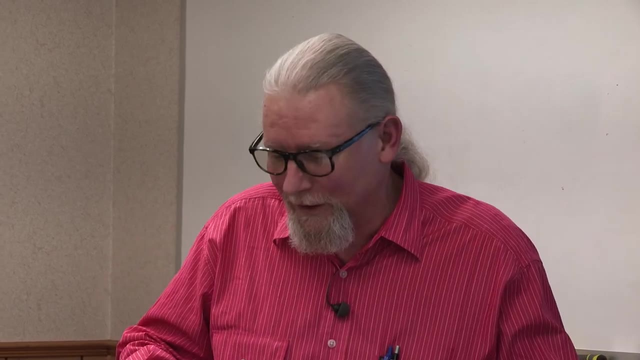 This is the part of the show where normally I would ask for questions and do a little Q&A. You over there, the imaginary person in the chair at the end of the table, what was it? Okay, I'll repeat the question for the audience. 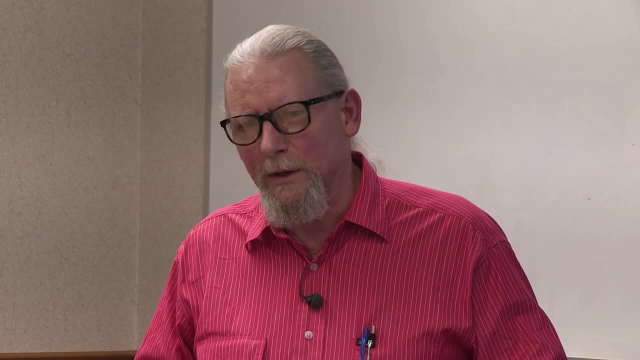 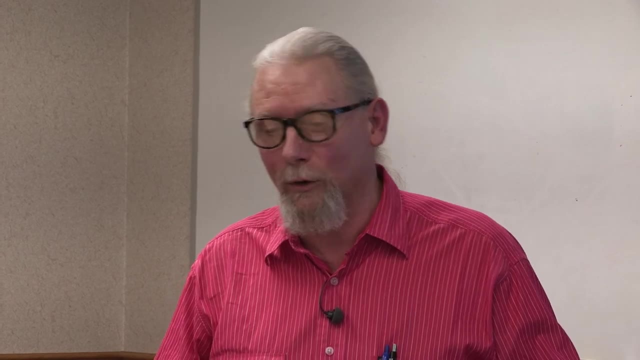 The question was: on the North Slope, do you drive piles to bedrock or gravel? I thought permafrost was really deep up there. The answer is that that is correct. The standard procedure for driving piles for bridges on the North Slope. 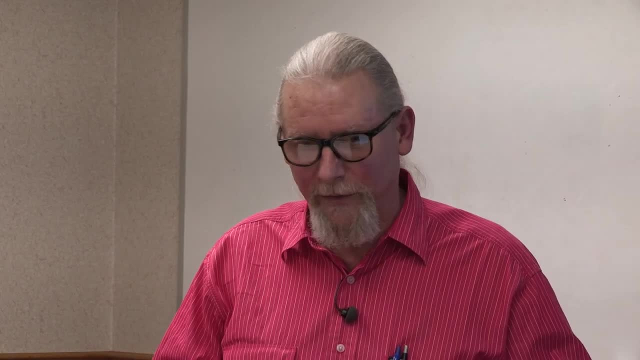 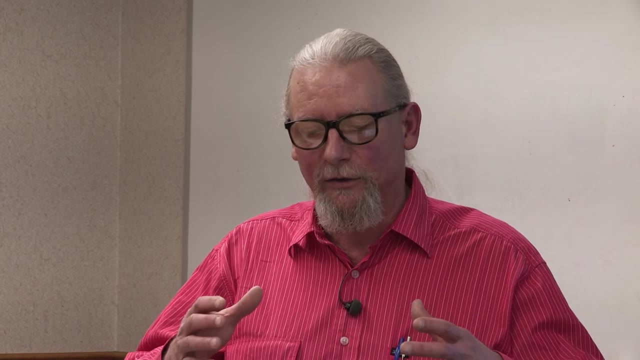 is to bore holes for the piles, place those piles and then pour a water-sand slurry around them and let them freeze back. Works really well, because the permafrost is cold enough that that sand will drain and freeze and you get the strength that you need in your piles. 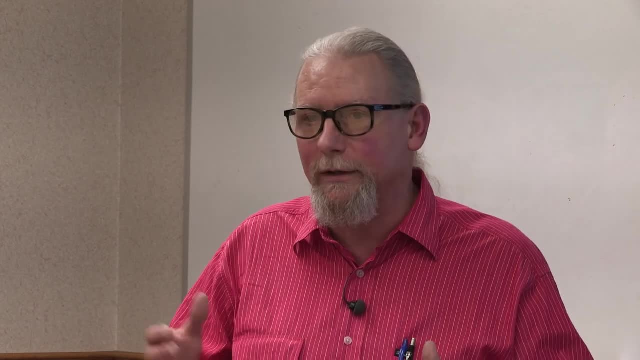 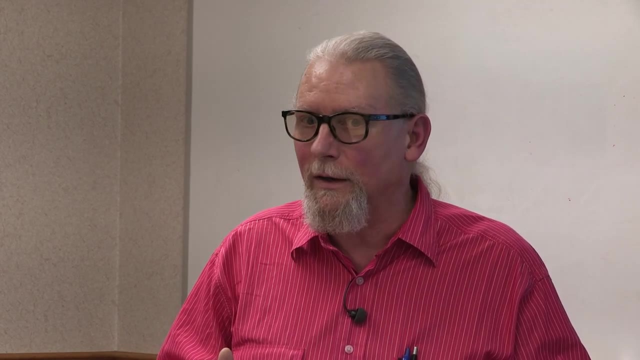 Now, someday, if the warming trends continue indefinitely, someday that permafrost is going to warm and eventually thaw, And then what's going to happen? That's all I got.